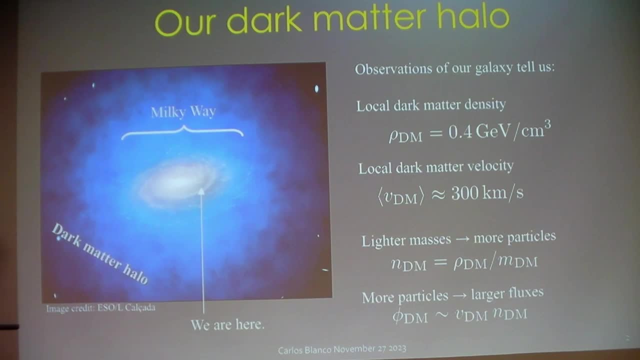 And measurement of the stars on the galactic disk. tell us something. tell us, really, just two very important things about the dark matter in our vicinity. One: it tells us the density, which is about half a proton per cubic centimeter, And it tells us about the rough mean velocity in our neighborhood, which is about 300 kilometers per second. 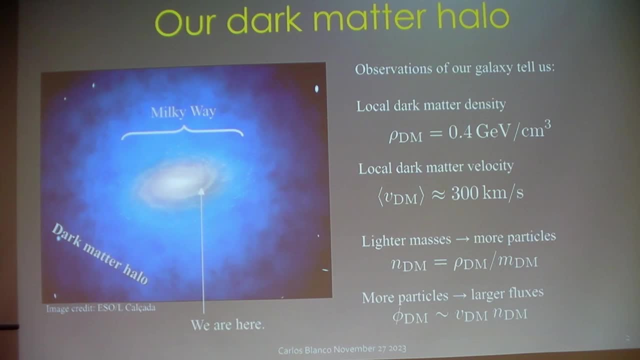 And these two things, these two constants, tell us something about how we should choose to go after dark matter. It tells us that there are two things: The number density increases as the dark matter mass decreases, And that means that if we go to lower and lower dark matter masses, we should expect to see higher and higher rates. 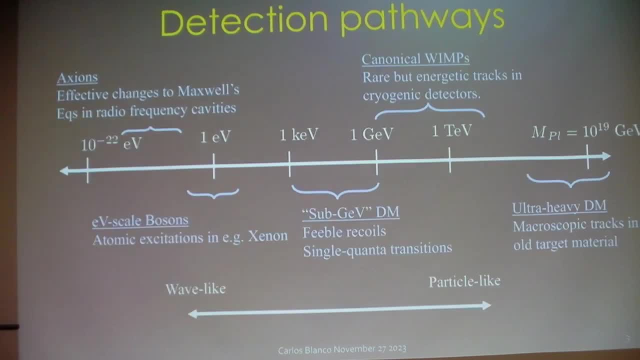 and so we can make our experiments much smaller, And, depending on what mass of dark matter you consider, the detection pathways that you might want to think about change drastically right, And so let me just point out a couple of signposts along this. 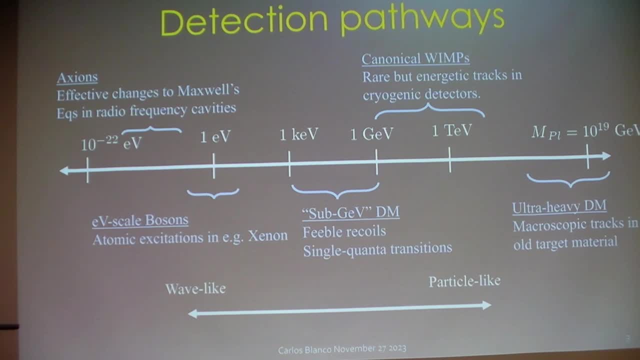 this huge spectra of dark matter masses. The biggest experimental effort so far has been put into these canonical WIMPs that are above by the GEV, and you guys have a great direct detection team here with the Conorogon and Xena. 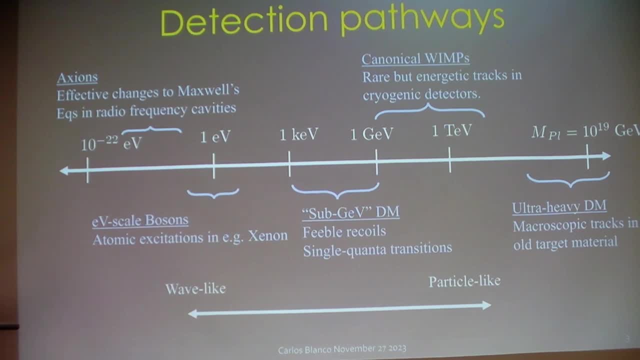 And so they focus all of their efforts into trying to detect things above a GEV. Why a GEV? Because it's the mass of the proton, And you can inject energy very efficiently into a nucleus if you're above that mass. Okay. 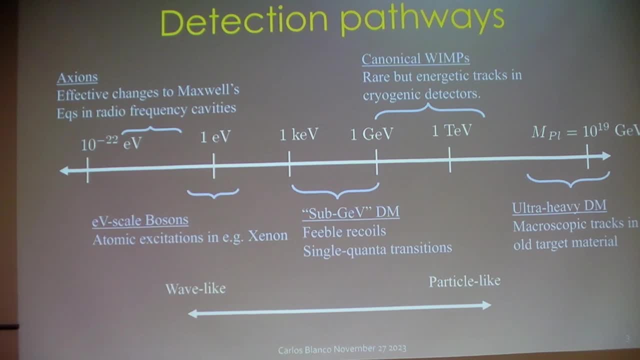 Below that mass you can still have these quasi-WIMP dark matter models, where you have some thermal history that makes sense, but down there you're no longer able to ionize an atom, And so, instead of looking for these very rare but energetic tracts in your cryogenic detectors, 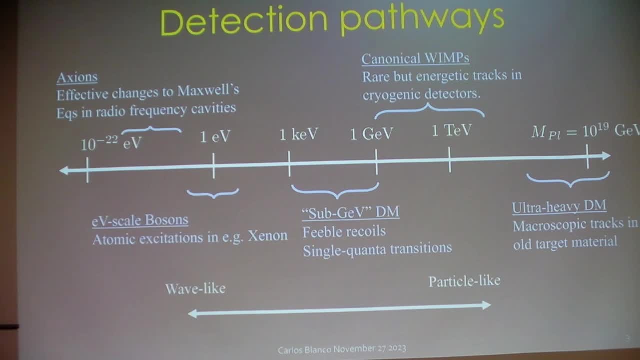 you're looking for very feeble recoils and therefore, what you're looking for are single quantum transitions, which is, in essence, very similar to what you think about in optical spectroscopy, And that's much of what I'm going to be talking about today. 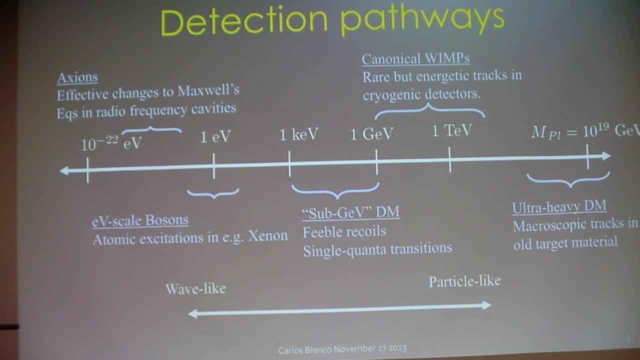 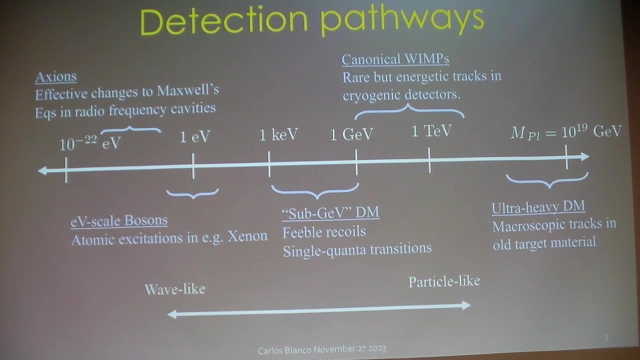 So do we know the distribution of the dark matter as function of energy, or we just don't know? We do, We do, We have a very good guess about the velocity distribution of dark matter? And what about mass? No, We don't know where the dark matter lives anywhere. 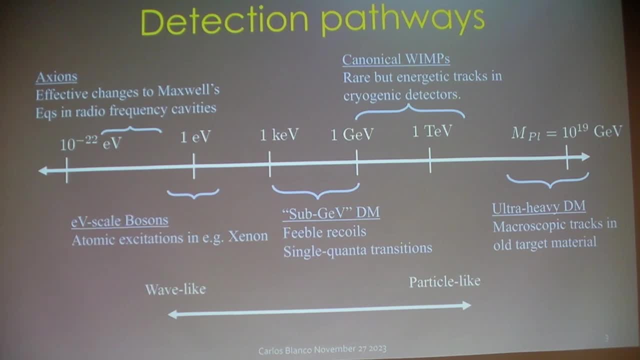 So just everybody just looks in the dark and hopefully something happens. That's right. There are strong theory priors that are placed on this parameter space that tell us that it will likely be somewhere between the sub-GEV and you know, the canonical WIMP picture. 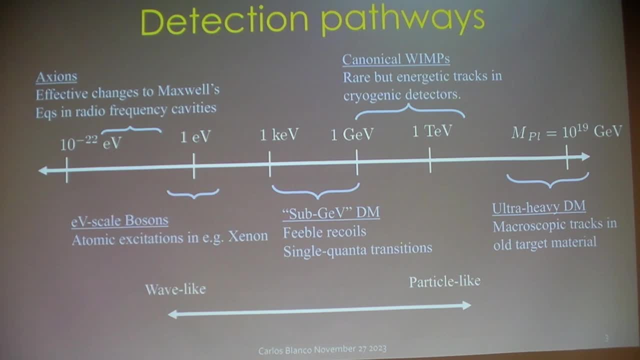 There's a lot of theories that place it there, but there's also a lot of theories that place it in this, like axion and EV scale, boson region, Right, That's why you said low energy. you know total mass per unit volume. 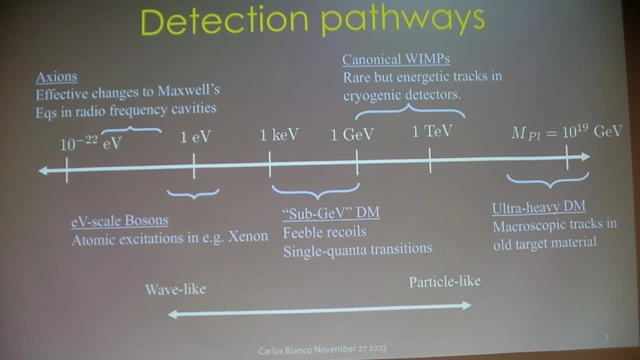 Yeah, That's why you said the lighter stuff. Exactly, You have a lot more Yeah, Number right, Yeah, Yes, sir, Can I have a question? Yeah, Is there a simple way to understand why one GEV is the magical number for ionization of an atom? 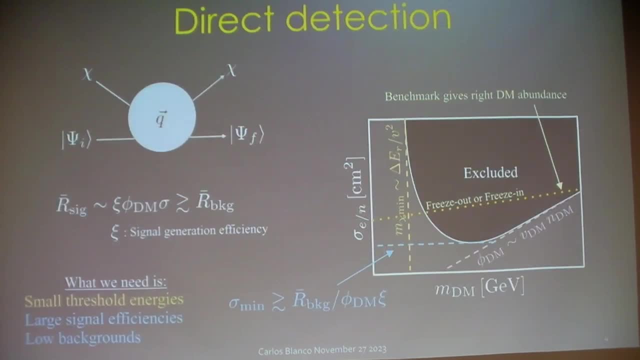 We will get there in the next slide. Okay, Great. So a lot of the plots that I'll be talking about today kind of look like this cartoon right, where you have the dark matter mass on the x-axis and then you have some coupling to the standard model. 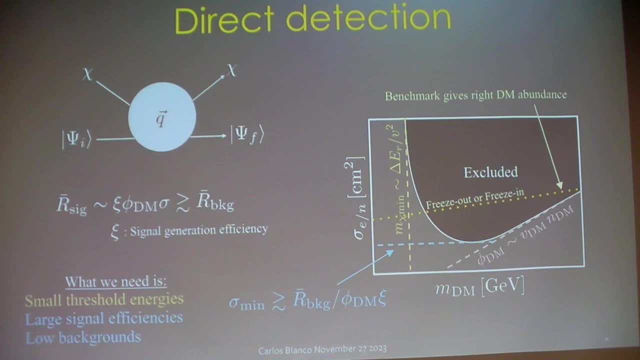 And the exclusion, the sensitivity of a particular detector setup is what would be in this black shaded region, And there's a couple of features in these plots. generally, right, There's a minimum dark matter mass that you're sensitive to and this is what you're asking about. 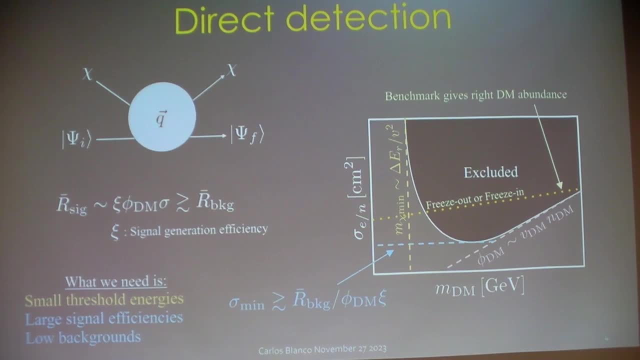 And that's really just set by the threshold energy necessary to drive a transition. So in the case of xenon, the minimum energy that you need to impart is about a keV, Right, Right, And so if you do the kinematics, that means that you need a dark matter mass of about a geV to drive a transition. 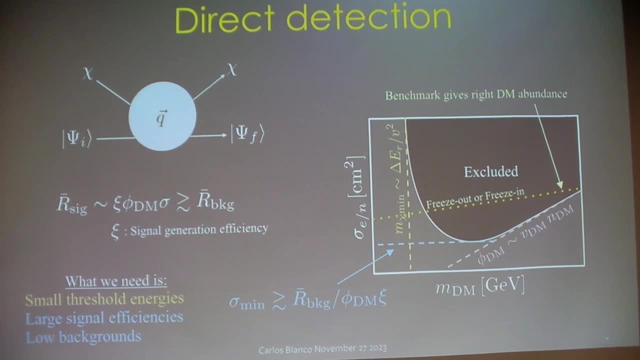 That's why that's the magical number. And so if you want to move further to the left, to light and light and light and light, you need to find systems with smaller and smaller energy transitions. Okay. Similarly, if you want to probe more feeble interactions, 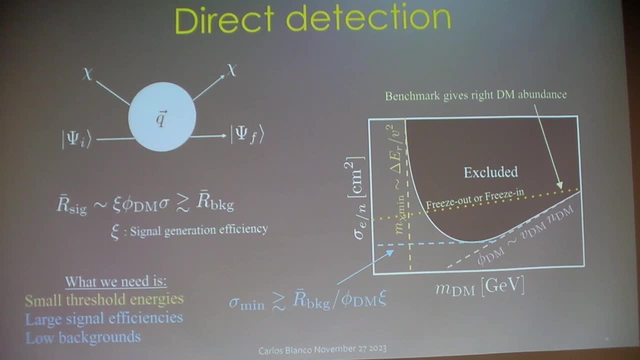 that's mostly just dependent on the rate of your backgrounds and the efficiency of your signal Right. And so if you want to get to more and more feebly interacting dark matter candidates, you need very efficient signal generation and a very sensitive detector that you can exclude backgrounds very efficiently. 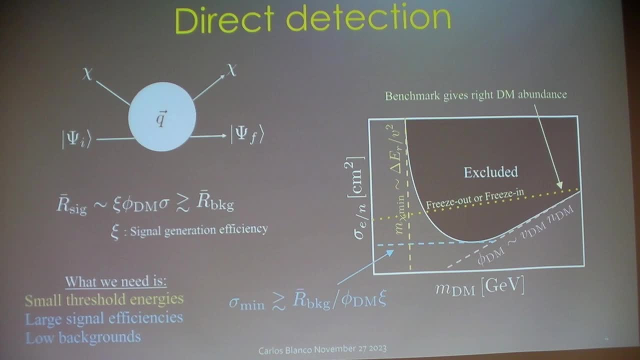 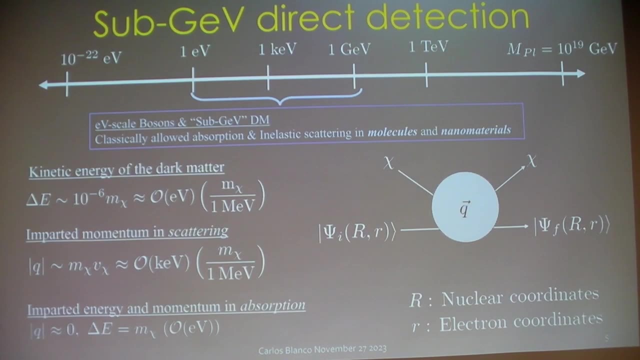 And so that's this list of things that I'll talk about: Small energy thresholds, large signal efficiencies and low backgrounds. Okay, So let me now say that I'm going to really focus on this. eV to sub-geV dark matter parameter space. 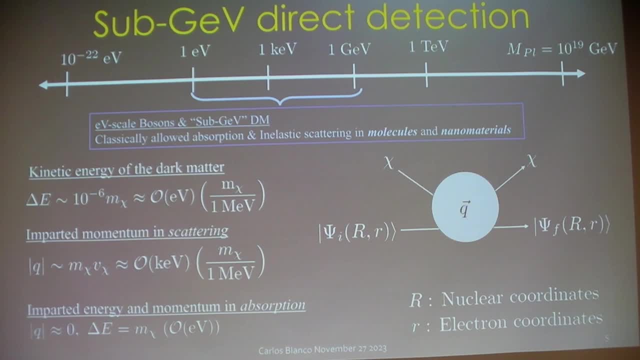 And here you have classically allowed absorption and inelastic scattering off of molecules and nanomaterials. That's really the topic of the talk. Okay, And so the schematic setup here is: you have a dark matter particle. I'm going to represent that with chi. 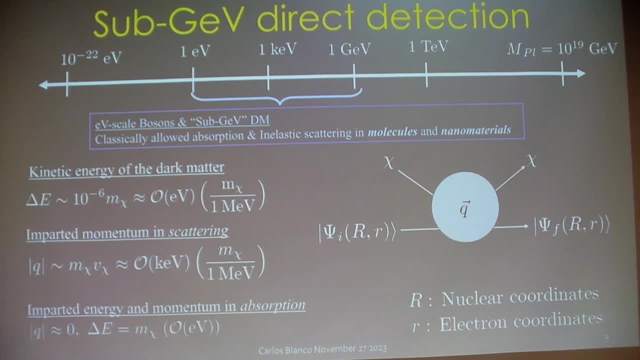 And this is not a Feynman diagram. It's just saying that you have a dark matter particle And if you have that interacting with some initial state, psi i, it's going to promote that state, some experimental state, to psi f and it's going to impart some momentum q. 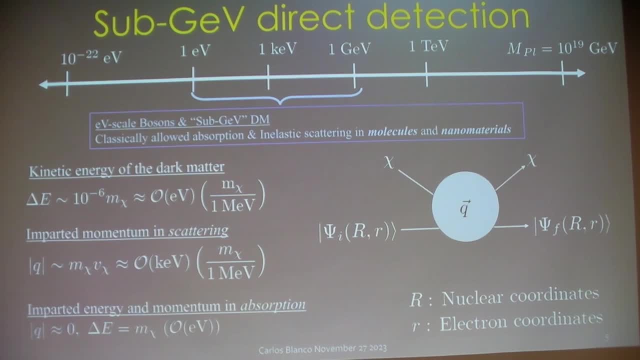 And we're totally blind to how it's going to do that. We don't really care. We want to work completely independent of a model And if you work out the kinematics, if you're looking for an eV dark matter candidate. 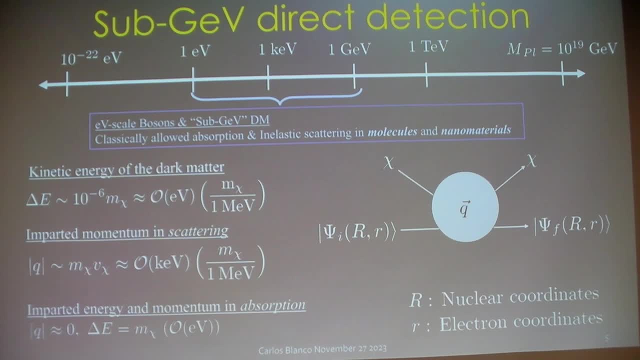 you're looking for systems that have older eV transitions, Okay, And that they will be able to accept momentum transfers on the order of k eV In the case of a bosonic absorption. you're just looking for vertical transitions of order eV. 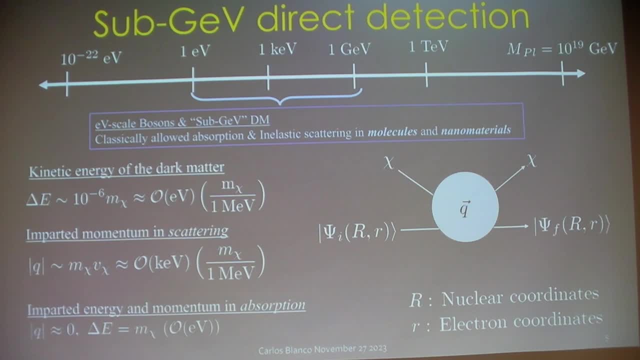 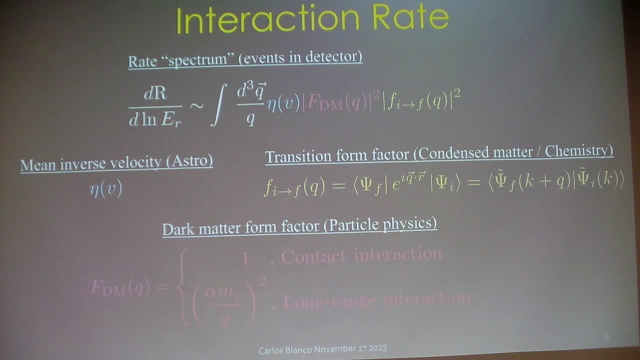 And that's why you can go all the way down to an eV if you can absorb the dark matter. Okay, The things that matter for the rate that your detector is going to give you really just fit into this rate calculation, And it doesn't matter what the details of this really are. 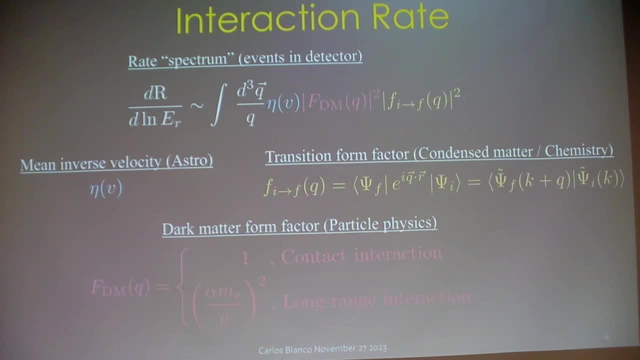 What matters is to say that the physics really factorizes into three parts: Eta, which tells you about the astrophysics of the problem, tells you about the mean inverse velocity. This is like the phase space distribution. The particle physics of the problem can be sort of factored out entirely into this thing called a dark matter form factor. 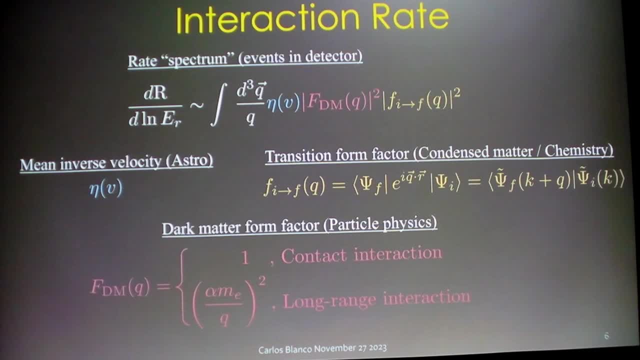 And this tells you whether or not you have like a contact interaction or a long range interaction. This is your vacuum matrix element. You guys can tell us all about that. And then, finally, the art of the problem, when it comes to bridging the gap between experiment and theory, comes in this transition form factor. 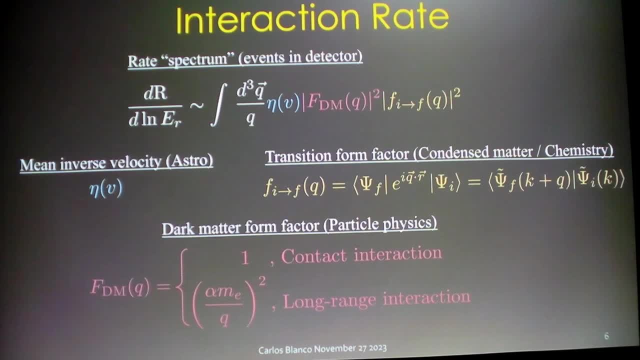 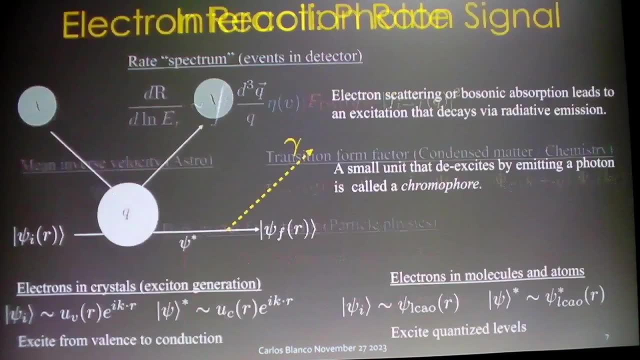 And that is informed a lot by the condensed matter and the chemistry And that tells you what the probability is of absorbing momentum q and doing this transition. Okay, So now let's start with the easiest possible thing that you can go after, which is looking for dark matter using some electronic data. 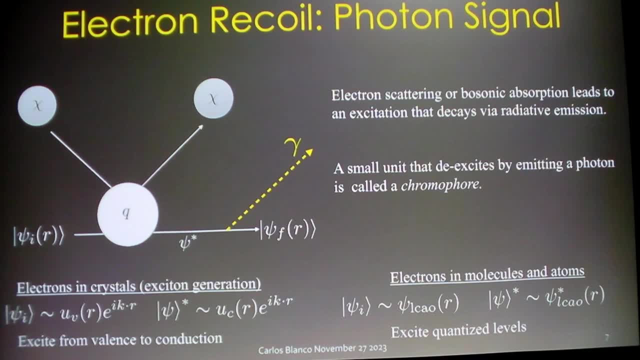 Okay, Okay, Okay. So let's start with the electronic transition. So here your dark matter is going to recoil off an electron, It's going to drive a transition And you're going to look for the de-excitation, And one de-excitation signal that you might look for is a photon. 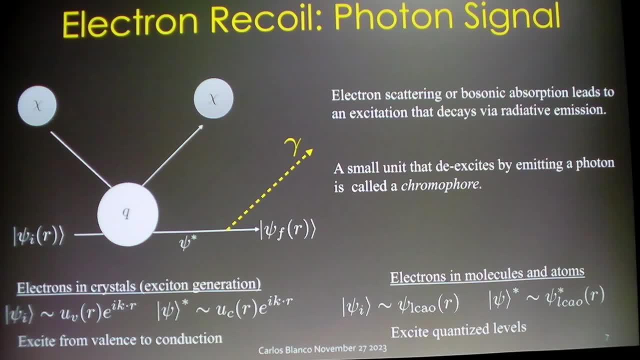 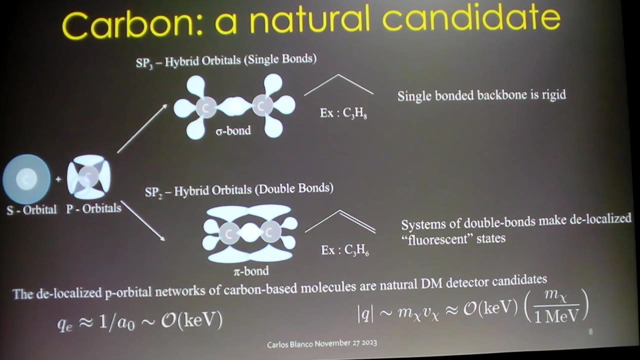 And there what you're trying to really look at, the kinds of systems that you're looking for, are called chromophores. They're small fundamental units that de-excite biomegantic photons, And so now let me tell you how we can think about chromophores in the future. 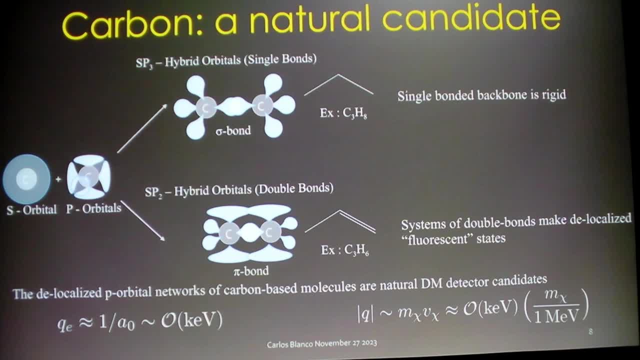 And we're going to talk about chromophores in the sense of molecules. Okay, So carbon should be everybody's favorite atom. That's a fact, And that's because it makes up everything around you. Hydrogen- Hydrogen is my favorite atom. 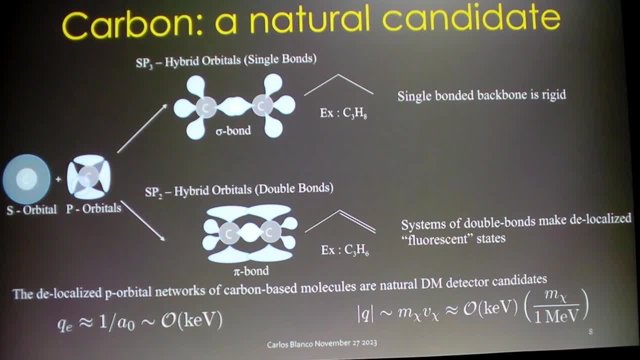 So I disagree, I disagree. So the electrons and carbon can hybridize into these sp2 and sp3 orbitals, And of importance is this sp2 hybridization. You have carbon atoms that are bonded first longitudinally in. you know this single bond. 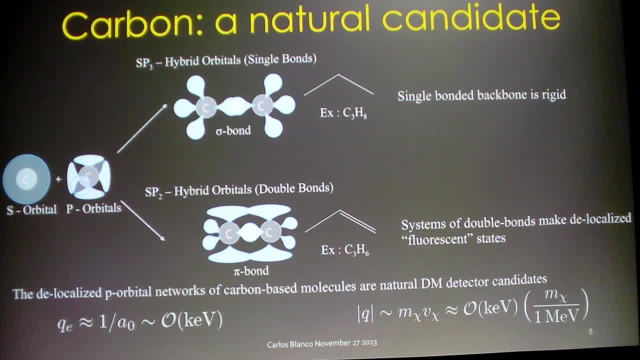 But importantly they form a preferential plane, symmetry plane, And above and below that plane you have these pi bonds, And these are very de-localized orbitals where the electrons are free to drive transitions that the molecule doesn't really know about. The backbone of the molecule stays largely unchanged, while the electrons in the pi bond are free to sort of roam around. 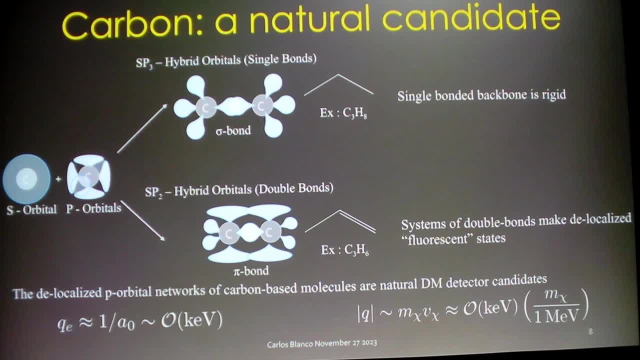 And if you sort of just close your eyes and you ask: well, should you expect that systems made of carbon are well matched to absorb the momentum of the dark matter? at about an eV? It turns out yes, Because the momentum transfer is of order of KeV, which is just one over the Bohr radius. 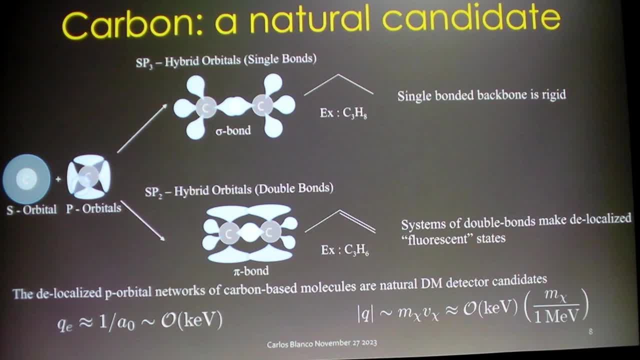 Right, And so that is the characteristic momentum that these electrons are flying around, with Transfer from where to where. Sorry, This transfer is from which state To which state? From some pi orbital to another pi orbital. Oh, okay, Okay. 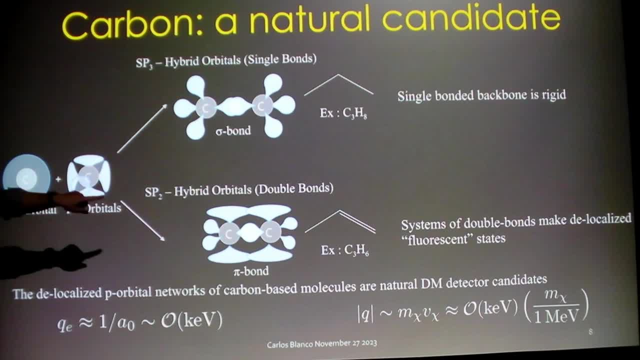 And you'll see these pi orbitals being signified as these double bonds. So are you sorry? are you so? are you thinking about? you said that this factorizes, but I mean, don't you need to know, like in this case? here I would want to know like are you imagining that the dark matter has a direct coupling to electrons? 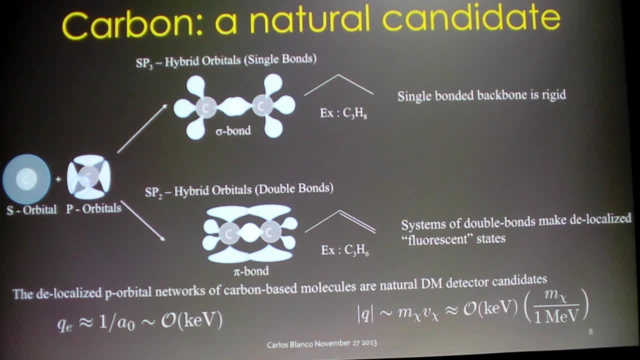 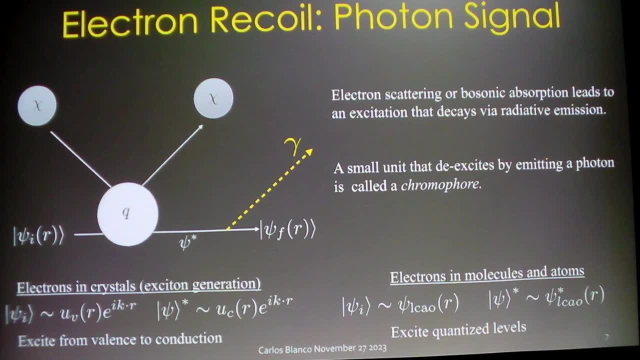 That's right. Yeah, So you are assuming that? Yeah, So So here I'm assuming electron coupling, electron coupling alone. The type of electron coupling I'm allowed to free float, whether or not it's momentum dependent, whether it's spin dependent. 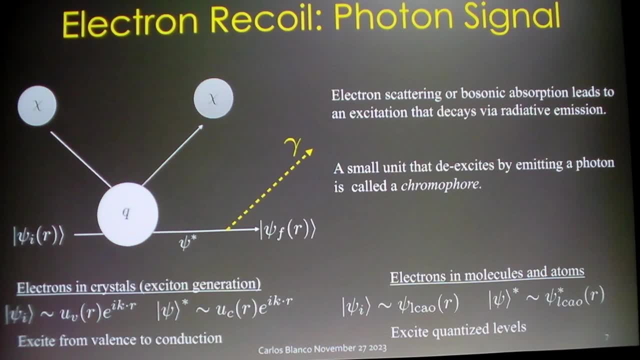 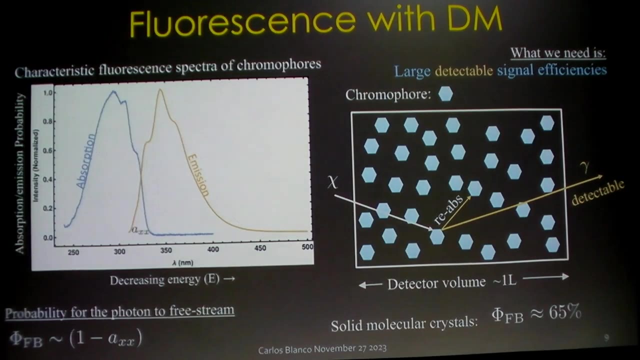 It doesn't matter. For each choice you would have a different matrix element to compute Exactly In pi. orbital, Yeah. Yeah, We kind of bracket the options between, you know, contact interaction and long range interaction, Okay, And so the kinds of experiments we're really thinking about. 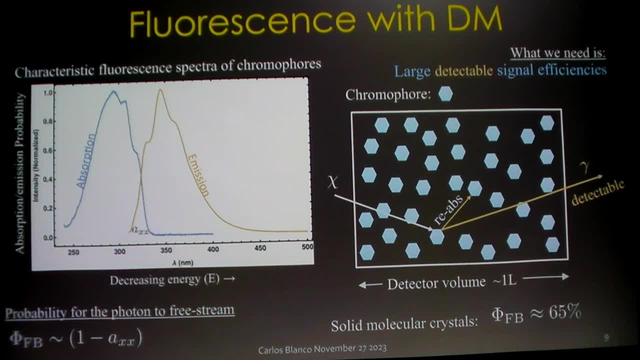 One of the experiments we're really thinking about is a system where you have carbon making up small subunits, chromophores, and you're sticking them all in a vat. The vats can be, you know, as big as a liter. 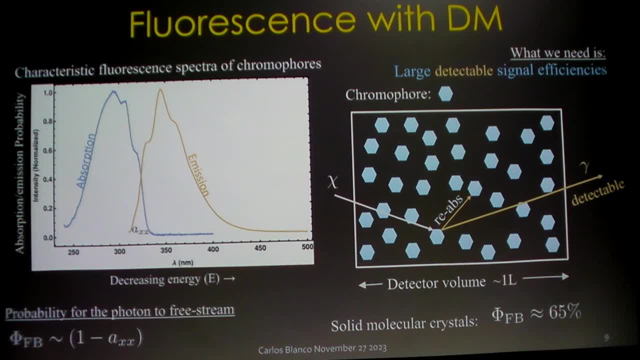 The dark matter comes in, it excites a chromophore, then emits a photon, And you're trying to detect that photon. The first problem that you think about is like: well you know, if you're really just driving excitations, won't the photon just get absorbed? 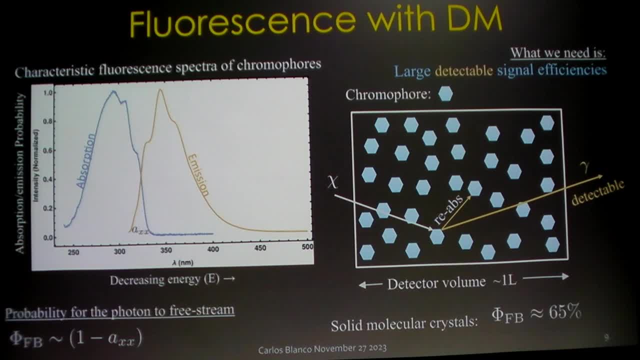 And here nature has been really quite kind to us, And it turns out that most molecular chromophores have a stoke shift with relation, the absorption and the emission characteristic. So this is like the band where you can absorb energy and the band where you emit energy. 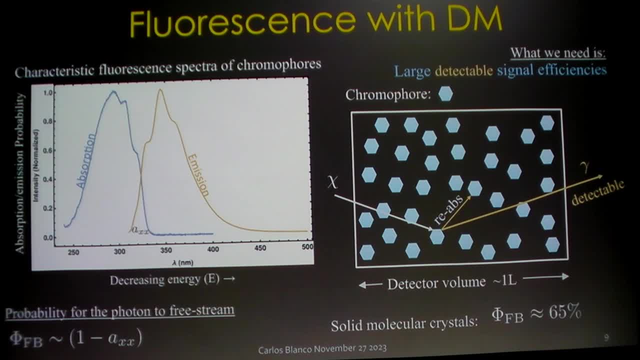 Which means that the photon emitted from one molecule is likely to just free stream And that free streaming probability is just proportional to the to one minus that overlap. So here you know, like this is kind of optimal, You get for free. 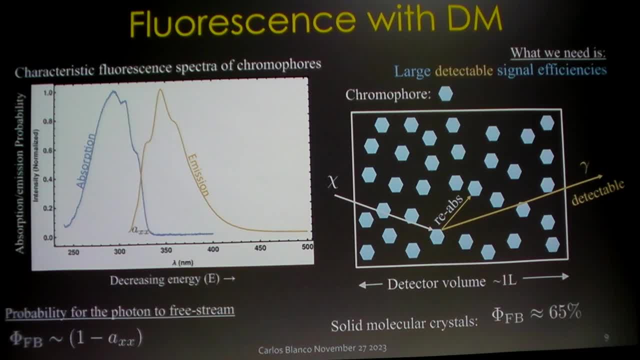 And the kind of free stream probabilities that we can look at are, you know, almost unity. Like 65% of all photons created will be able to leave the material. So what is? it looks like the kind of traverse approximation that just shifted between absorption and emission. 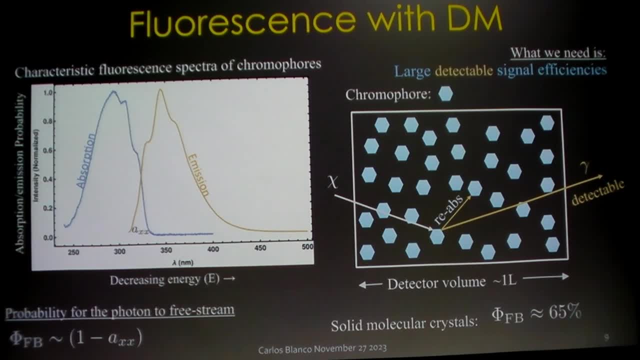 So what's responsible for that? Good, So what occurs is, if you think about the selection rules of driving electronic transitions, is, if you absorb energy, you also have to excite the molecule, And so what you're really doing is you're driving an electronic transition plus a little bit of a rotavirational excitation. 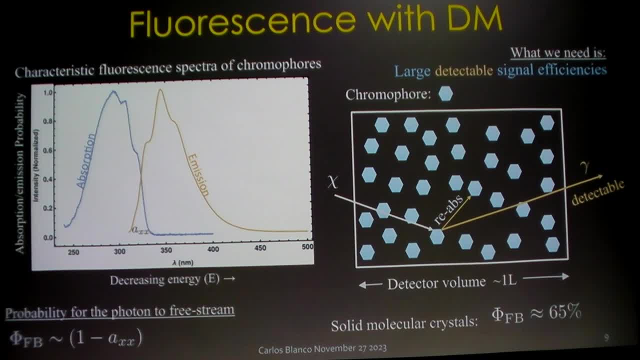 Right. And then that rotavirational excitation has a lifetime, that's like minimal, That totally de-excites immediately, And then when you de-excite the electronic state, you're now working with a much smaller energy And that you know the effect of lost vibrational relaxation is this stoke? 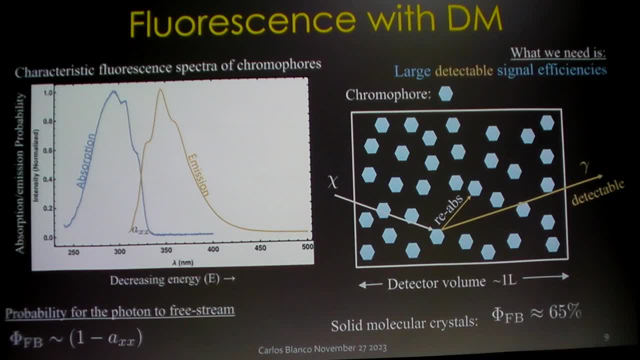 You're saying you lose. you sort of lose the energy quickly and then you emit the rest of it in momentum, And that's so. then you're emitting less momentum than you absorb. Yeah, Okay, That's right, Got it Thanks. 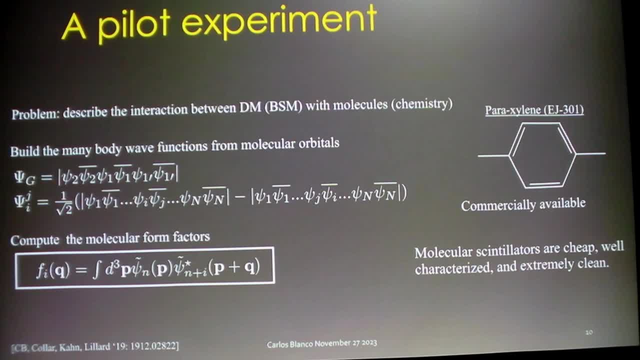 Okay, So three years ago we had a pilot experiment in Chicago where we looked at this molecule, parazylene, which is a commercially available scintillator, And a colleague of ours, one of my colleagues at the University of Chicago, knocked on my door and said: 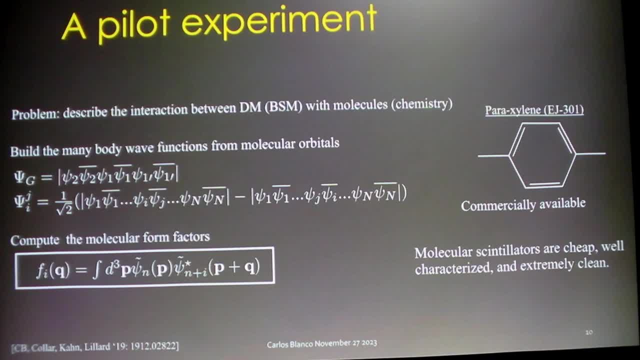 look. we got to determine what kind of dark matter we can go after, how dark matter is going to interact with these simple molecules, And so we got to work writing down what like the molecular orbitals look like, what their states do, and how you can absorb momentum through these things. 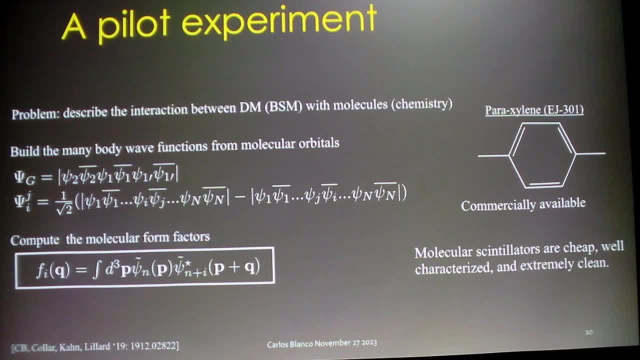 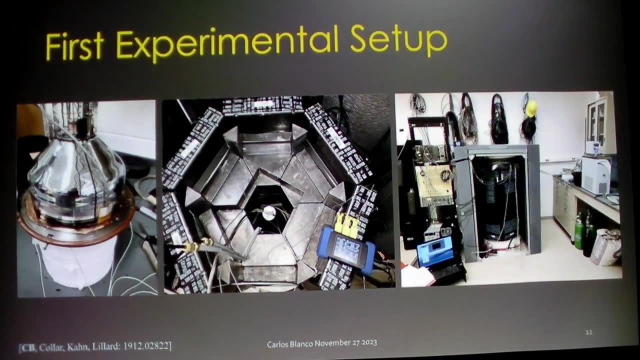 And we found out that it's actually a pretty straightforward calculation, And so we went from theory to actually experimentally deploying this thing. It was quite easy, So this is a picture of the experiment. This is about a paint can's worth of this xylene. 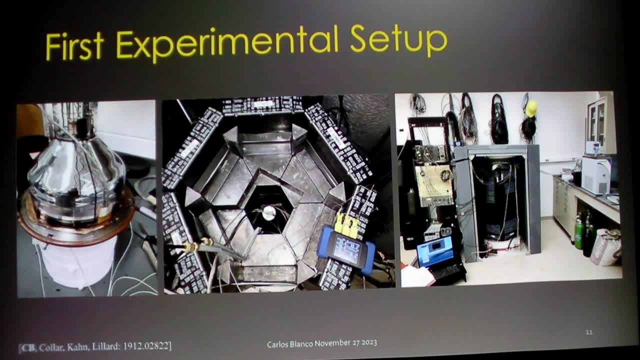 And on top of it is a PMT. It's a very sensitive Hohematsu PMT. You stick that in a very shielded vat with you know your muon vitas all around, You know this is ancient lead in the basement of a physics building in Chicago. 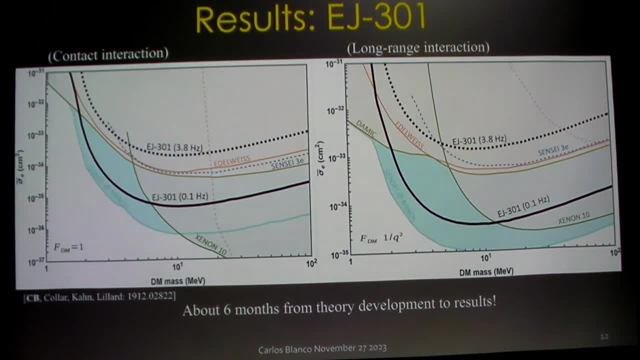 And you take data And after about six months we had honest-to-goodness results. And so these are the sensitivities for what was the bleeding edge at the time of silicon and xenon. And then our experiment is this dotted line Right. 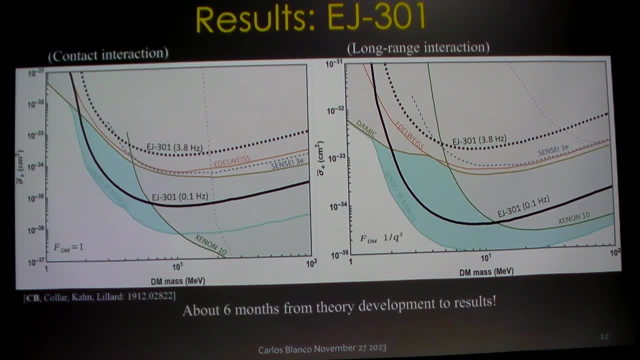 And this 3.8 hertz. what that corresponds to is: that is the limiting factor that comes from what the PMT was seeing in its blinded mode. Now, this PMT was characterized to go much smaller than that, So we expect that to be mostly driven by cosmic radiation. 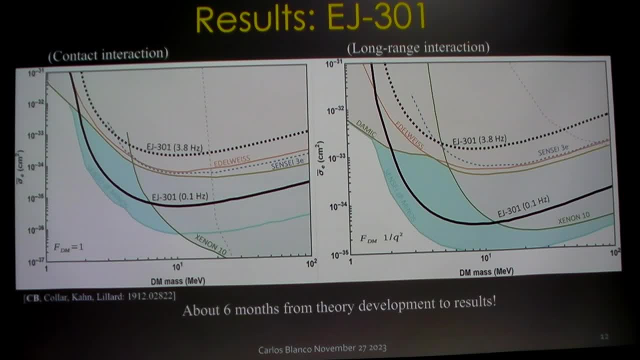 And so we tried to predict what that rate would be if we'd be able to go to a deep underground location at Hermula, And we would have the black line if that was the case. And really this is all just to say that fluorescence, with these things, works. 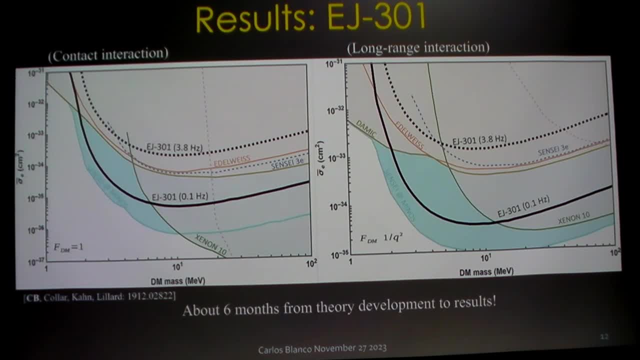 And it's a very cheap, very fast way of probing parameter space. I mean, we were within striking range of Sensei And we were able to do it with what's essentially garage level physics And so great. So roughly sorry, you probably said it. 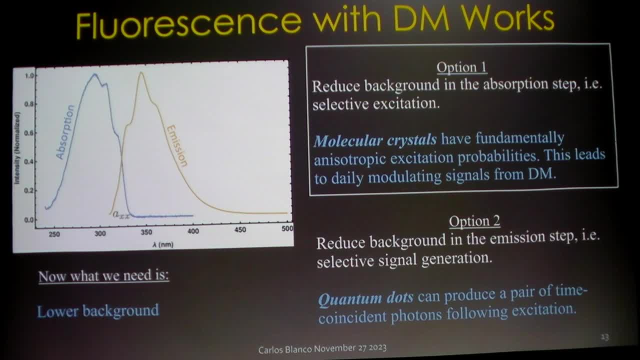 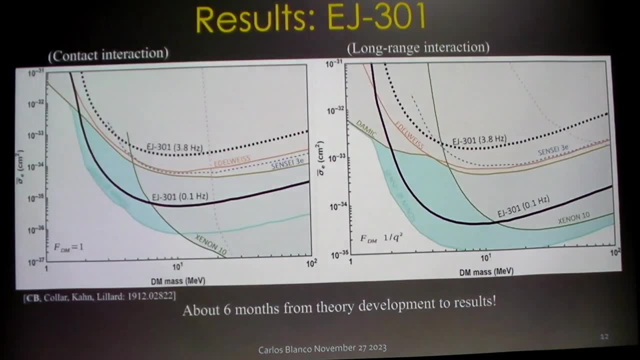 But, roughly, what is the photon, I guess? what do I want to know? I guess I want to know the frequency of the emitted photons. There are single photons emitted in these things- Yeah, There's you're looking for, And what are? so what's the frequency? 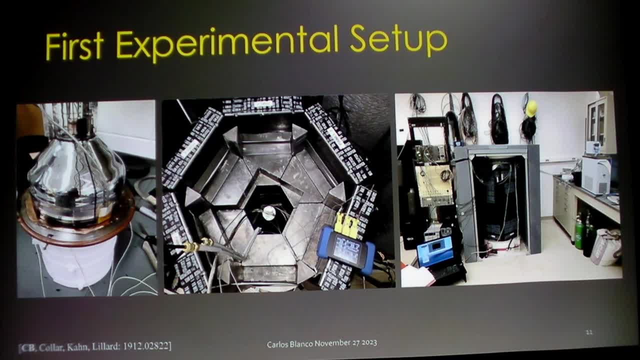 I don't know about the frequency, but there are about five UV photons. Okay, It's UV photons. Yeah, This is UV photons. This is why we can use a bioalkali PMT. Yeah, Okay, Great. So my question is: you don't know how the electrons interact with the dark matter you're trying to detect? 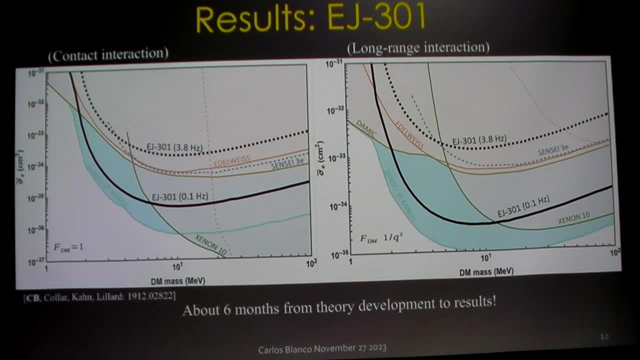 How do you set the detection limit Right? So that's why You can have a plot. but Yeah, Because if the cross-section is, the vanishing is small, Right, You're not seeing anything. So that's why this is a function of cross-section. 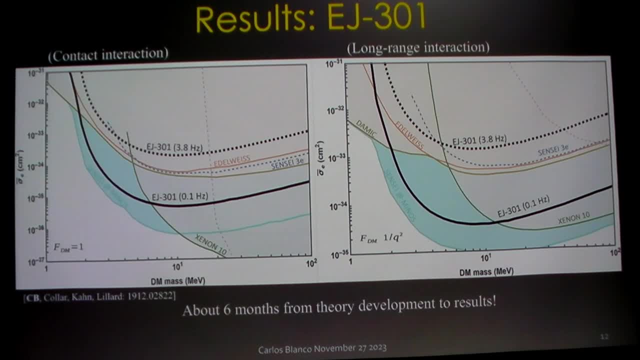 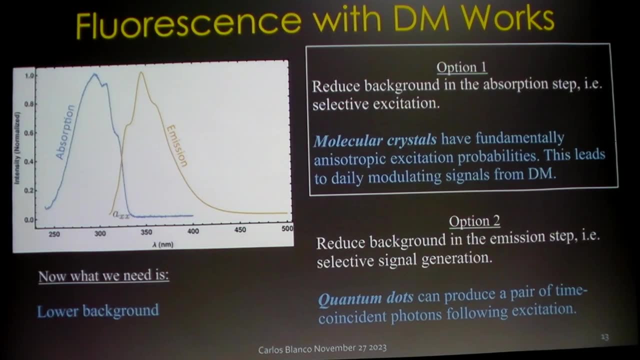 We can rule out cross-sections that are above a set amount. Oh, this is okay, Yeah, Okay. So we proved that you know, these fluorescence experiments work and they're very effective. So how do you do better than that? 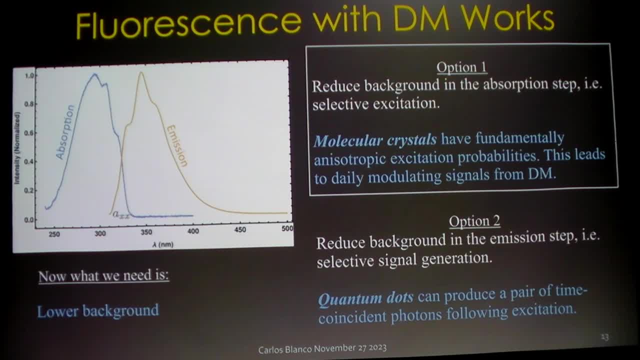 Well, I'll tell you about two options, And the first option is to go after this lower background, And you can do that one of two ways. The first one is to reduce the background in the absorption step. In other words, if you focus on how you're exciting these molecules, you can get some really strong improvements. 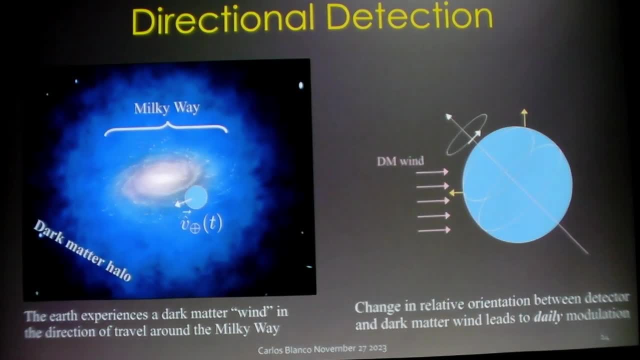 And so first I need to tell you about how I lied in my experiment. I lied in my first slide. I kind of cheated you because I told you that we were in the middle of the galaxy. We're of course not. We're somewhere off center and the galaxy is rotating with respect to the dark matter, halo. 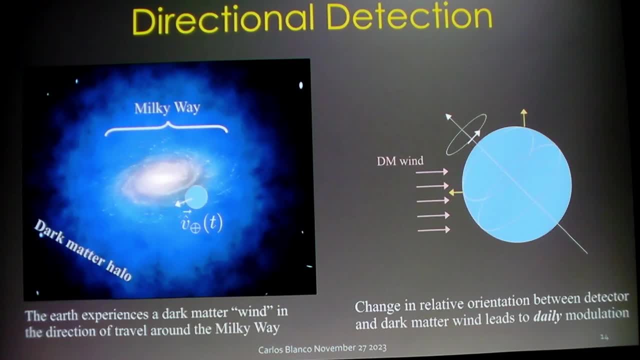 And this induces an effect of dark matter wind. And due to the rotation of the earth that's on an axis, this wind can be thought of as coming at some point in the day from the wall and at some point in the day from the ceiling. 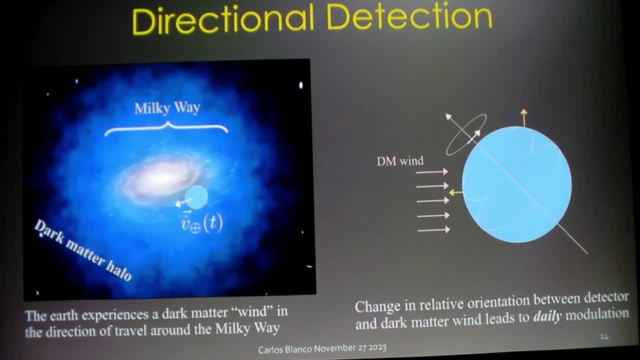 When you're, you know, at a latitude of something like Chicago. And what does that mean? It means that if you have a dark matter detector that can tell the difference between momentum being injected in the direction of your walls and your ceilings, then you can have an excitation probability that is way different than just random thermal noise. 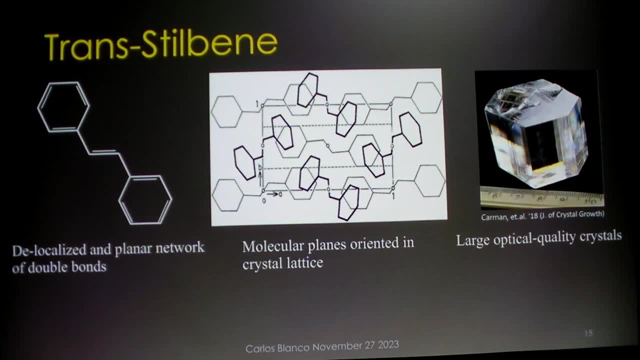 And so we went out and we tried to look for chromophores that could tell this difference, And we came up with this simple example. It's called transsylvanium. It's very similar to xylene, It's just these two fennel rings bridged by an ethylene oxide. 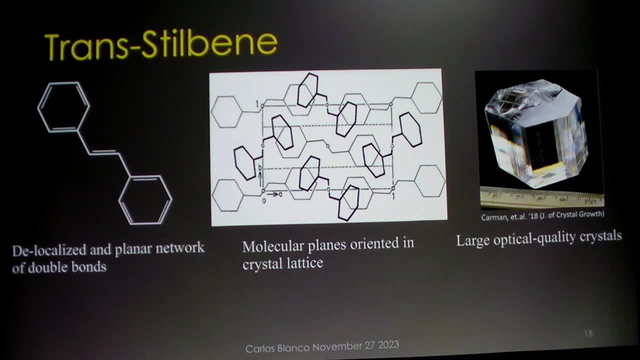 And they like to stack in these crystals, basically that they look face on all towards the same direction And they can form these macroscopic single optical quality crystals. They're, you know, very inexpensive. Can I go back a little bit? Can you maybe just say a little more? just in the first kind of setup that you described, 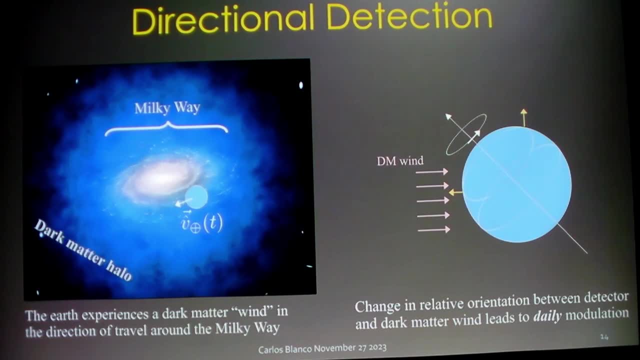 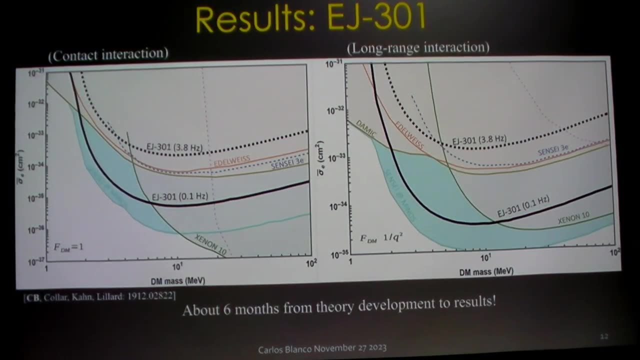 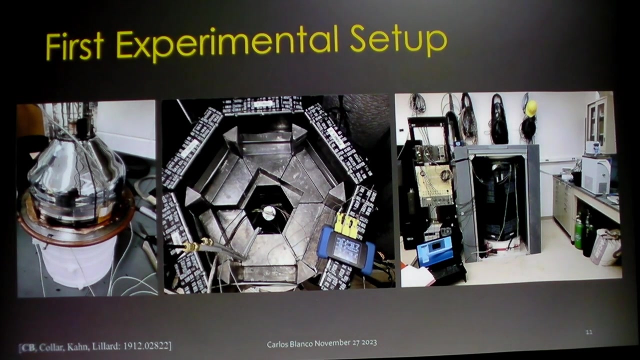 Sure, Like, what are the limiting factors? Is it just background? That's right, That's right. So it's just like low frequency, well, just like photons, or Yeah. So it's. you count the clicks coming off of this PMT. 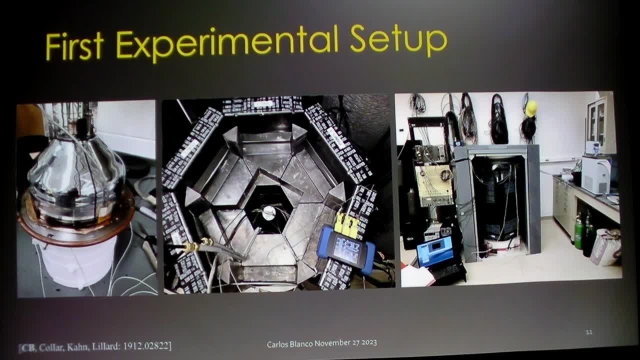 Yeah, And you say: what's the dark matter? interaction have to be to give you a signal that is higher than what I pick up as the dark rate of my PMT. That dark rate of the PMT was measured here, but it's calibrated at, you know, deep underground locations to be here. 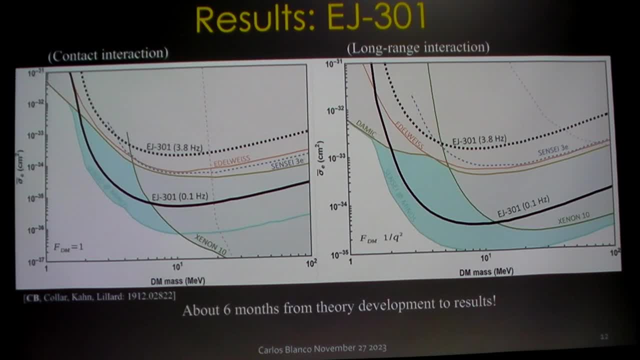 So that would be the ultimate sensitivity. Can you do better than that? Can you beat the dark rate of a photodetector? Yes, So is that the dark line then? Is that essentially zero background, Or is there some? if you could reduce the background to literally zero, would there still be some other thing, like I don't know, like just electronics noise, or in the PMT or something? 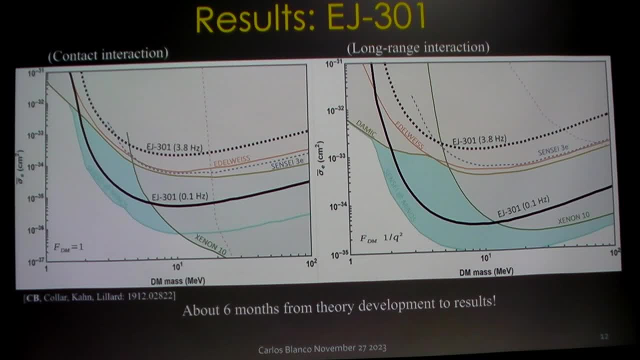 I mean, what would be? Yeah, Is that pretty close to the zero background limit? the dark line? No, No, no, no. The zero background limit is many words of magnitude below this limit, Because this is a very dirty experiment what I'm showing here. 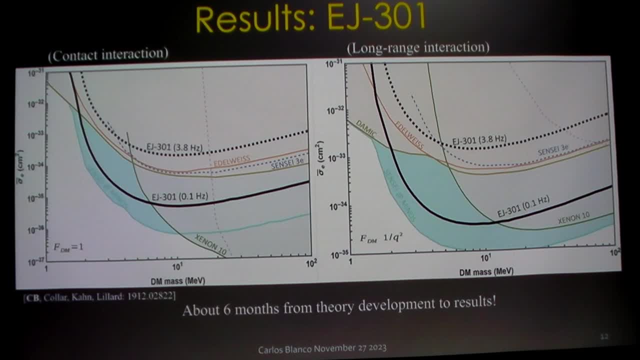 This is the background, coming from a PMT that's really calibrated to do physics at ionization energies, not at fluorescence energies, And so if you were to be able to dip this background way further down with the lowest noise photodetector, which turns out to be Sensei, 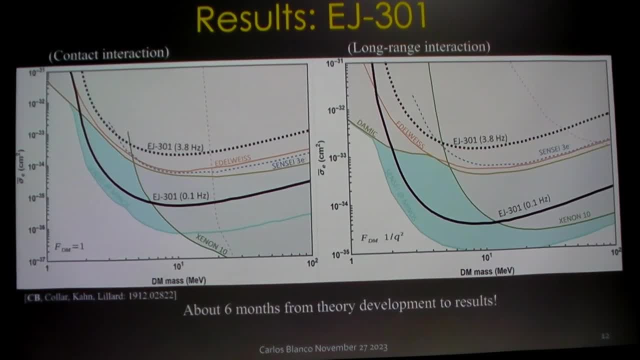 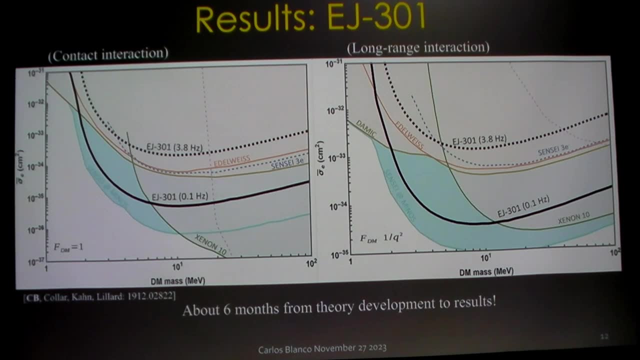 Sensei, is a photodetector that's essentially background free. So you go lower and lower And then your main source of background is essentially the thermal self-activation noise and the very, very tail end of beta decay of carbon, And I experimented with it. 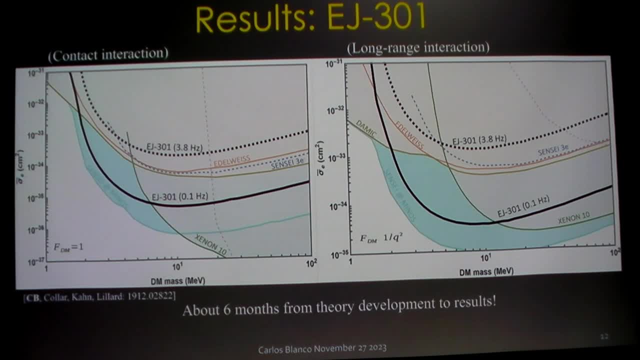 So you can, in principle, cool the detector? That's right To control thermal part of it, Yeah, But now this background is mainly from actual events that strike the cathodes or you know some other particles, you know just striking the cathode. 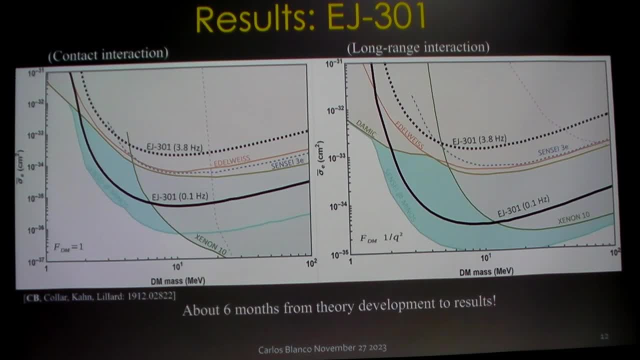 There's nothing you can do about it. You can't shield them, They just simply come to the detector. They're rare, but they're there. That's right, Or thermal? It's not thermal, I guess, right Yeah? 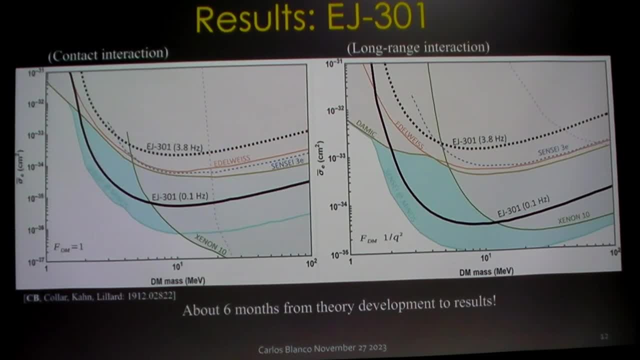 So this background ray up here, we think is coming from things hitting the cathode- Real deal, Real particles hitting the cathode, right, Real particles hitting the cathode that weren't vetoed by the panels. So cooling is because they look exactly the same as your events, right? 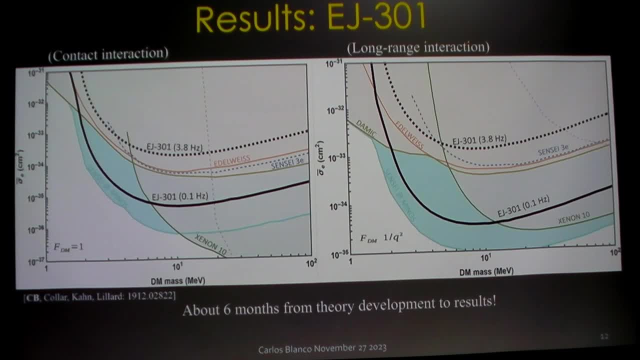 Yeah, And nothing to do with temperature. That's right. That's right. So this is what the background is known to be. if you can totally shield the astrophysics of the problem, If you can get rid of all the cosmic rays, 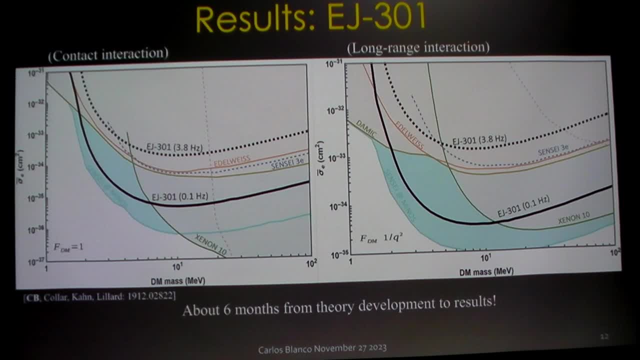 That's the limit of, that's the dark ray limit of a bioalkali PMT, And you're not doing that in the bottom line. yeah, That's right, That's what I so I think that's what I sort of meant by background free. 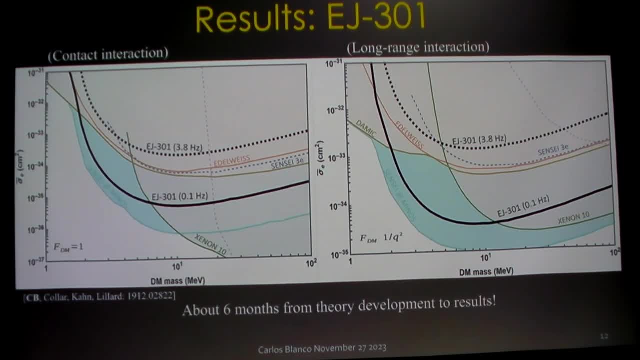 I mean, you've got the PMT that you have. You don't get to turn off that background. But you're putting it into a background: free environment. I see You're saying that's what essentially what that dark line is. Yeah, 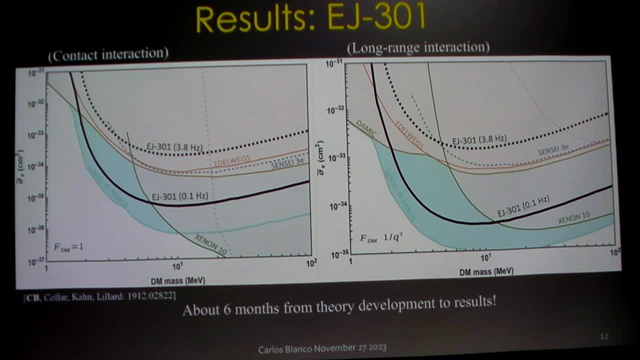 With this experimental setup, the best you could do is the black line. Oh, I, I, okay, I got it, I got it Okay. So the reason I was asking is because you know what I was sort of expecting to hear. is that okay? so we made this paint can with, the thing you know, duct tape on top, the photomultiplier tube- duct tape on top. 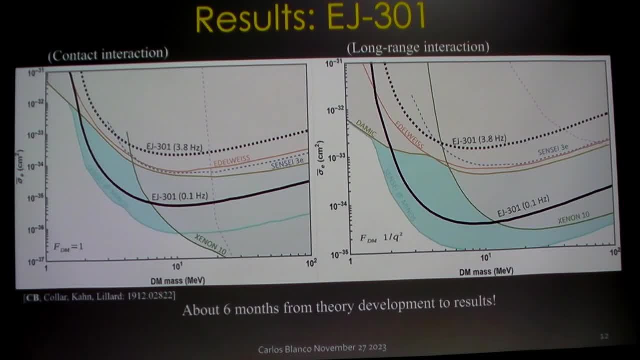 But now we're going to make one that's bigger And it's going to go in deep underground. You're just going to like: make it better, make it bigger, whatever. But you're not talking about that. You're saying: okay, we're going into direct detection. 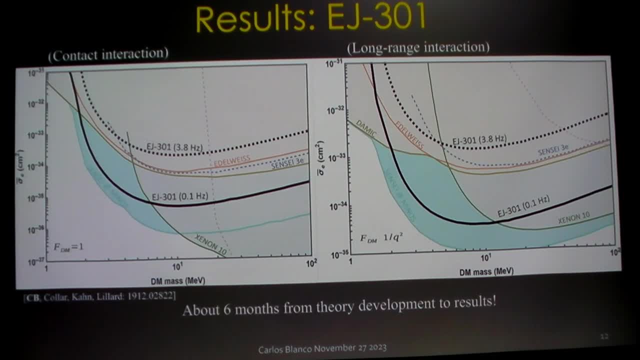 Yeah. And why is that? Is it because you can't compete with Sensei, or No? So we're going in a different direction, because there are smarter ways to gain sensitivity than just making your back bigger and trying to look for lower rate PMTs. 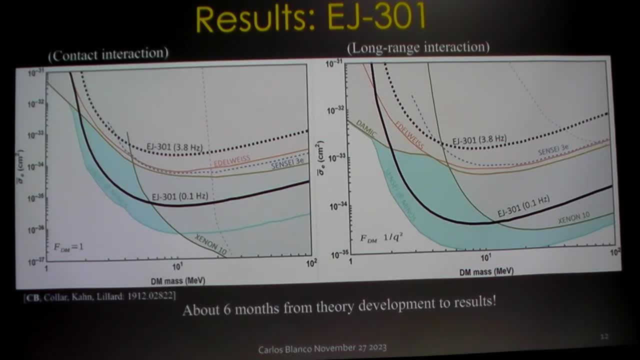 Right. So Trying to find more and more sensitive PMTs forces you into instrumenting smaller and smaller areas, And then it becomes totally prohibitive to instrument. you know a ton scale detector, So that's a non-starter Okay. 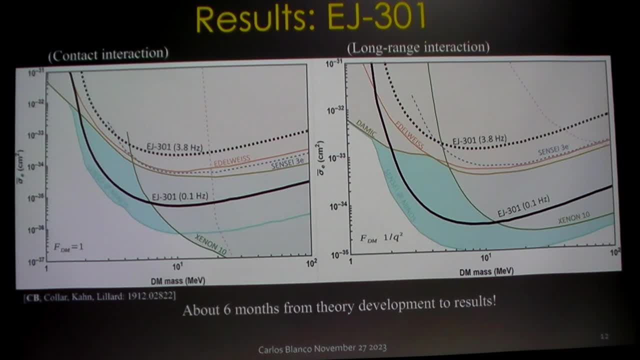 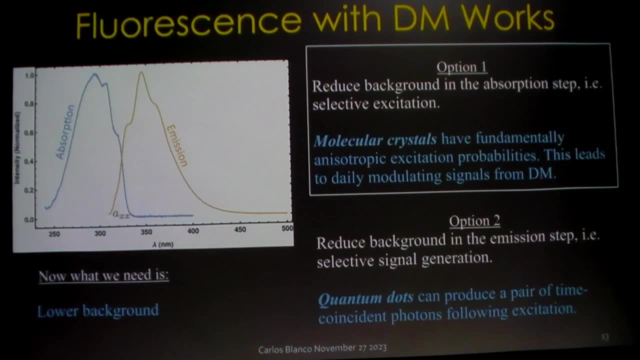 So you want to get a little bit more clever, And that's why you want to reduce the background rather than reducing it in the fundamental noise rate, lowering it in the way that the signal comes out. Okay, And that's why we're looking at the daily modulation. 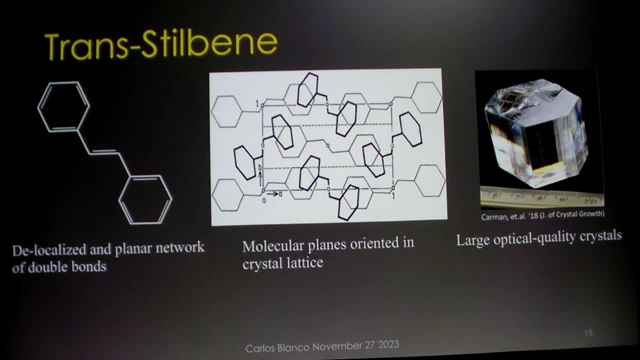 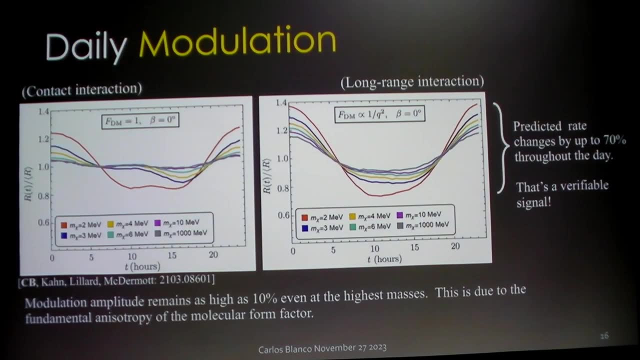 And if you look at the rate probability- yeah, at the expected rate as a function of time, looking for this daily modulation, you get curves that look like this: And so here every curve corresponds to a different dark matter mass. possible dark matter mass throughout the day. for a crystal that's the same size as the paint can. 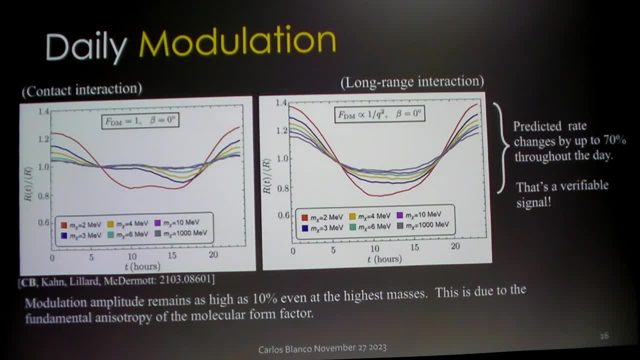 And throughout the day, you see that the signal, The signal that you're looking for, really varies by quite a lot- up to 70%- And that's a very verifiable signal That looks a lot different than just a constant dark rate. 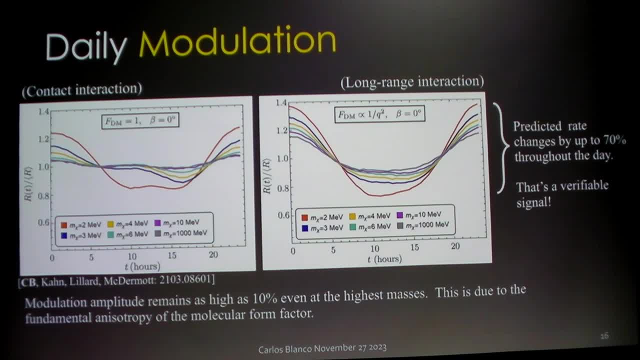 And that allows you to, you know, get rid of a lot of background. So this is the overall rate. This is not some directional thing. This is the overall rate, Right? So this crystal will absorb preferentially in one direction, but emit isotropic. 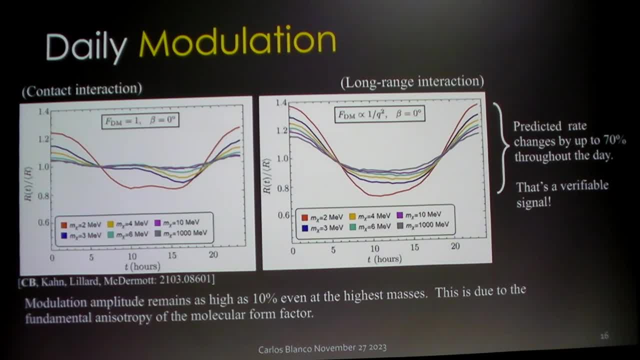 Okay, But it is. So it is a directional effect. Yes, It's not a preferred direction, That's right, Okay, That's right, Okay. So we know that the dark matter has some amount of just like velocity that, like we think, is like thermal. 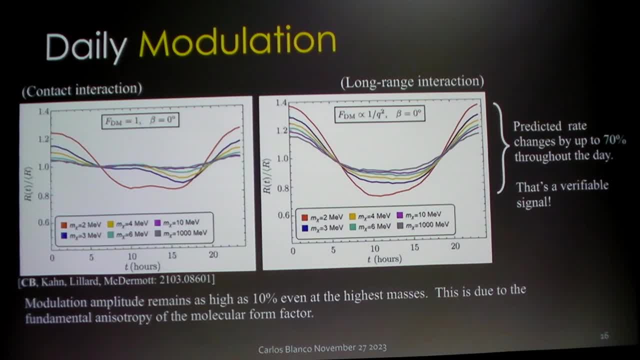 So, as we're flowing through it, how are we sure that our, I guess, like, how does our speed moving through the galaxy compare to the speed of the random motions of the dark matter? Good, So it turns out that, like the way that we build the standard halo model, as it's called, is you just think of you know? 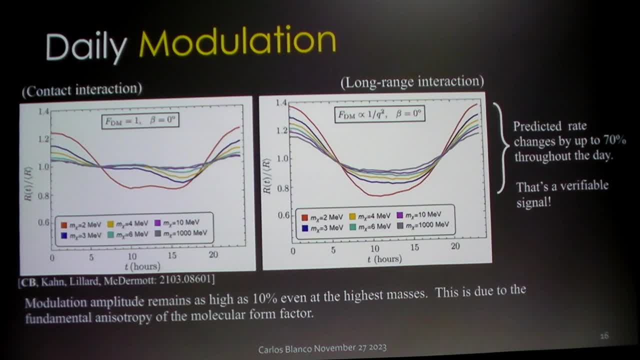 maximum volts in the distribution of dark matter velocities in the rest frame of the galaxy And then you boost, you do a gallium transformation into the rotational frame of your solar system And the mean velocity of the dark matter sort of in its own rest frame is, you know, about 50 to 100 kilometers per second. 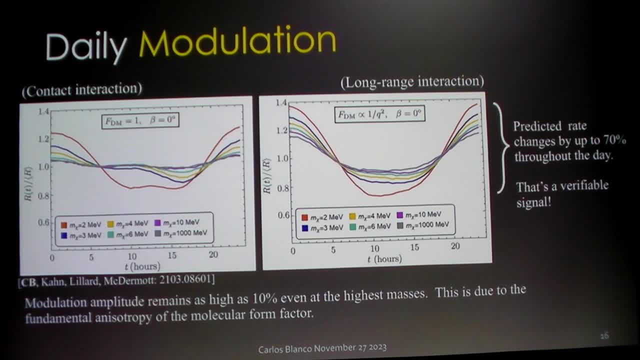 And you're rotating around the galaxy at like 60 kilometers per second. So you know it's an order of one effect. You still get things coming from all directions, So your right never drops to zero, Got it? But you do vary it throughout the day. 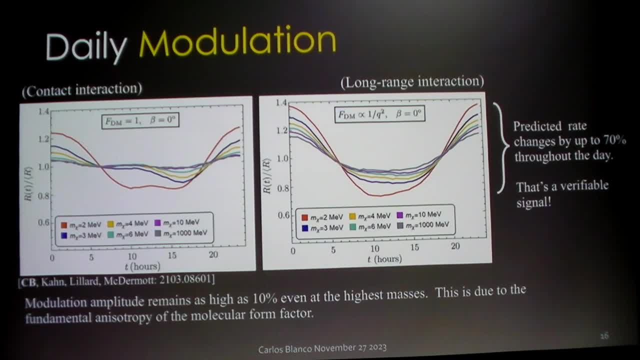 Okay, This is something that we take into account. This is a full simulation of the velocity distribution. It's not just asking you know how you change, if all of it comes from here. or all of it comes from here, Okay, Neat. 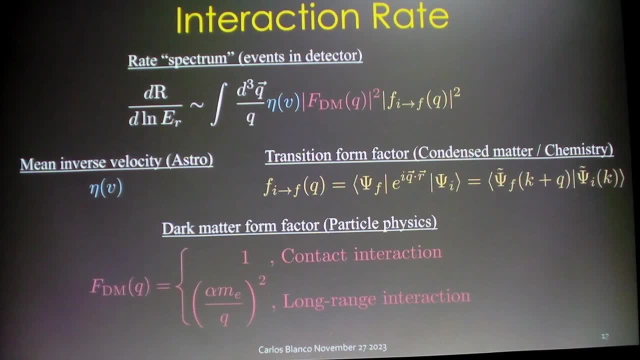 And this shouldn't be surprising, because what we've done is we've selected a target where this transition form factor is anisotropic, And so we should expect that. We should expect that the rate is anisotropic. That's what drives this. 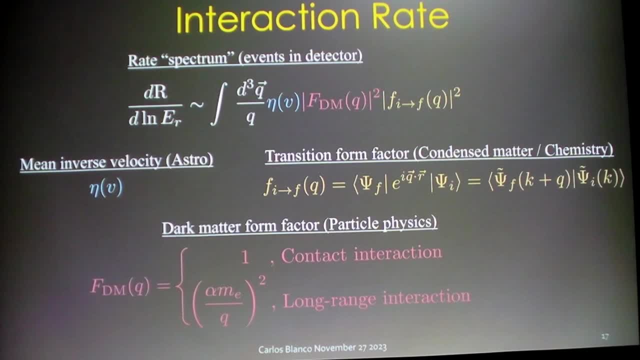 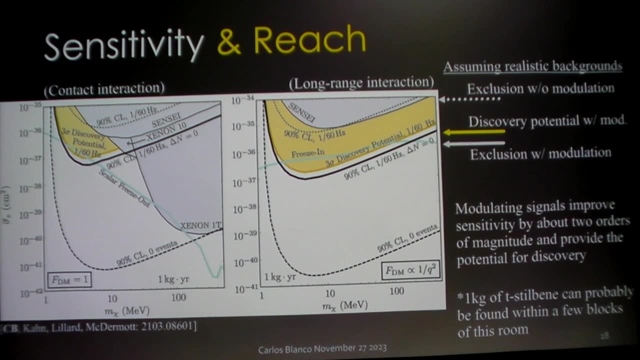 Here you were asking about this object. right, The velocity distribution. We modeled that fully in these simulations. And so what does this buy you? Well, say you had a crystal and you totally ignored daily modulation. Right, Say you were just looking at the paint can and trying to do cuts based on rates. 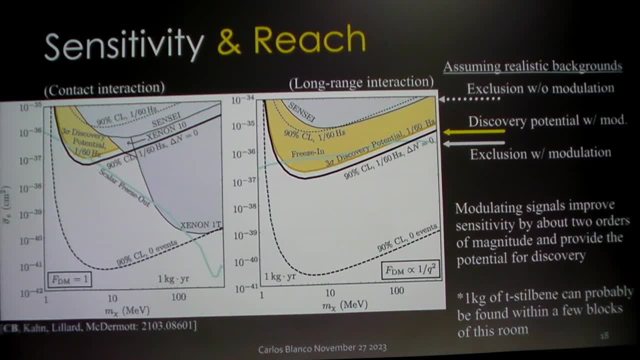 Well, there, for one kilogram crystal, you would have sensitivity. You would have these dashed lines. In looking for your daily modulation, you essentially get sensitivity improvements by two orders of magnitude. Okay, So that's this black line, And not only that, since it's a verifiable signal, there you have an actual discovery potential, not just an exclusion sensitivity. 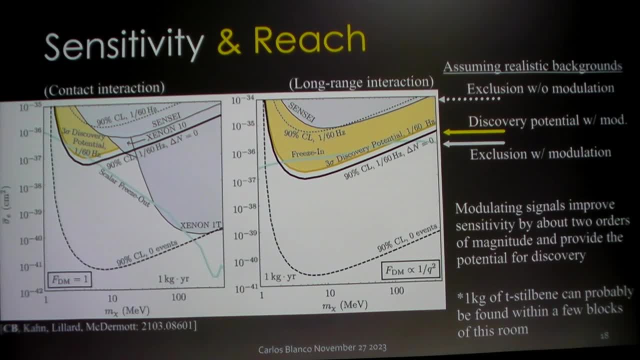 And so that's great. And these projections are for background rates from background rates of the PMT or your photo detector That are very much pedestrian-like. These are not futuristic. These are, you know, something like a one per minute dark grid. 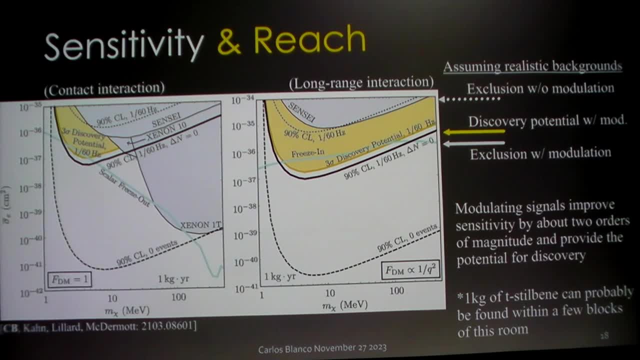 Okay, So what kind of a scale of an experiment is this? Is this like a paint can scale, or is it much larger? Yeah, One kilogram is about this big Wow. And you might ask: is that going to be expensive? 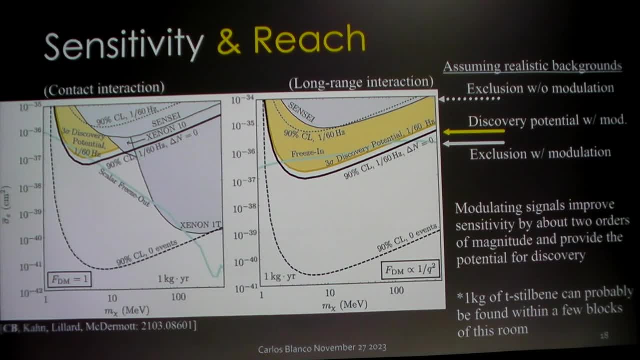 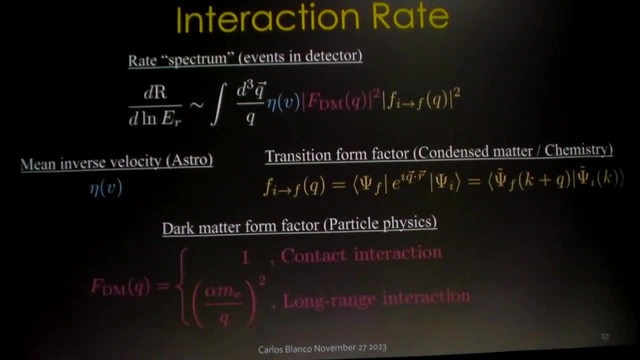 No, You can probably find a kilogram of still being within two blocks of this. This is found in every undergrad laboratory. So the graph you saw earlier This is an obvious one. Is this experiment or simulation? This is simulation. This is simulation. 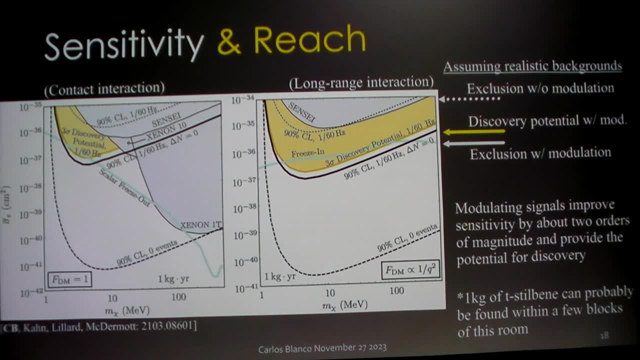 And, based on this simulation, we predicted this sensitivity. Okay, Now these blue lines, these blue lines here- are benchmark dark matter models that would give us the right relic abundance and that have a self-consistent thermal history in the early universe, And so that's where we expect dark matter to be. 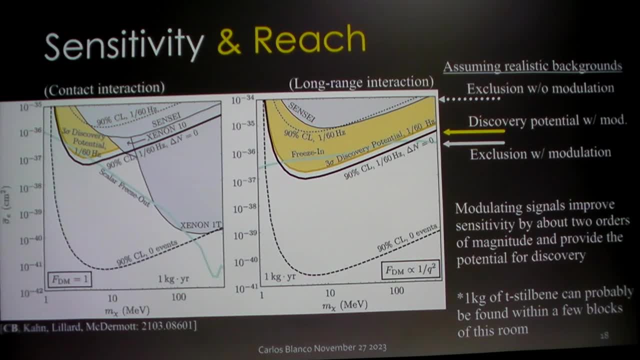 And so it's pretty surprising that with just one kilogram of still being, You can already probe something like a freeze-in scenario over two orders of magnitude, And you start to probe this scalar freeze-out scenario with a kilogram. So this got quite a bit of attention. 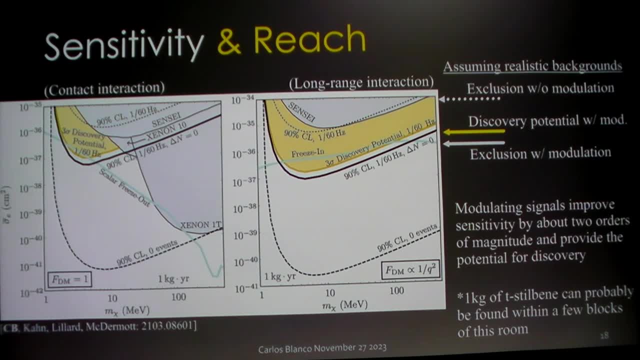 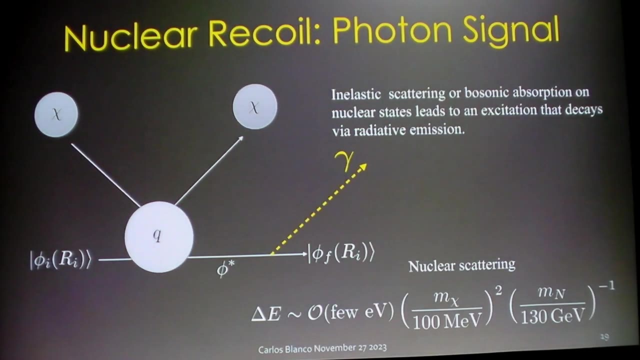 And it's now being developed at Fermilab. They're characterizing the materials actually here in California And then they're going to be flown to Fermilab where they're going to be deployed. So we're quite excited about that. What happens if now you want to look for not just the electron coupling but say you want to go after dark matter models, that couple instead to baryons? 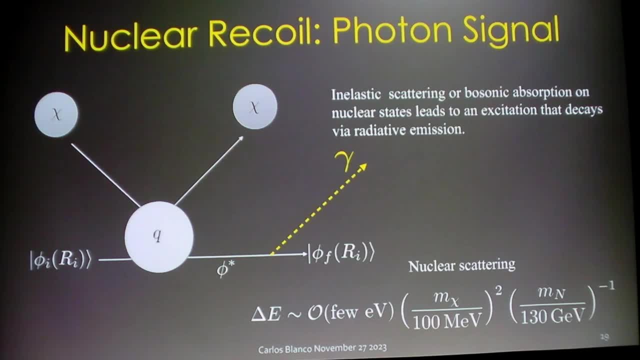 Then you're looking for nuclear recoil And you can do the same tricks, right? You can say: how do I excite electrons using nuclear recoil and how do I look for the photon signal that you get from that? Well, let's think about how we do that with atoms, right? 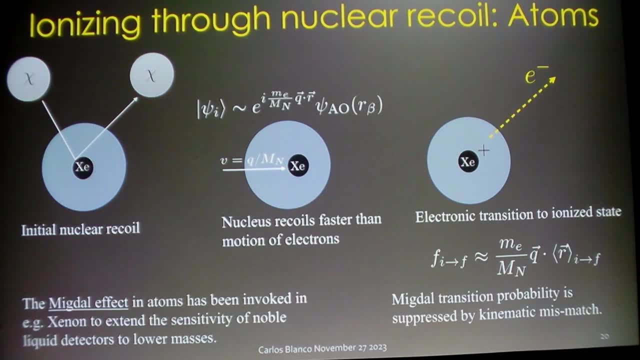 So you can ionize an atom. You can ionize an atom by recoiling off the nucleus, And the way that you do that is the drug: when it comes in, it recoils off the nucleus And from the point of view of the nucleus, now all of your electrons have picked up a phase and are no longer in the ground state. 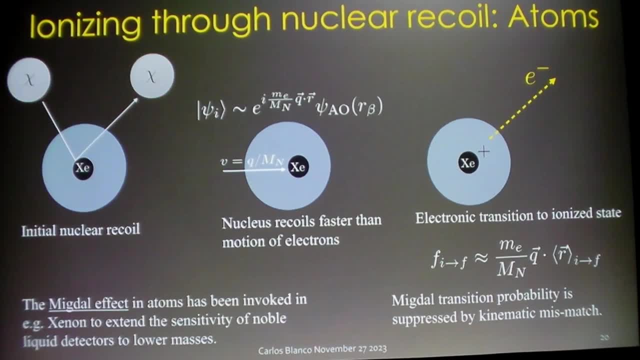 And so you can just calculate the probability of them being ionized. And this is what dark matter experimentalists call the MIGDO effect, And this has allowed people like the Xenon collaboration or the liquid argon community to take their sensitivities and stop at one GeV and go towards lower masses. looking for this inelastic second-order process, 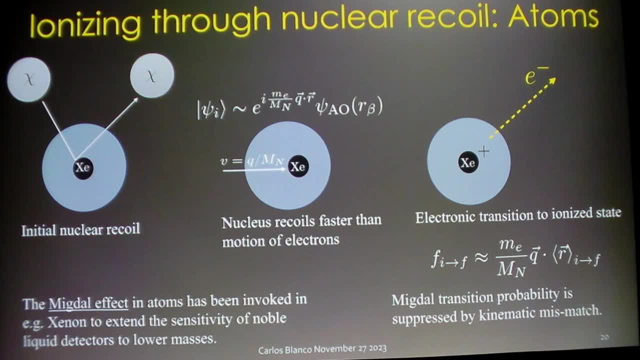 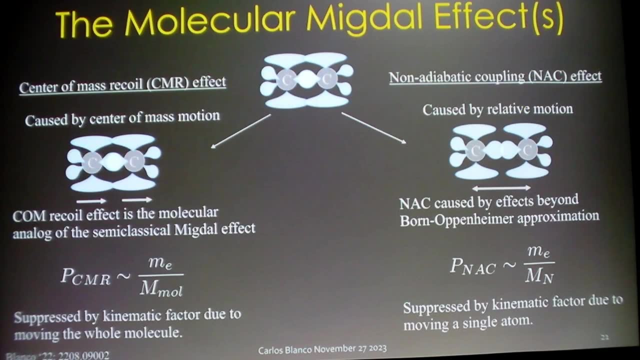 And so this has, you know, really revolutionized the way that we look for light to dark matter with these noble gas vats. And so a natural thing is: well, do molecules have a MIGDO effect? And, as we discovered last year, yes, they do have a MIGDO effect. 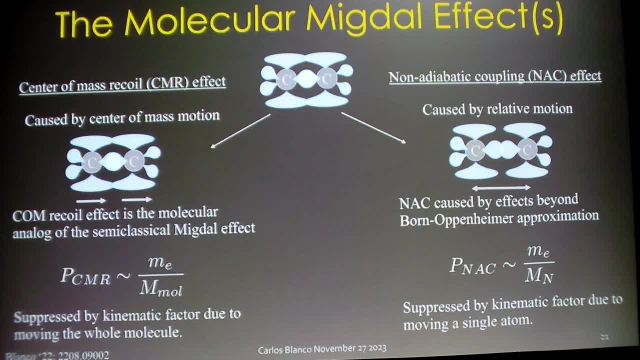 Not only do they have one, they actually have two, And the way to understand this is that if I have the most basic molecule that you can form, which is just two atoms, how do you shift the nuclei? Well, you can decompose all of their motion into a center of mass motion, where they move together. 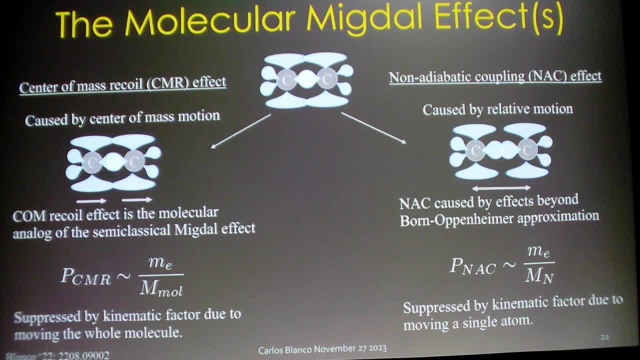 and a relative motion, and each one of those two things come with their own separate probability of excitation of the electrons. And so the center of mass one is totally morally equivalent to the atomic MIGDO effect, whereas this relative motion one is something totally new. 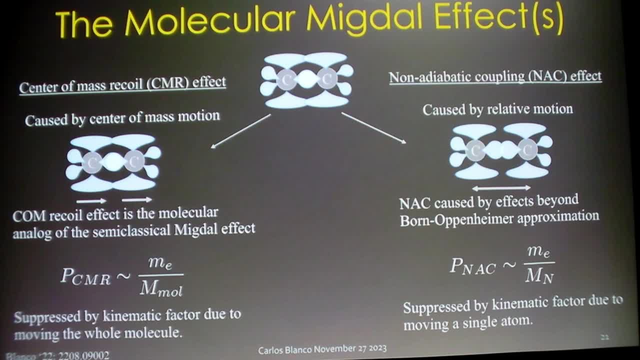 that only exists in these scintillators and that's the non-adiabatic coupling MIGDO effect, And so this comes from effects beyond the Born-Oppenheimer approximation, Importantly because these internal deformations don't have to move the entire molecule. 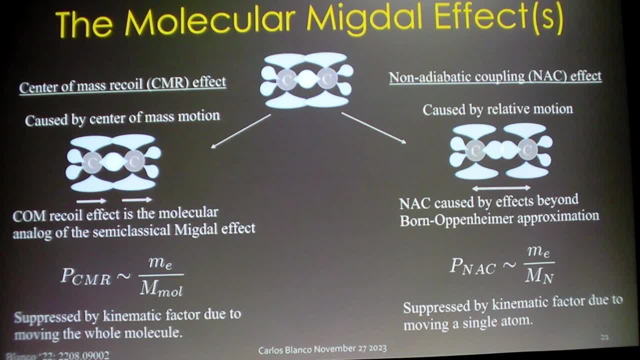 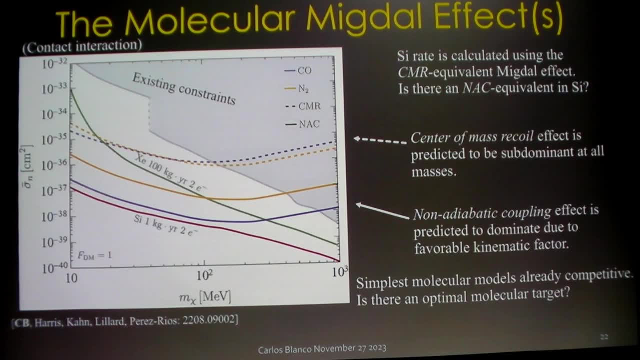 they don't pay the same kinematic penalty as the center of mass recoil effect, And so they're expected to dominate across all dark matter masses. And when we put this all together and we turn the crank, we find that that's totally true. 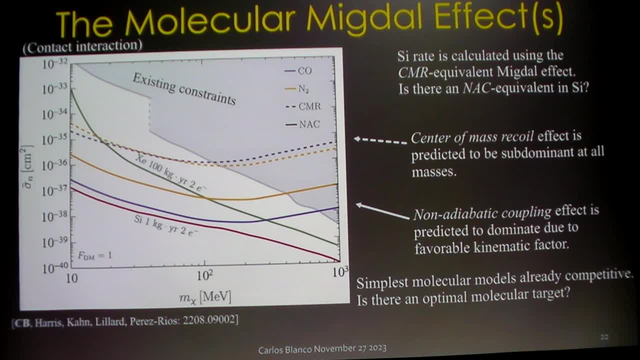 So for two toy examples of carbon monoxide and nitrogen, which you would never actually use in an experiment, they're just things that we can calculate almost exactly. We find that the sensitivity coming from the non-adiabatic coupling effect totally dominates the center of mass recoil. 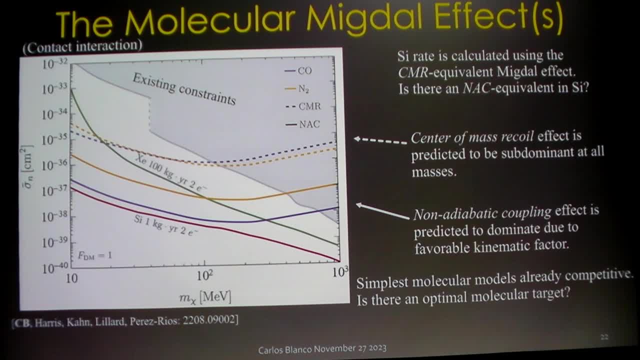 And we also find quite interestingly that even for these very dumb molecules we're already within less than a factor of two from the equivalent silicon sensitivity. So these are sort of the bleeding edge experiments now, And the silicon sensitivity comes from a calculation of a MIGDO effect. 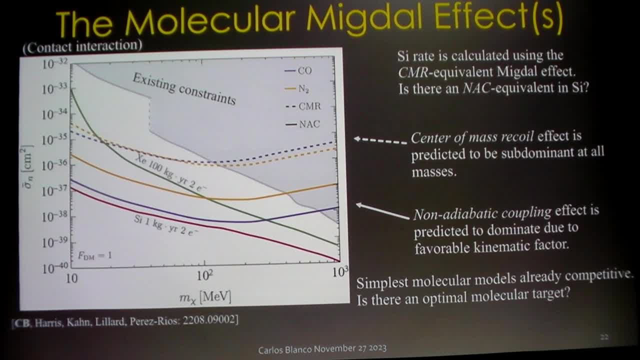 that only takes into account center of mass motions, And so a natural thing to ask is: does the non-adiabatic coupling effect exist in silicon? And if it does, then the community should calculate it, because then this line should be expected to actually be down here. 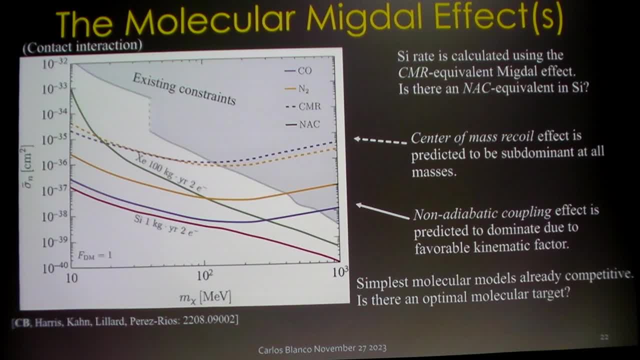 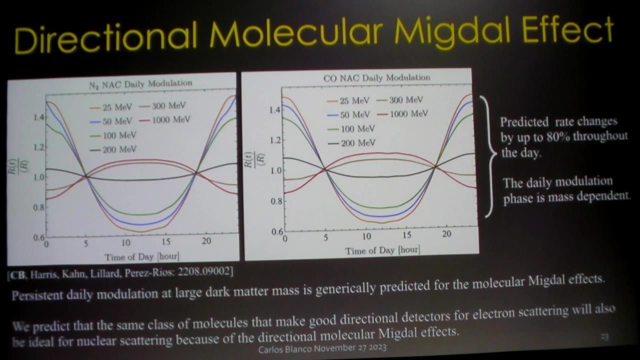 And the silicon community can enjoy way higher sensitivity that way. The other thing that one can ask is: well, how do you go about finding really optimal molecules? And so I'll get to that. Another thing that you get for free is that the molecular MIGDO effect is also directional. 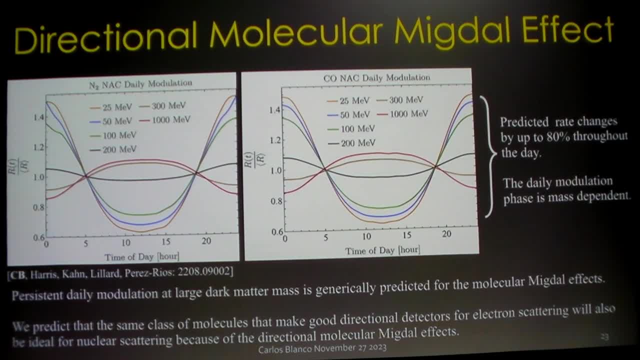 because molecules aren't isotropic, And so you can make these similar daily modulation curves And you'll notice something kind of subtle here: As a function of dark matter mass, the phase of the oscillation changes, And so in these experiments you can tell the difference. 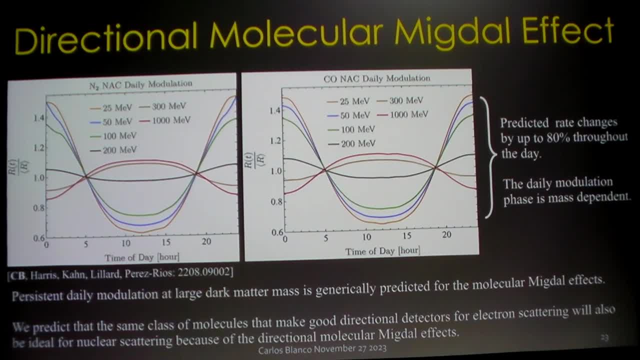 and I believe it's the only kind of experiment that you can really do. this is you can tell the difference between a light dark matter particle that's strongly coupled versus a heavy dark matter particle that's slightly coupled. This was very surprising to us. 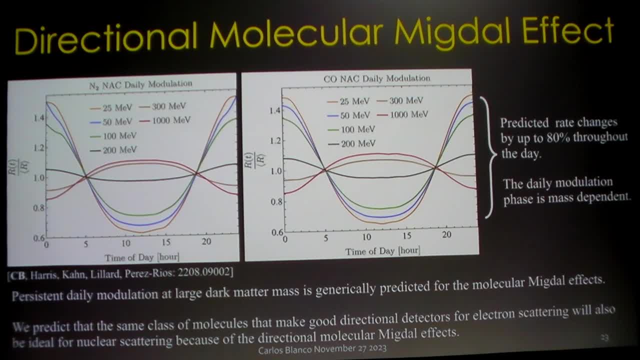 It's a very subtle effect that comes from the fact that there's two probabilities that factorize from the nuclear matrix element and the electronic matrix element, But we were quite excited about this. So how do you go about finding molecules that are optimal for this? 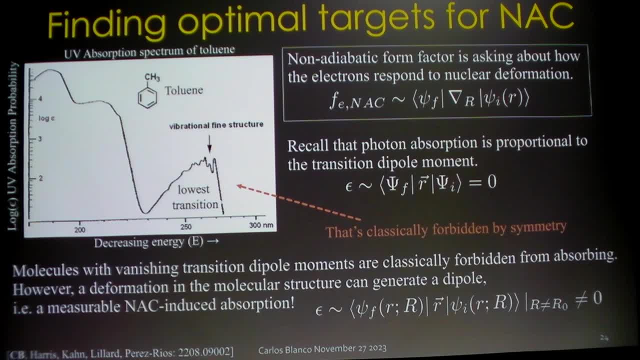 Well, it turns out, you can actually observe the non-adiabatic coupling effect in real life with spectroscopy experiments. So this is a molecule called toluene, And the first electronic transition of toluene is classically forbidden, because this thing has no dipole moment. 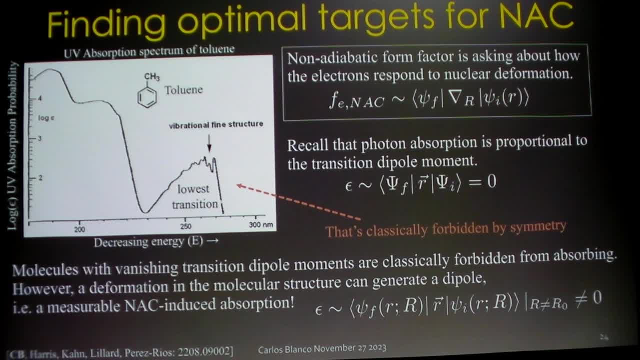 And so you go out and you measure the electronic transitions and you find, well, it's actually there, It's visible, It's quite visible. Why is it there? It's classically forbidden. Well, it's there because the vibrations of the molecule drive a non-equilibrium dipole moment. 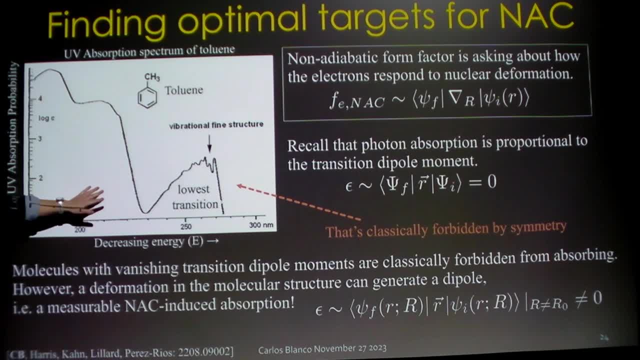 And it turns out that the matrix element that dominates this kind of forbidden transition is the same matrix element that is responsible for the non-adiabatic MacDowell effect. And so, whereas in the atomic case, the MacDowell effect has never been measured, 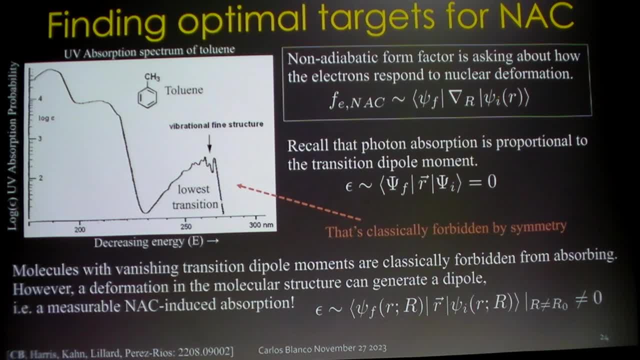 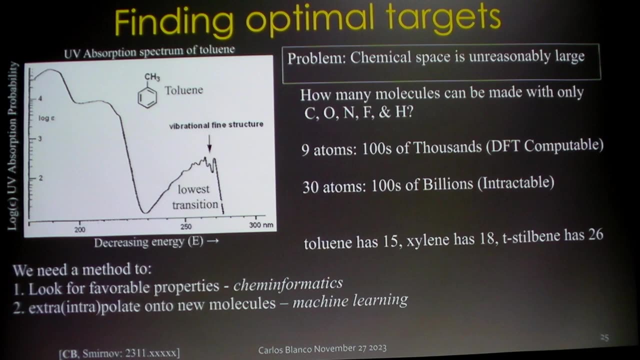 in molecules. it's essentially been measured since the 50s. So that was really exciting for us because it means that we can do some quite interesting data mining to look for really just the best possible detectors for dark matter, And there you run into a really complicated roadblock. 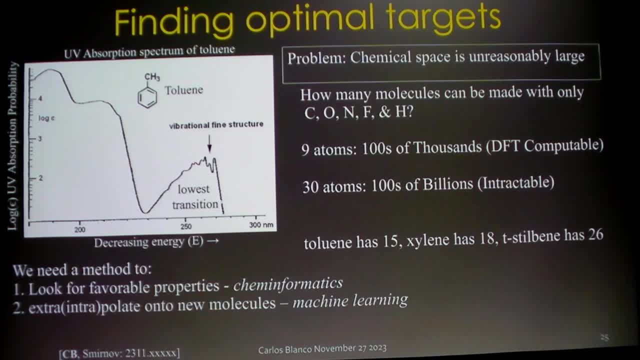 which is the intractability of molecular space. So the question you can ask yourself is: how many molecules can I make with just these basic atoms? If you have nine atoms, you can make hundreds of thousands of them and that's kind of computable. 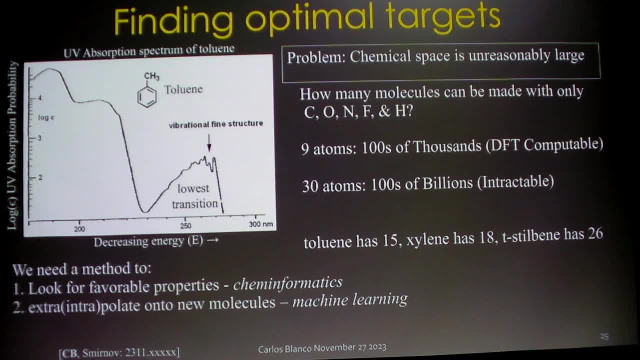 You can do density functional theory on this many molecules and it'll take a ridiculous amount of time. but you could do it at least in principle. But when you go up to 30 atoms you're now totally intractable. There's not enough computational power in the world currently to do this. 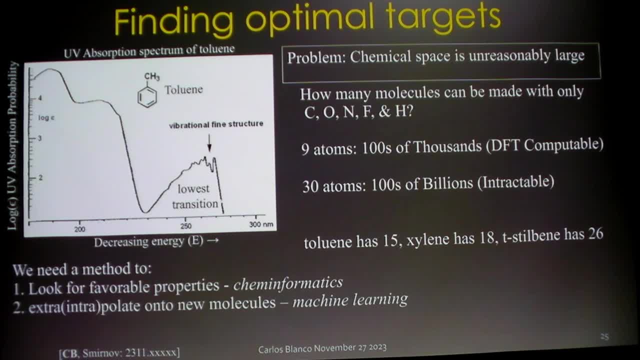 And for comparison, this trans-stilbene molecule that we've selected as just the simplest candidate already has 26 atoms. So looking for optimal molecules by computing each one from scratch totally intractable. So what do we need to do? 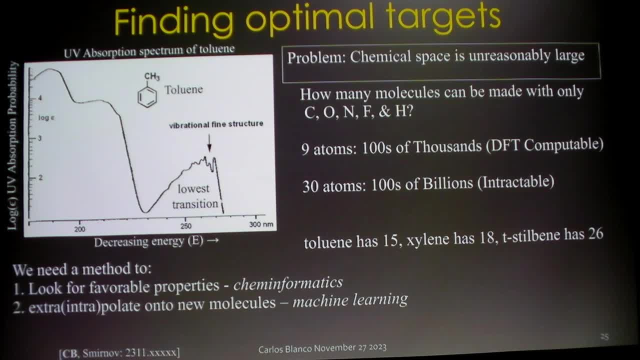 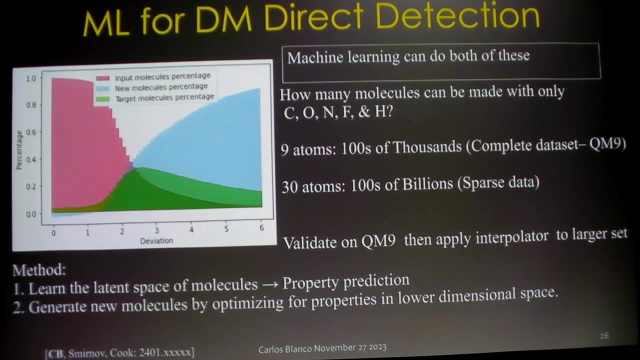 Well, we need to look for favorable properties. that's called cheminformatics, and that exists as a field. But we also need to interpolate from existing computations into new molecules, And for that machine learning is optimally suited. And so that's what we're doing now. 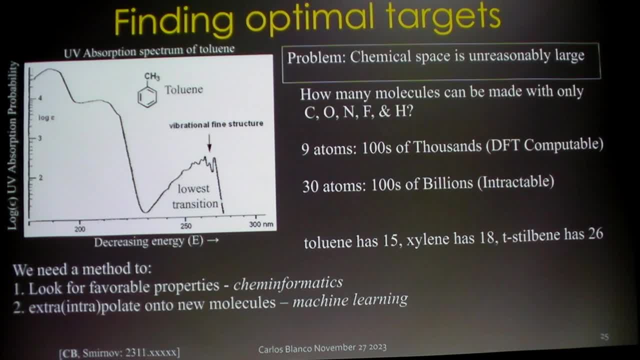 So optimal in terms of what The best molecule to make a dark matter detector? So to maximize the sensitivity to the dark matter. Maximize, you're not maximizing the cross-section of the matter. so you were looking at the sensitivity, So the sensitivity, that just means maximize the rate of the signal. 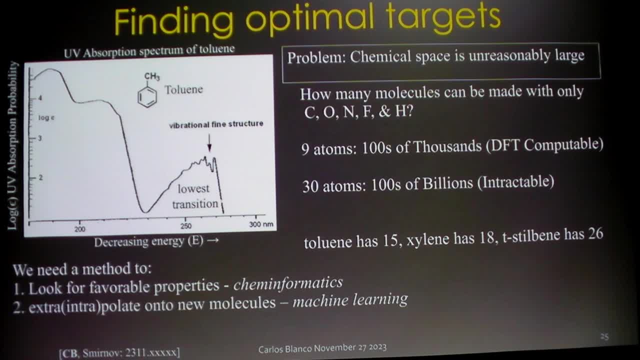 with respect to the rate of the noise. So that means maximizing the non-adiabatic coupling matrix element, maximizing directionality. All of these things need to be For a given. you assume a cross-section of the dark matter To the electron. 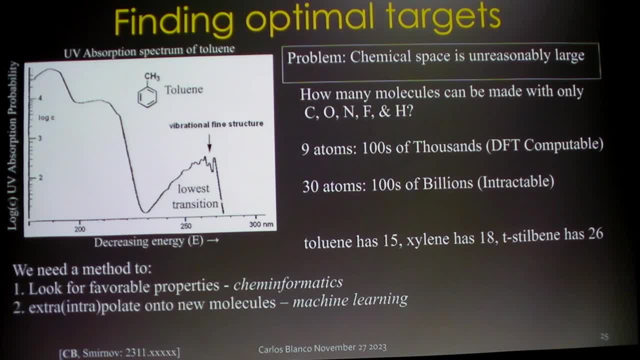 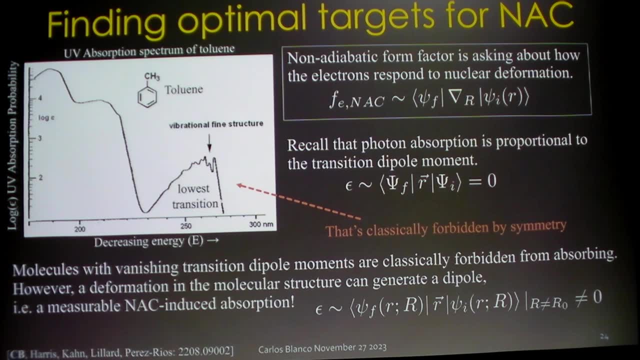 And that's some number that will vary, but for a given value of that, you want to know how big of a signal you have. But you can only do that. You don't. it's a pre-factor, right? You don't know this pre-factor. 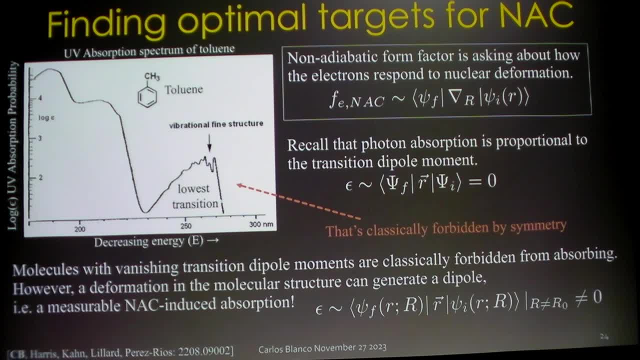 So you want to be able to after interaction, how much you can get into excited states, then how much you can turn into photons. So that's, it's a latter two-state you're interested in. So we're basically optimizing this matrix element. 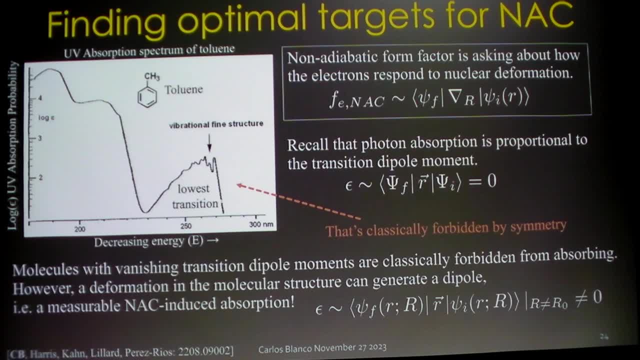 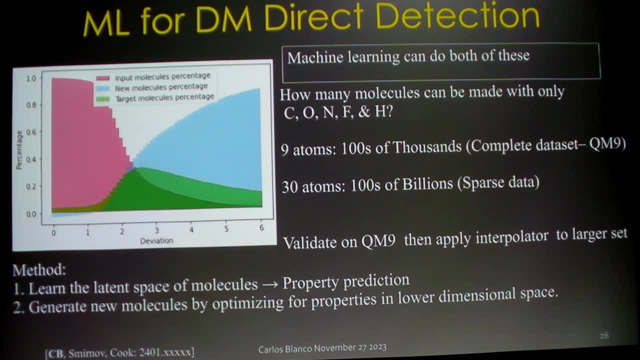 This matrix element and all the other electron matrix elements that we consider for scattering. And How do we do that with machine learning? Well, let's start with a small data set, A data set called QM9, which is quasi-complete. 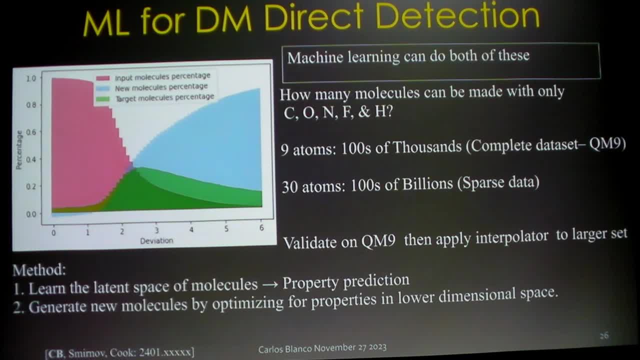 This was a huge effort. It's essentially like the human genome project, but for molecules. They tabulated all possible molecules that are experimentally viable up to nine atoms, and they computed a bunch of DFT on them, And so we can use that as a training set. 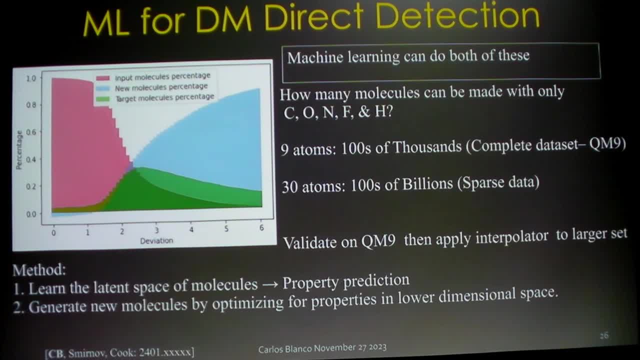 And to validate a machine learning network that we made bespoke for this task, and then we can say, okay, take that network and now apply it to a sparse data set that has much more atoms per molecule, and then use essentially a fancy interpolator. 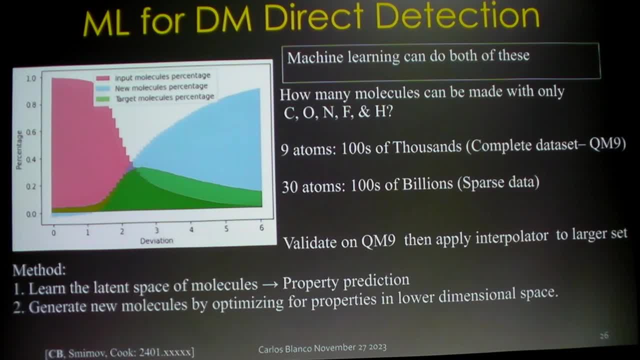 which is what machine learning is, to really complete the data space, And so this is a plot that's kind of hot off the presses, And what it's showing you is as a function of essentially an order parameter in our network. this is a generative network. 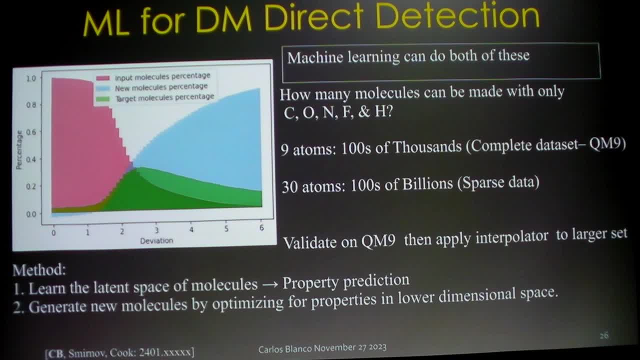 what we do is we put in a data set a subset of QM9, right, And that's the rut. And we ask: generate a bunch of molecules. And so, as a function of this order parameter, we generate essentially all the data set. 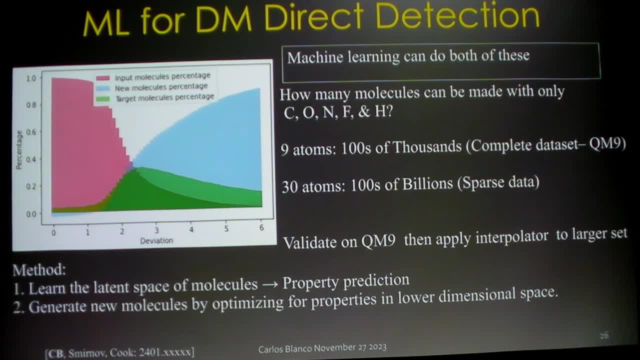 and only from that subset, And as we increase it, we're generating far less of what we trained on and far more new molecules and far more molecules that belong to the rest of the QM9.. Now new molecules here, really just says. 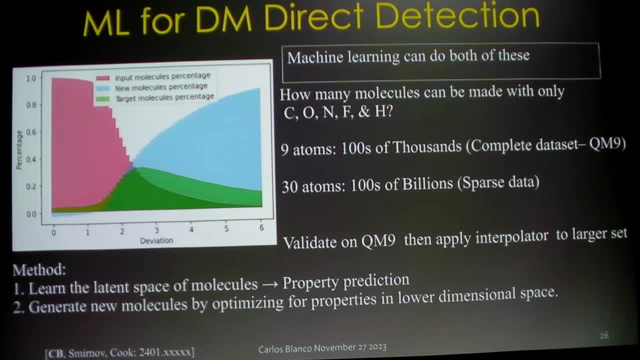 molecules that are not experimentally vital, And the fact that the machine can tell the difference between these three populations means that it's really learning chemistry. It's pretty beautiful. So you basically predict: let's give you 30 atoms, and you're going to try to find your similar arrangements. 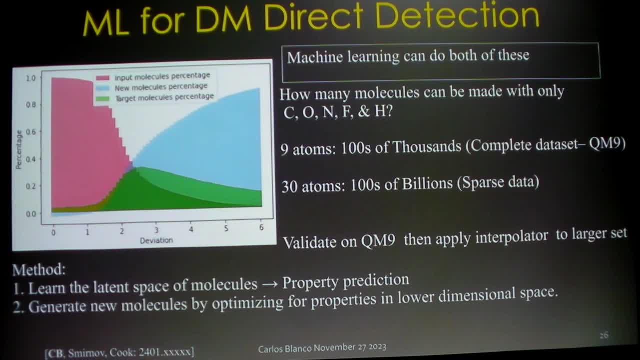 The thermo is stable And they actually can be made. That's right. But that's actually. it's kind of like in medicine. they used to have very limited parameter space to do drug discovery, But here it's a tricky business. 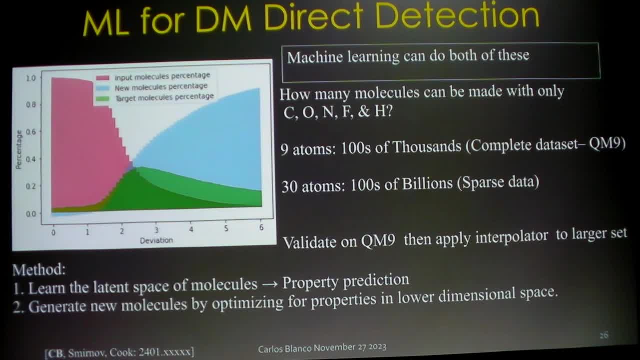 It's very tricky. You can say you can make a molecule like that, but in reality you won't be able to make it. Yeah, so all the molecules that are known to not be that you can't make are in blue. 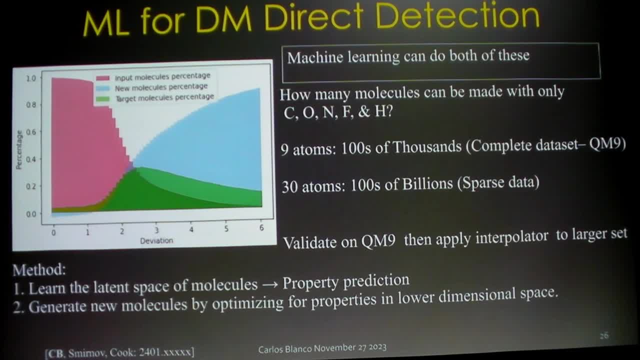 The ones that you can make are in these other two populations. And it's funny that you bring up drug discovery, because this research is the only dark matter project that I can think of that's funded by the NIH. You've got a high school for screening work. 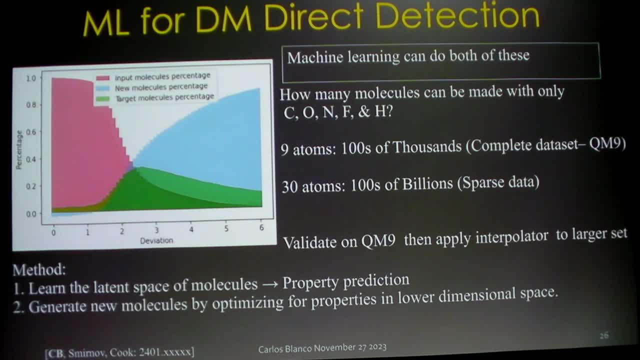 That's right, And it gives you tens of thousands of molecules in one shot. But here you're basically doing similar things Exactly, And that's why we use very similar machinery. So I'm sorry, I don't understand this plot. 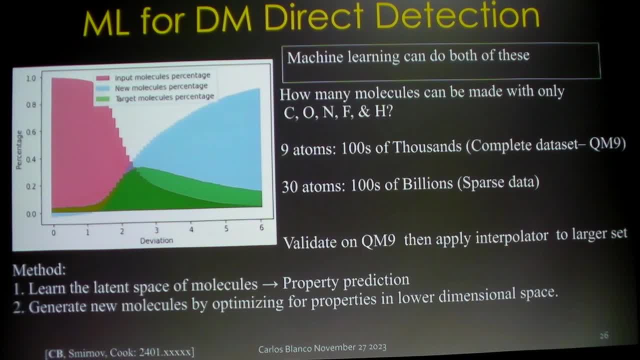 So the deviation is: what is your training sample right? If you go to the right, you're using less and less training data. which is the red? Not quite. So you can think about this as a knob that allows your black box to either generate things. 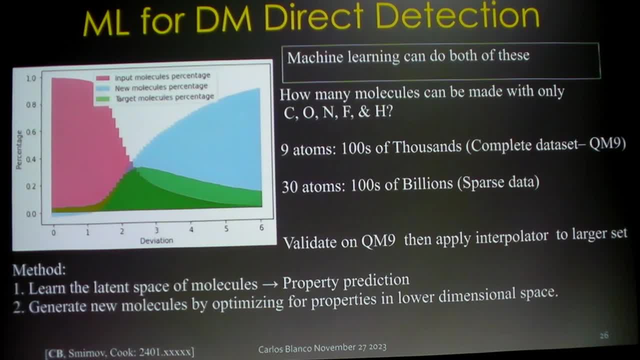 that are very close to the training set, or can explore a latent space farther and farther away from that initial training location. And as it's able to diffuse out and to deviate from its original location, it's able to produce new molecules and molecules that belong to a set that you know of. 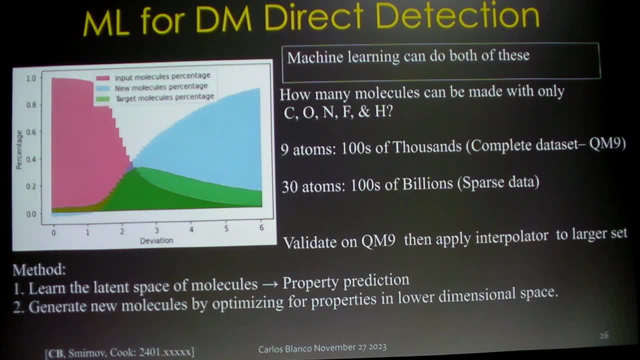 but that is a superset of your training set, And so that basically means that it's learning the manifold where molecules live, But it knows the difference between the blue and the green or the blue and the green. you only know because of truth data. 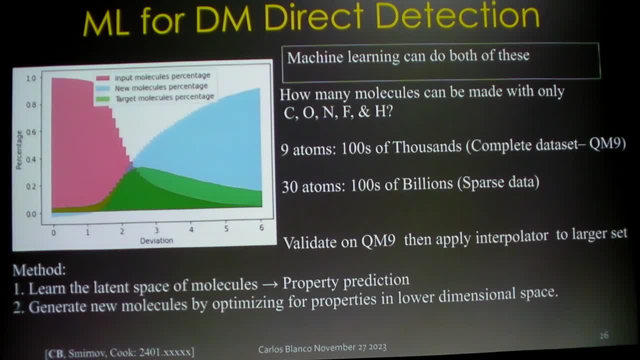 Well, we know the truth data between the blue and the green, but we trained the machine to also tell the difference right. So blue are all molecules that are not found in QM9 because they are not experimented with, And so part of our network is a subroutine. 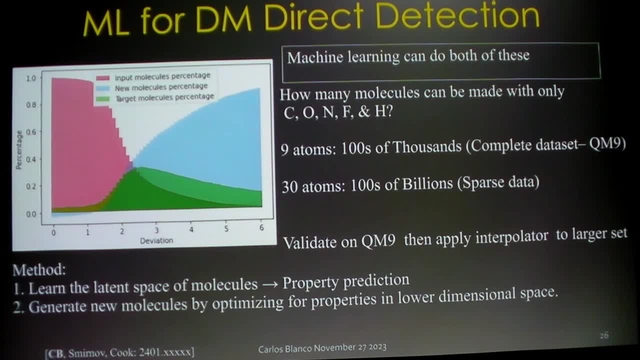 that is able to tell the difference between the submanifold, that is possible and whatever else. Yeah, Okay, So this is really interesting. Stay tuned for this. In the next few months we'll put this out. Okay, I only have a little bit of time. 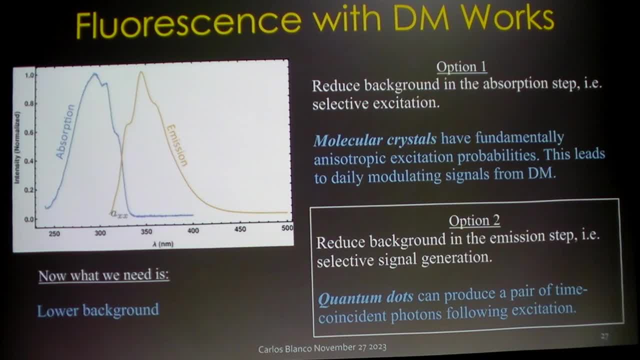 so hopefully, I'll be able to tell you about this next part, which is: how do we reduce backgrounds beyond that? Well, now we can focus on the emission stuff right, And one way to do that is to look at nanomaterials. 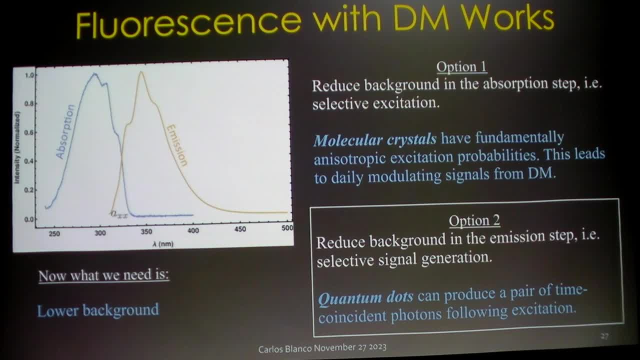 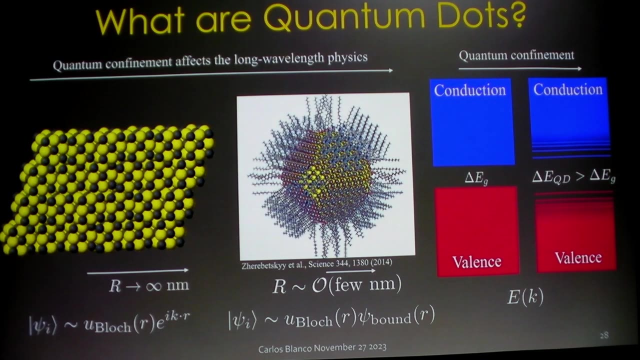 So I will just tell you that there are these things that are called quantum dots and they can give you signals that have very interesting statistics that are far different than random statistics. Okay, so what is a quantum dot? This is a computer-generated graphic. 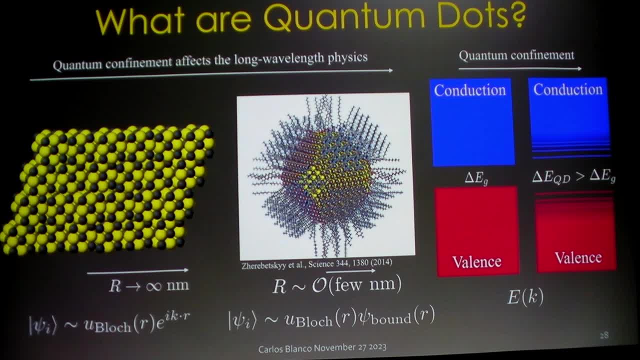 A lead sulfide quantum dot is an anisotopic crystal and on its surface you have these molecules that are just there to stabilize the crystal from falling apart And energetically, what is happening can be understood by first considering an infinite crystal. 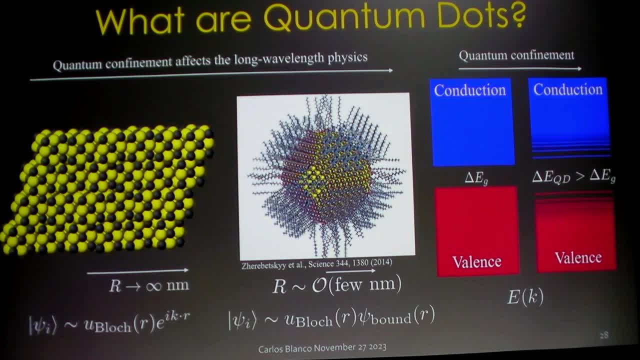 So let's consider an infinite crystal here. The electrons here live in block states which are just a block piece. that tells you about the microphysics and the symmetries in the lattice. So this is a free space wave times, a free plane wave right. 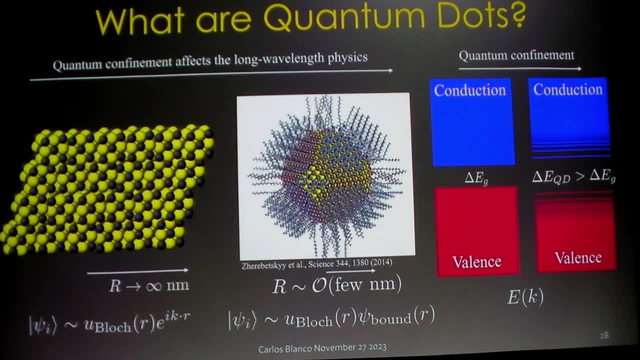 The solutions of the Schrodinger equation in free space. As you imagine, taking these boundary conditions from infinity and shrinking them to the size of the wavelength of an electron, your states now look different. The microphysics stay the same, so the block piece remains relatively unchanged. 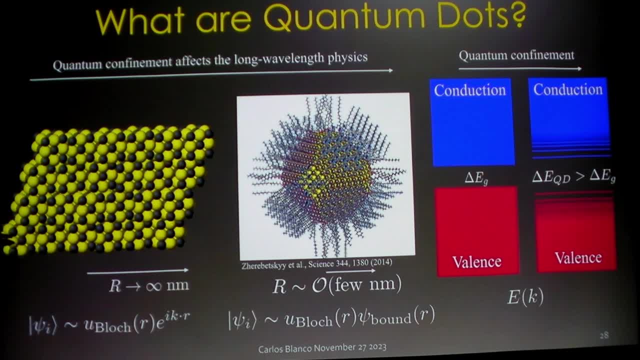 but now your free space wave is now no longer a solution and that piece really turns into what's called an envelope, a bound envelope, And that's sort of the first-order understanding of what the electronic states look like in these quantum dots And energetically what that looks like. 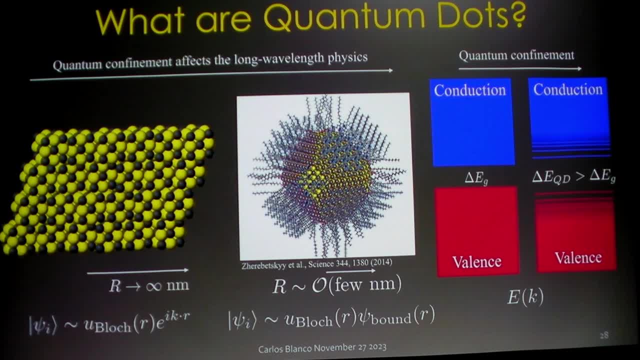 is where you would start in the infinite crystal, having some continuous valence and induction bands. The act of quantum confinement allows you to resolve the band edge states that really look like particle in a box. Okay, And it's interesting, because the radius the characteristic size of your crystal. 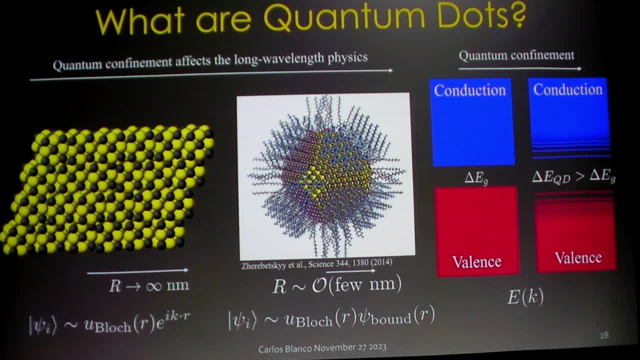 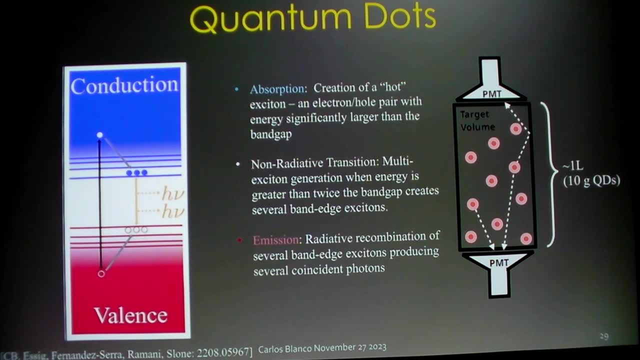 controls your effective band gap. So you have an extra knob that you can use to tune the electronic properties. What's more is you get this interesting effect that occurs when you excite an electron from your valence band deep into your conduction band. 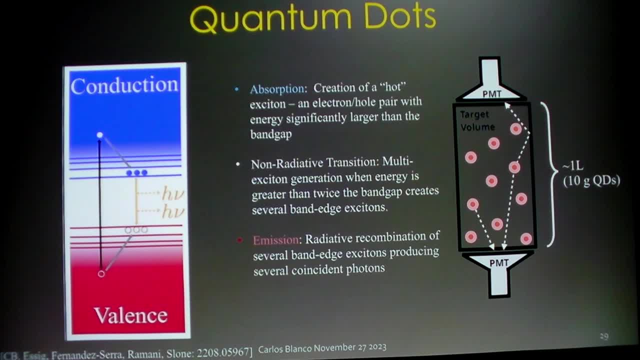 creating what's called a hot carrier. These things can relax down by a couple of ways. One is they can emit a bunch of phonons, but now you're living in a nanocrystal and your phonon density of states is very different. 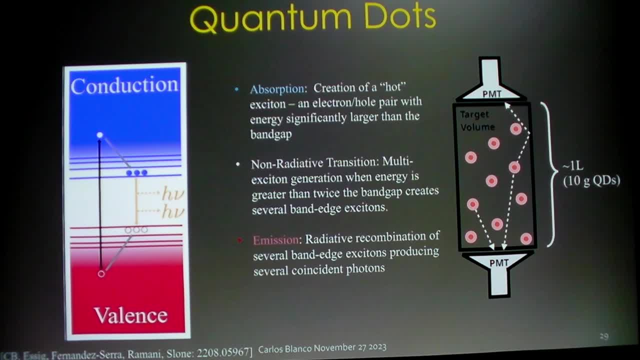 And so that process turns out not to be very different. It's very efficient, And instead you relax this hot carrier by generating more excitons that now live on these band edge states, And because you have multiple band edge excitons, they can then recombine the electrons in the holes. 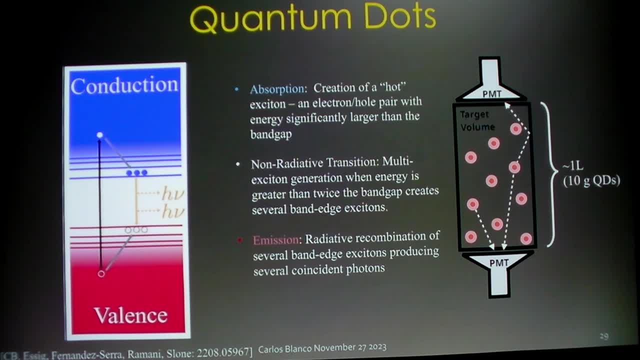 and give off photons that are correlated in time to within the radiative lifetime of your exciton. Okay, So what does this mean practically? What this means practically is you have these chromophores called quantum dots. You put them in a vat that looks the same. 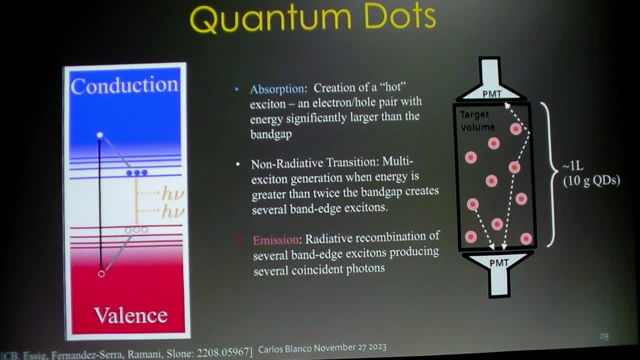 the same paint, can you have two PMTs, and instead of looking for single photon counts, you look for correlated double photon strengths? Thermal noise has a very, very hard time mimicking that, it turns out, And so you can reduce background very efficiently this way. 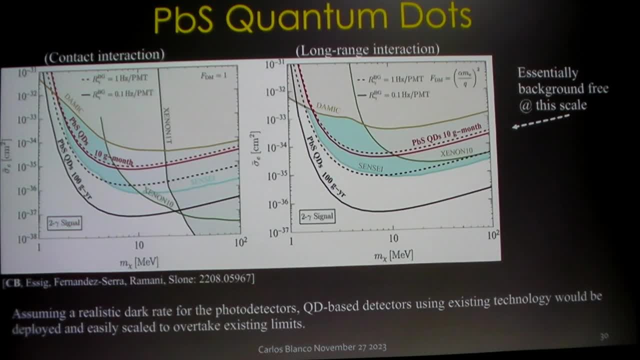 And so these are projections of what those sensitivities will look like for two different scales of deployment. So here you have a 10-gram-month exposure of quantum dots. This is like a one-liter volume of quantum dots suspended in liquid. And at that scale 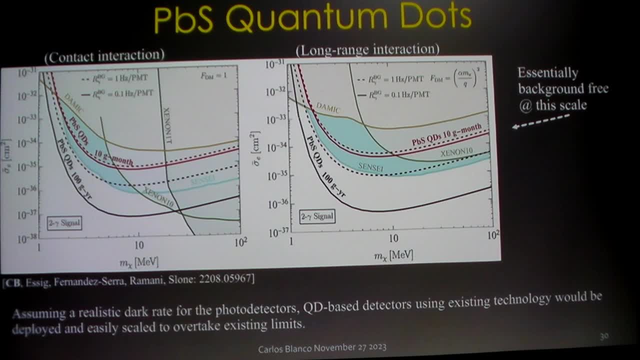 this sensitivity is kind of independent of the dark rate of your photodetector, if the rate is in order of one hertz. So even with these off-the-shelf parts you can already characterize these perfectly, because these are essentially background-free at this scale. 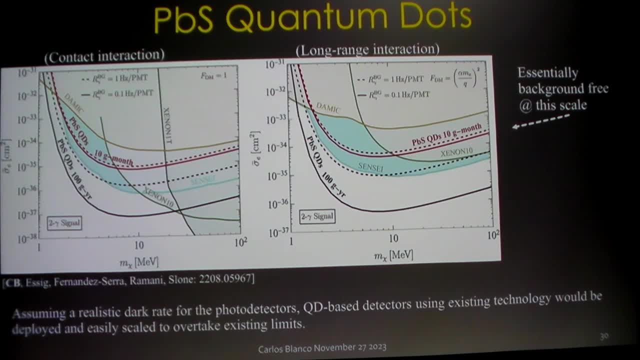 So you build this experiment, you characterize it, you're essentially background-free, you can do it, And then you scale it up by a factor of 10, and then you can start telling the difference between background and this ability to do this double-counting thing. 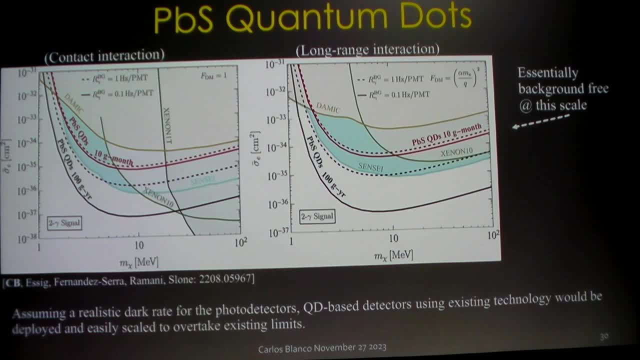 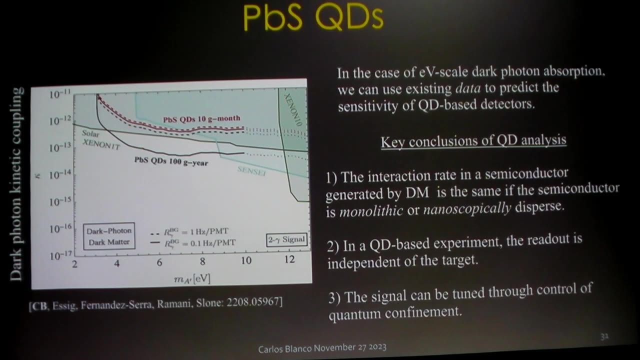 allows you to go from here all the way down to here. So this is this order of magnitude improvement that I was talking about before, And this is all existing technology. This is just a clever way of going after these signals, And so people were quite interested in this. 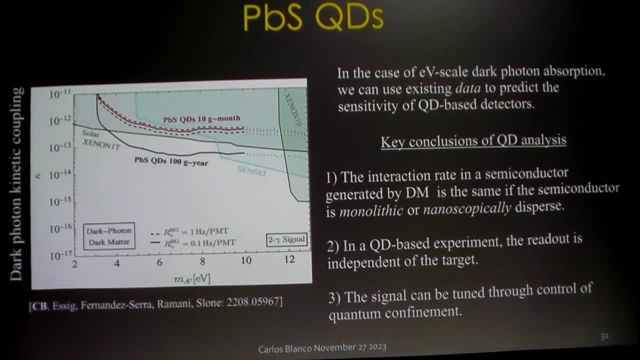 also because there exists honest-to-goodness data that you can look at to do sensitivity studies of, say, light, dark matter, bosonic absorption. So you'll see that these sensitivity curves are jagged and that's because this comes from honest-to-goodness data. 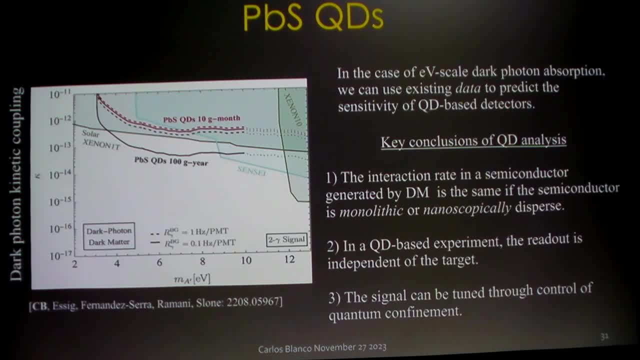 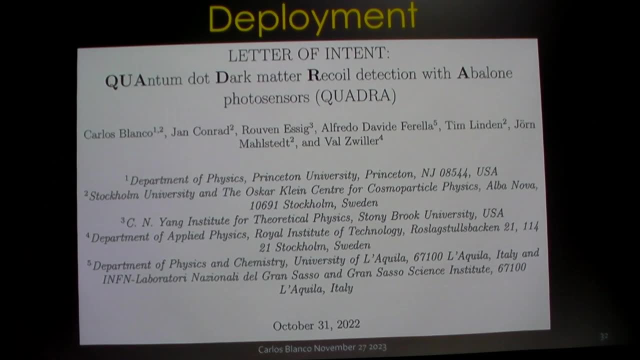 This is like a pre-calibrated experiment, if you want to think about it that way, for absorbing something like a dark photon. So some very good experimentalists in Stockholm got very interested in this, and so we wrote a letter of intent, starting a collaboration called the Quadra collaboration. 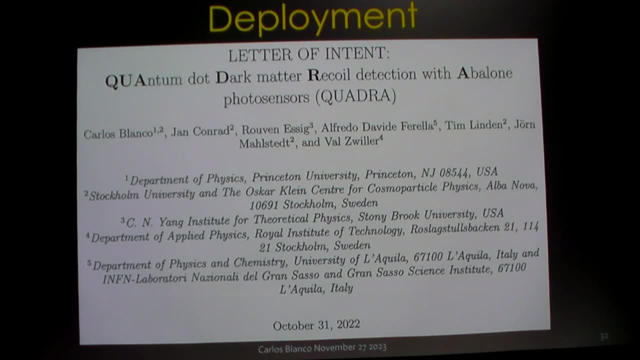 to actually deploy a quantum dot-based detector. At the same time, there's an MIT team that is also trying to deploy this, led by Lindley Winslow, And this is a CAD rendering of what that might look like in sort of its fully upscaled state. 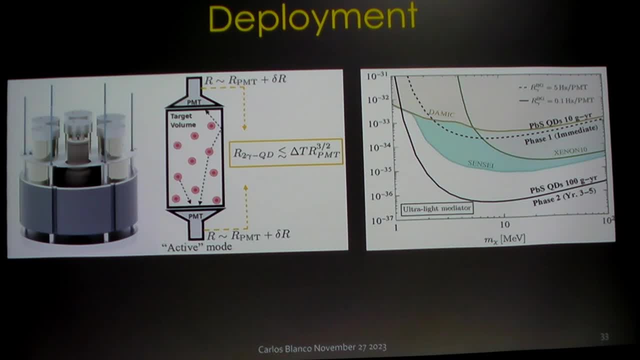 And so these are sort of next-generation PMTs that are being developed for the Xenon collaboration that we're going to be able to use afterwards, And it's going to be deployed in two phases: An intermediate phase, which is this totally background-free phase. 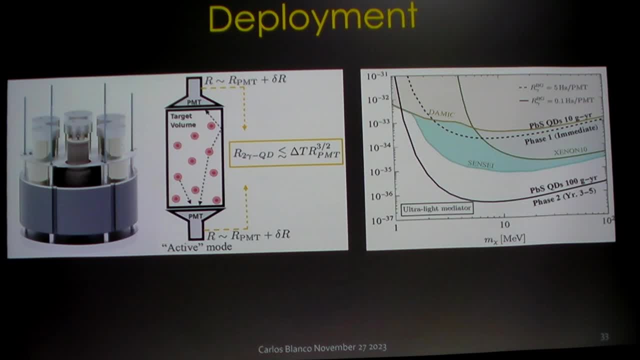 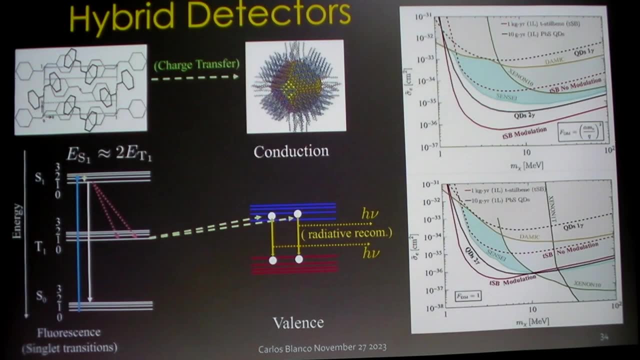 where we characterize and then we deploy it three years later And the expectation is that we'll outdo pretty much everything in the field for sub-GE dark light. Okay, Can you bring these things together? Can you do the selective excitation? 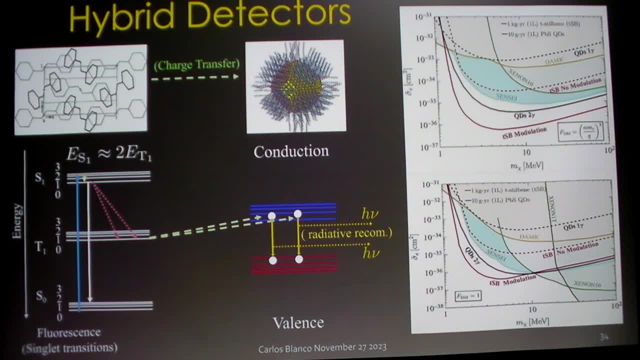 and the selective emission. Can you bring them together in such a way to get multiplicative background reduction? I think yes. So this is something that I'm working on right now And this would be the- You know, the next stage in this research program. 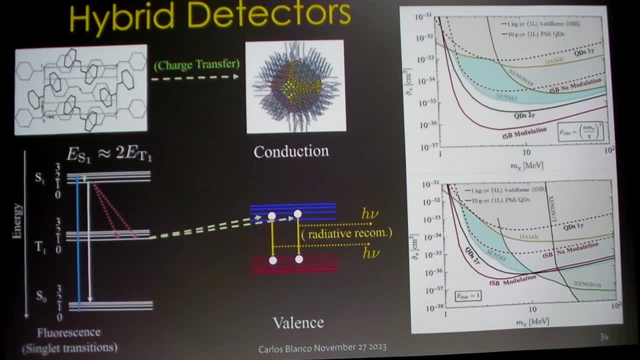 would be to form these hybrid-type detectors where you have this directional absorption followed by a charge transfer and a radiative recombination in time-coincident photons. And if this is possible- and there are very good reasons to think that it's possible- the multiplicative effects are kind of ridiculous. 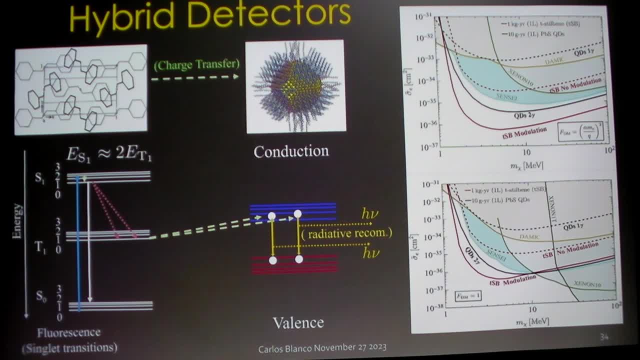 So these plots? what they show are the individual sensitivities of a one-kilogram detector of quantum dots and a one-kilogram detector of trans-still beam in the dark red and dark black. Okay, Individually, that's how good they do. 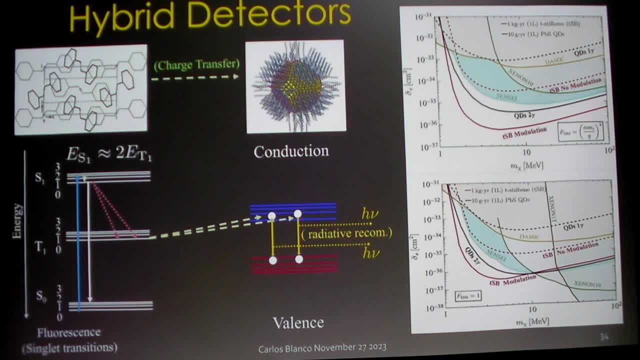 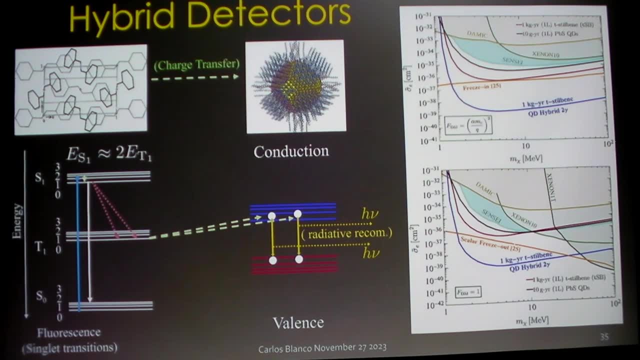 They do better than anything else in the field, but they're still within reach. If you put them together and you get a multiplicative effect, you're now doing better by many orders of magnitude. You'll be able to rule out freeze-in and freeze-out. 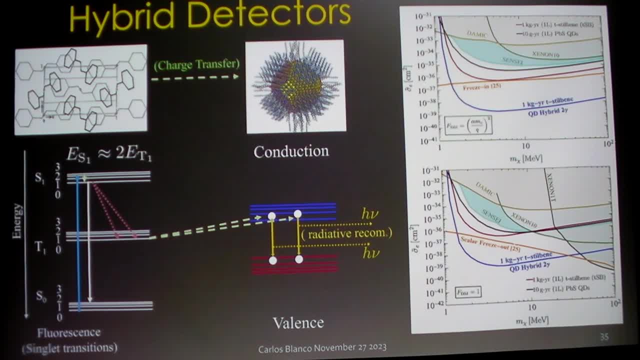 in the sub-GE parameters, You'll be able to control the entire space entirely. Why do we expect this to be the case? Because there is experimental data to show that this charge transfer happens. It turns out that the same process that governs this dark matter detection scheme. 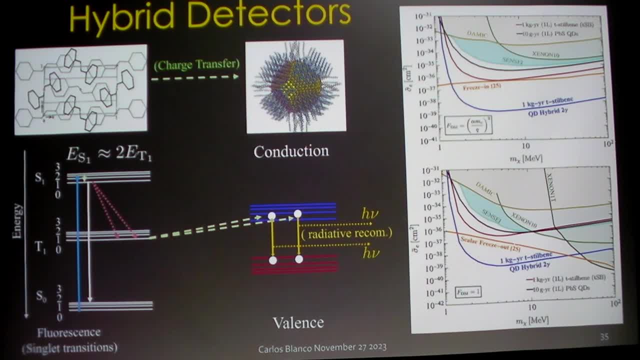 is the same kind of processes that the private sector has been really interested in because they will break the Shockley limit of photoabsorption. So this is essentially like it would be the best type of solar harvester, but instead of having to be very clean and marketable. 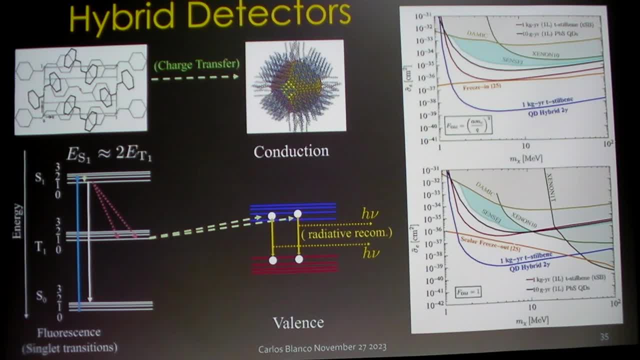 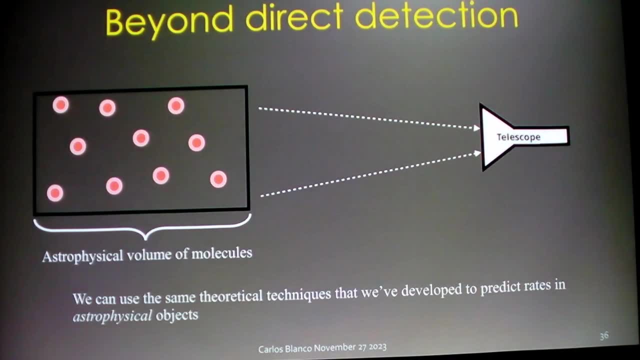 we can make it large and not very sensitive to the sun but extremely sensitive to dark matter. Okay, I think I have five more minutes so I'll tell you about going beyond direct detection with these techniques. So I've mostly just told you about what happens. 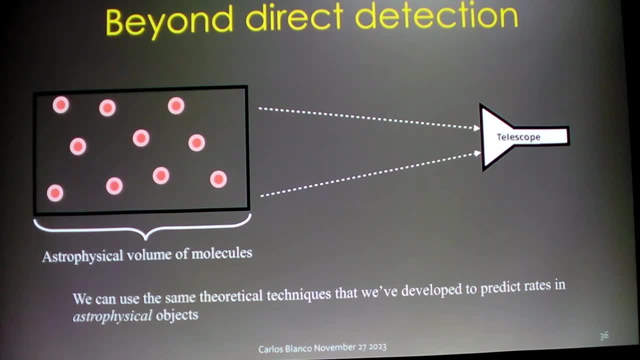 if you stare long enough at chromophores in laboratories. And these chromophores are just batches of molecules. But it turns out you can do this in space, to do what's called indirect detection of dark matter, And there what you're really looking for. 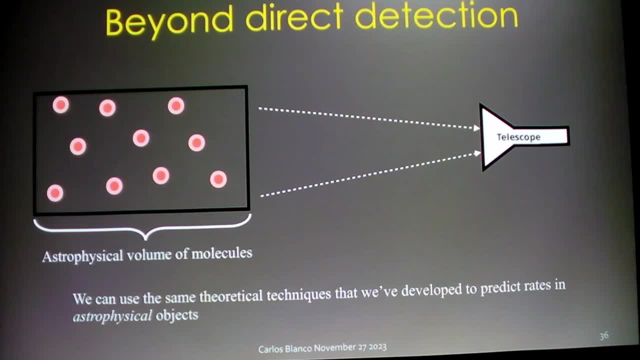 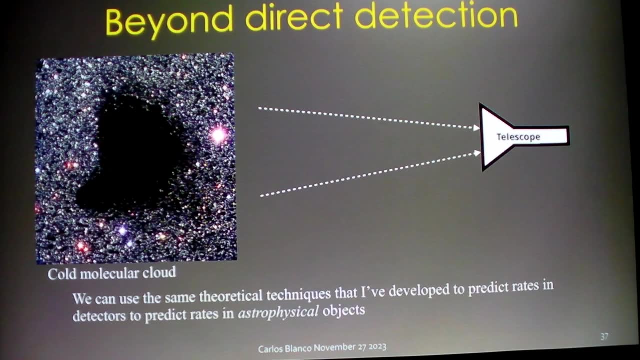 is large astrophysical volumes of molecules and instead of photodetectors you know in, you know biocollide, PMTs, you use telescopes And these things exist. They're called molecular clouds, cold molecular clouds. 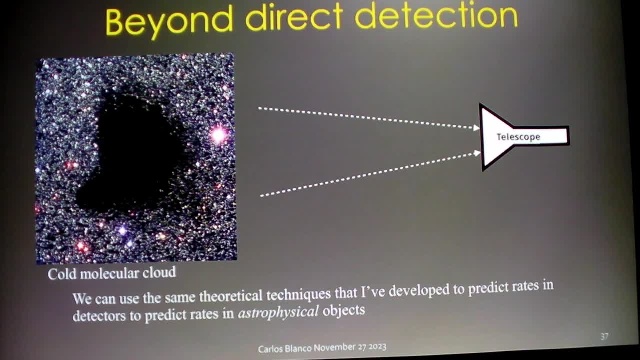 This is an example. This is the Barnard molecular cloud, And it looks like there's something wrong with the telescope. Is the cloud a black thing, or do you see it the wrong way? It is the black thing, Right? So here's what's happening. 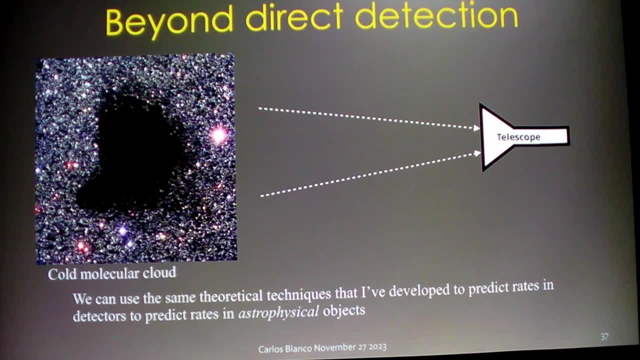 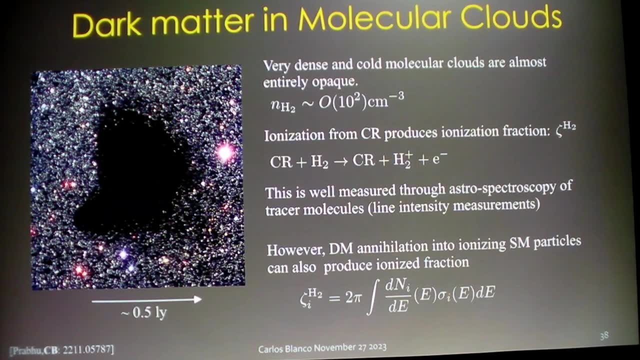 The cloud is composed of hydrogen. It's very dense hydrogen by astrophysical standards, very diffused by Earth standards. It's about, you know, hundreds of atoms per cubic centimeter. But this hydrogen basically absorbs all of the light, above the necessary energy to drive its transitions. 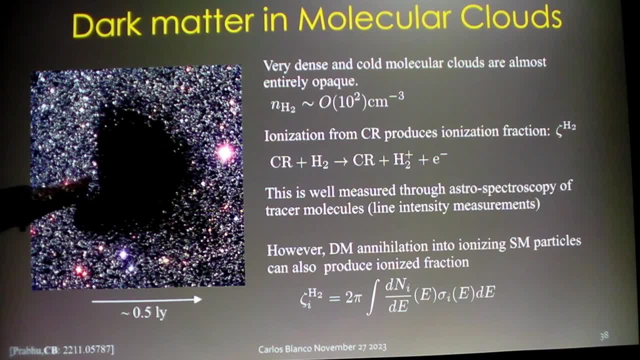 And all of that light is really just absorbed at the surface. You can kind of see the surface skin depth there, And so inside, at the core of these molecular clouds, you have an incredibly clean laboratory where the ionization rate is just governed by cosmic rays. 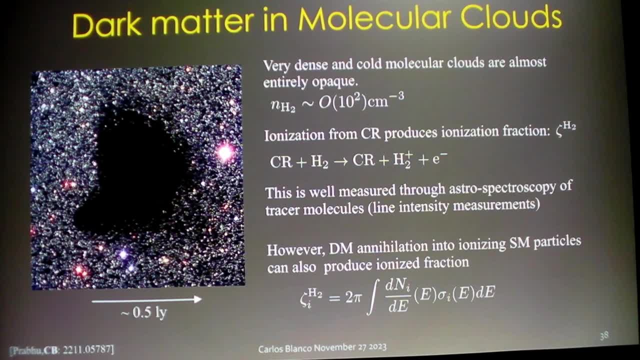 And we know quite a bit about cosmic rays And we know quite a bit about how they ionize hydrogen and how that ionized hydrogen really controls the chemistry of these clouds And therefore the spectroscopy. And so we know very, very precisely. 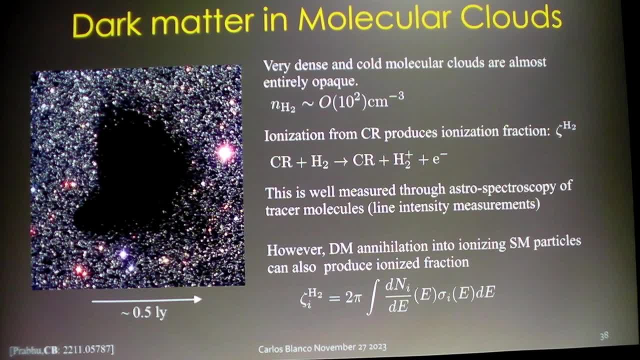 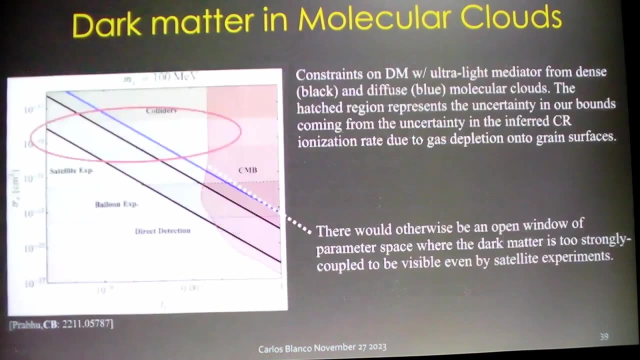 to astrophysical standards what the ionization rate is. If dark matter also interacts with these clouds, it will contribute to the ionization rate in a visible way And we can use that to set constraints on dark matter that interacts very strongly with the standard model. 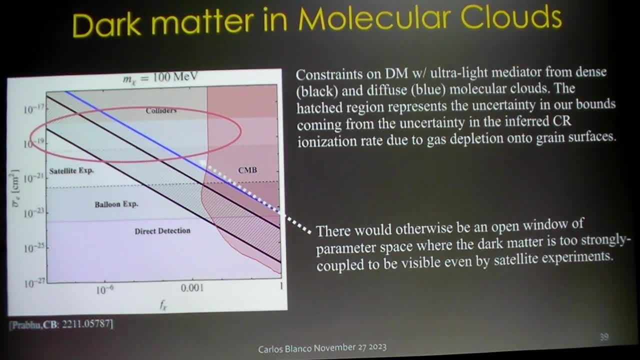 So what do I mean by strongly? Take a look now at the scales that I'm talking about here. So this is like the electron cross, The experiments that I was talking about before, these very sensitive experiments looking for feebly interacting dark matter. 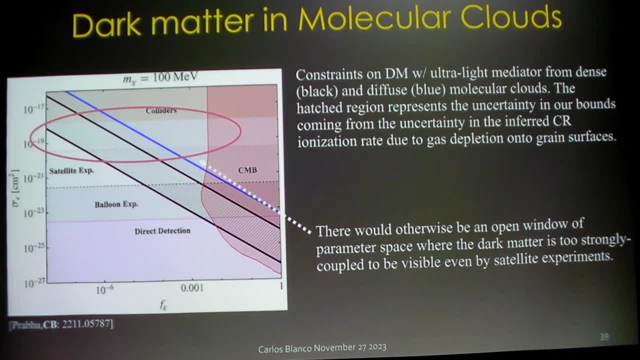 really take place 10 or so magnitude further down here. Now I'm talking about very strongly interacting subcomponents, And in these scenarios what happens is that the dark matter tries to get into your laboratory, but you just can't. You get stopped by the atmosphere. 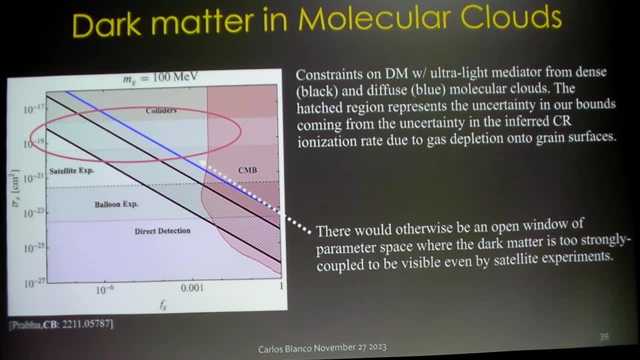 you get stopped by the walls, by the concrete, by your neon paddles, You're totally blind to it, And so the direct detection experiments on Earth have an overburden limit. that's really set here. If you set up a balloon experiment and you send it up to near space, 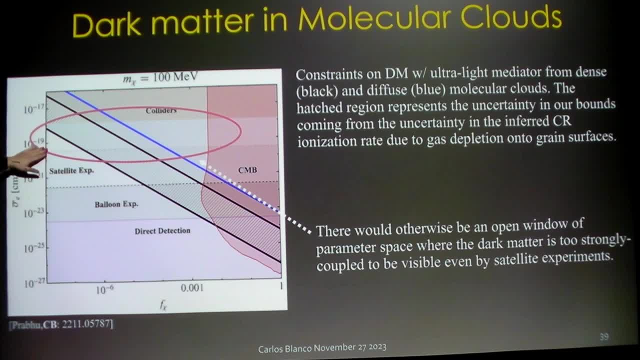 you do a little bit better and satellite experiments do a little bit better. but it turns out that there's still this open window here that is kind of fundamentally unprobable by current experiments, And normally that kind of strongly interacting dark matter would be totally ruled out by CMB considerations. 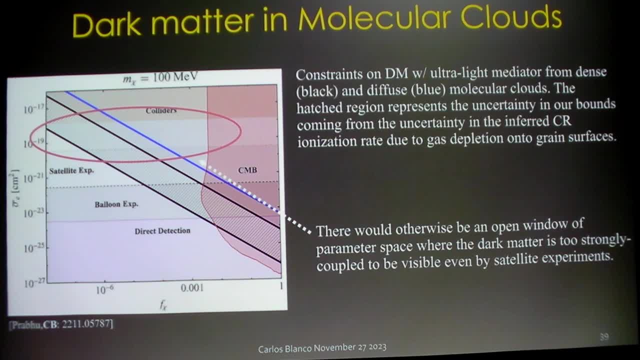 but it turns out that if the strongly interacting component of the dark matter only constitutes a small fraction of it, and models that have strongly coupled components predict that it will only be a small fraction of it, in these scenarios the CMB loses sensitivity entirely. 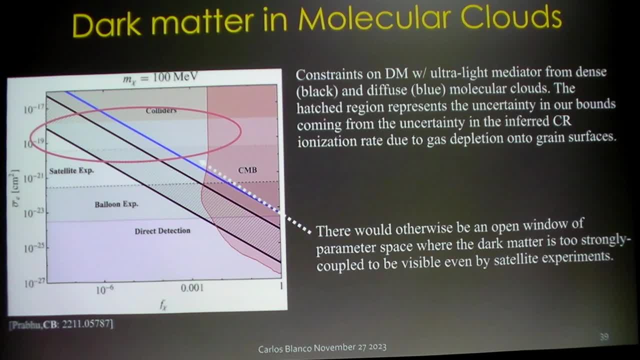 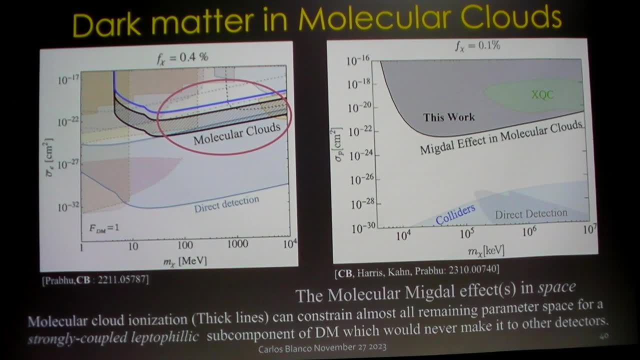 So what do we do? We look at molecular clouds and it turns out molecular clouds are sensitive to exactly this open parameter space. and we can look at things in this way In both orthogonal couplings, the electron coupling and the proton coupling. 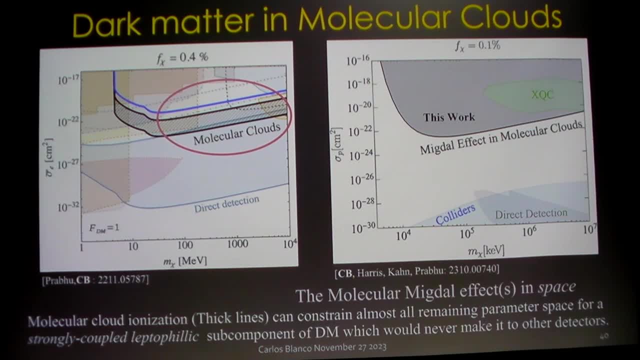 and so in the electron case, which is the first study that we did, the open window is this sort of white space up here and molecular clouds totally rule it out. We were quite happy to basically see an open window write down the basic chemistry. 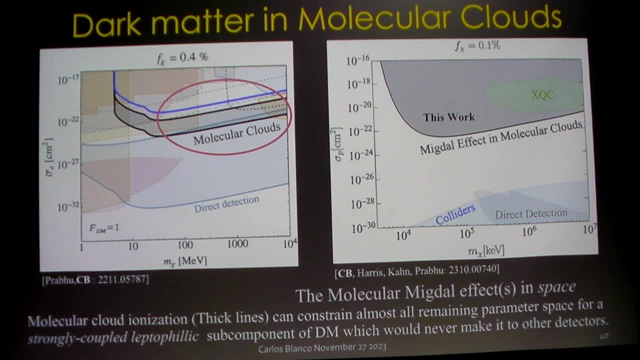 and completely rule it out. and then it became obvious to us, like let's just apply the molecular matrix and the migdol effect and see what the sensitivity is for the nuclear recoil case. and that's what the right-hand side is. 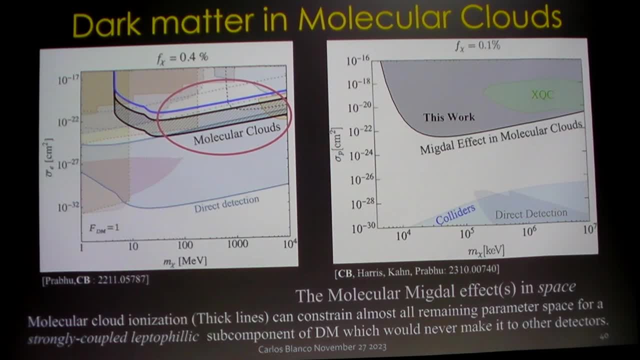 It turns out there it's much harder to constrain dark matter, but overwhelmingly the biggest constraint in these strongly coupled subcomponents is this migdol effect in space paper, And so this is adding to the many reasons why, looking at chromophores, looking at chemistry, 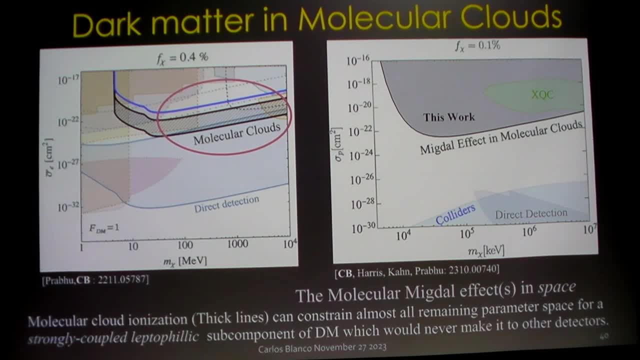 looking at nanomaterials can really benefit HEP departments everywhere. These are all techniques that have existed for a very long time, all technologies that are well understood that we just really need to reach out across the hall and call in our chemist friends. 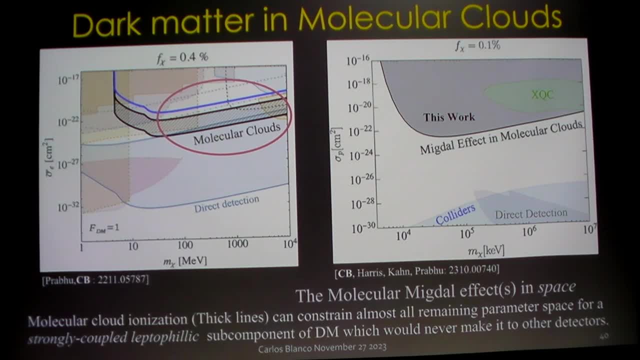 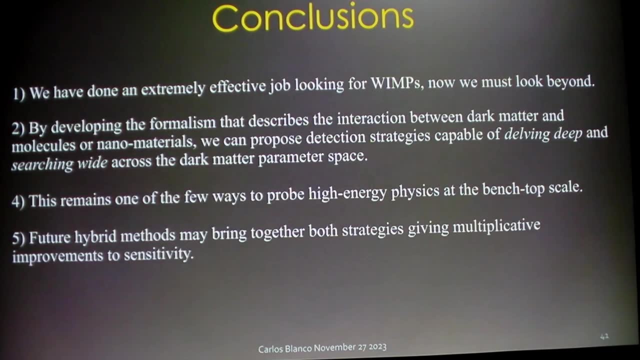 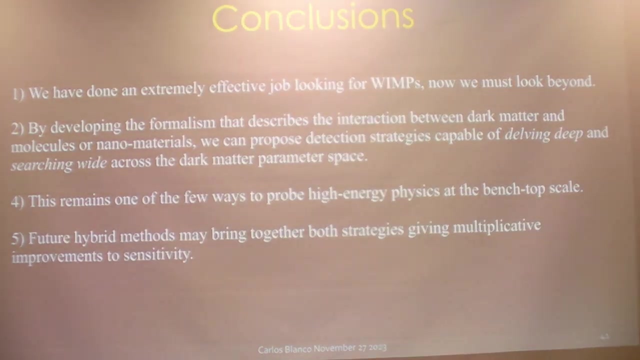 or direct kinetics matter friends and tell them: teach us. Okay, I think that is it. Let me just conclude there. Yeah, take questions. All right, Thank you. So how pure does a sample need to be? Like experimentally, there's always impurity. 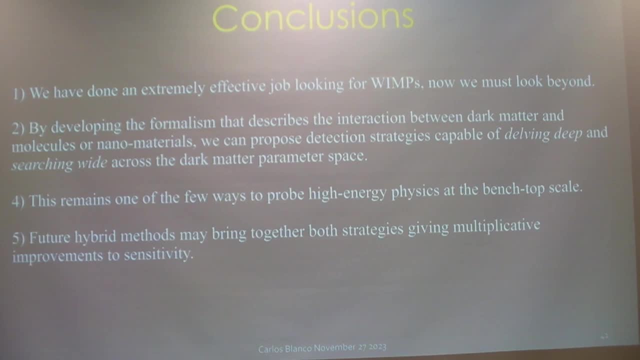 even though you're synthesizing some molecules, right? Is that a big problem? Yeah, so in the chemistry lab, if I have a dirty sample and I want to clean it up, one of the best ways to do that is to crystallize it. 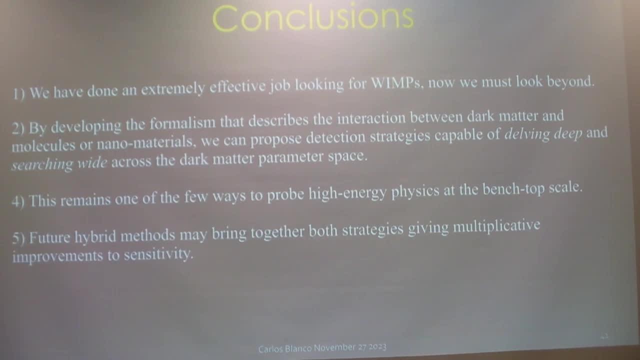 We're working with crystals. If you form good crystals, they are inherently extremely pure. because impurities lead to bad crystals, The crystal formation does not propagate, And so the problem of purity when it comes to molecular crystal really boils down to the problem of large-scale crystallization techniques. 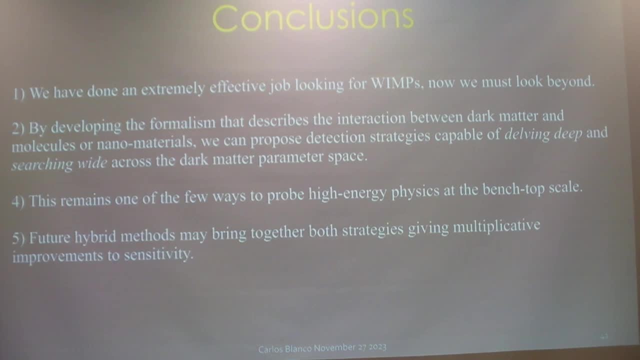 And that has been really perfected for many years. That picture of a crystal that I showed you is a single crystal, But it doesn't matter if it's a very good crystal. Seriously Well, you can work with What if that can contribute to your signal. 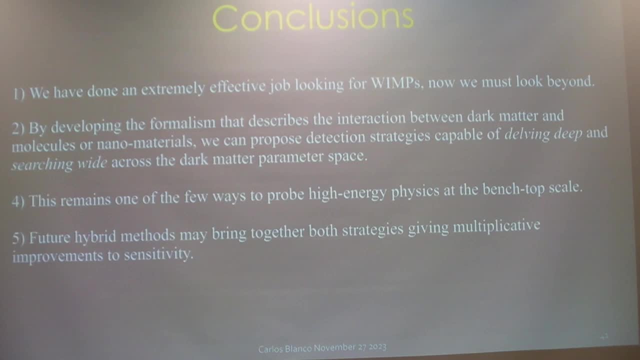 if you don't, You don't care. right, You might care. So what we're learning is that very sensitive experiments do care about microfractures in crystals, because these small atomic shifts lead to phononic excitations and energy depositions as these crystalline phases 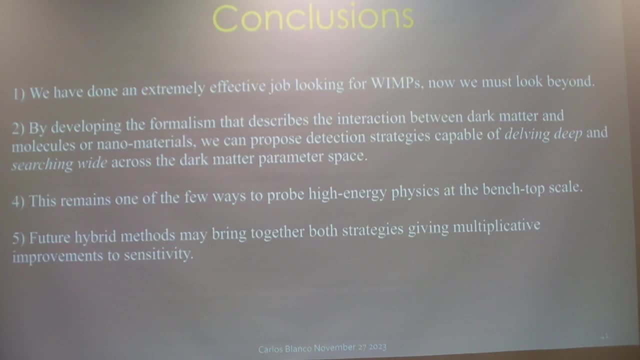 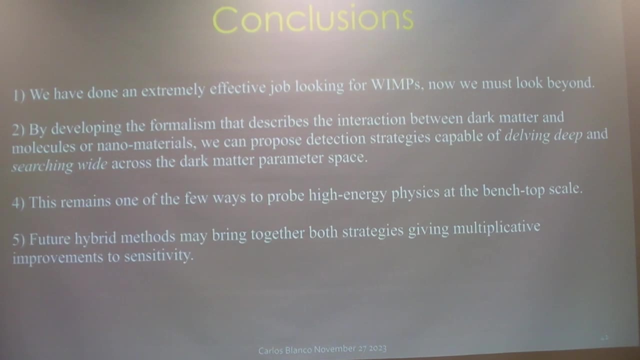 rub against one another. They look like energy depositions, And so if you're looking for small energy depositions, these fracture points can lead to bad ones, And so you might still be able to work with things that have fractures and that have defects. 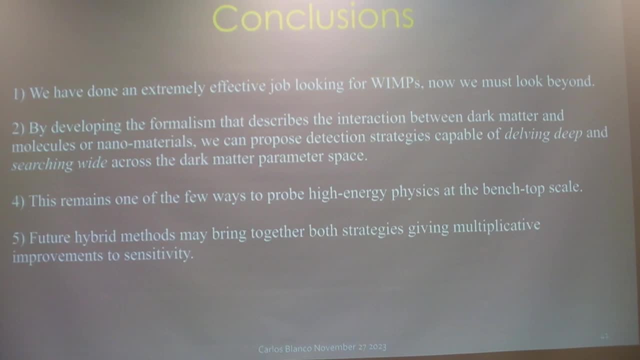 It's always better to reduce them. How do you physically introduce signal? Are these cracks and defects? I don't see it, because unless you cool the whole thing down, nothing comes to the crystal. What contributes to? Why did it produce 5 eV photons? 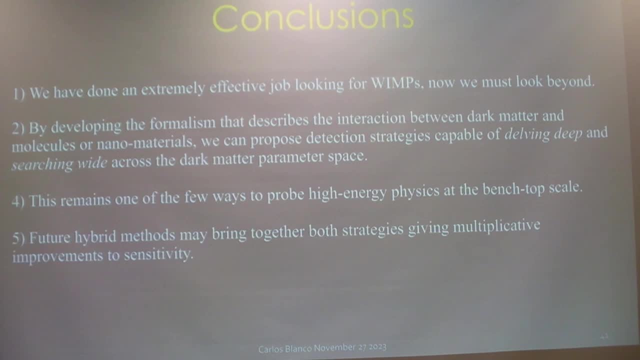 There's no chance it produced 5 eV photons, right Yeah, so the experiments that see the backgrounds from these things are not looking for 5 eV photons. They're looking for, like milli eV excitations. So you're right that the signal is different. 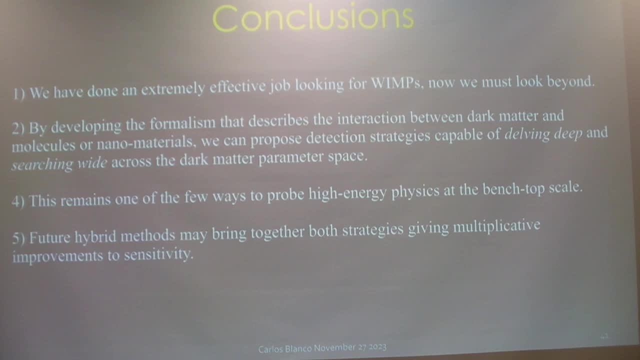 But the point remains that, say, I have a single atomic dislocation, right. What I have is a color center which is another kind of chromophore, right, That's going to change my emission characteristics? The fact remains that you always want to work. 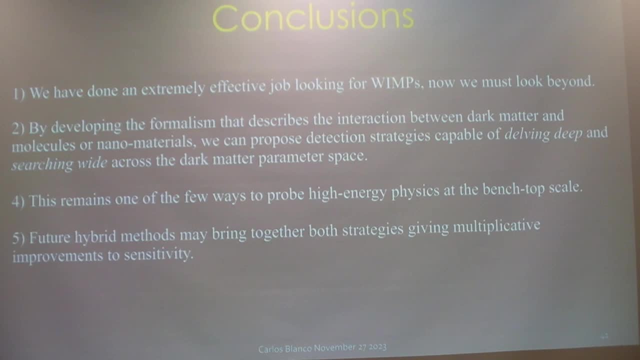 with the purest possible crystal. If you introduce color centers, if you introduce dislocations, you need to be able to characterize those backgrounds. So if the only source of excitation is a dark matter, you are happy. if they actually produce more signal, right? That's why you do these weird synthesis of all these weird molecules right. You want to find a molecule in a weird composition structure to give you high efficiency. When the electron, you know when they take place, they make it the hardest. 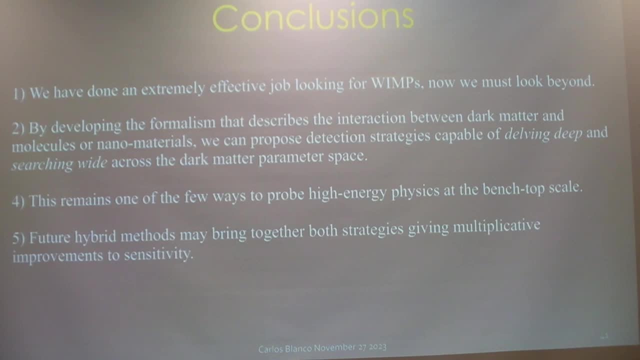 The thing is, is that the expected result is that you're not going to find any signal right, And then to interpret that result you have to know what your sensitivity is. So is that correct? It's a question of you know. 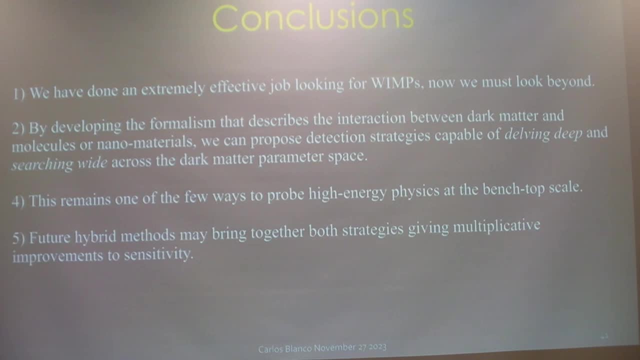 in order to know what your result means, you need to be able to theoretically characterize it. That's the answer to the response. So if you had your cracks and you were able to completely theoretically characterize it, you'd be right. Is that correct? 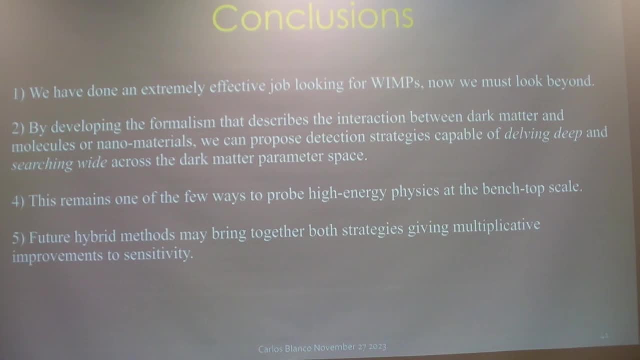 Yeah, yeah. So calibration is hugely important And if you just look experimentally at you know you generate 10 crystals and you do spectroscopy on the 10 crystals, the spectroscopic analysis will be slightly different on the 10 crystals, right. 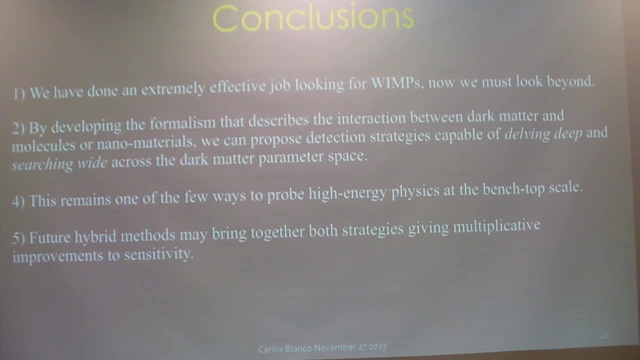 The quantum efficiency is going to be different, The emission characteristics are going to be different. right, And that all comes from fundamental impurities and cracks inside of the tube. A crack is not only a place that you can have dislocation, but it's also a reflection surface. 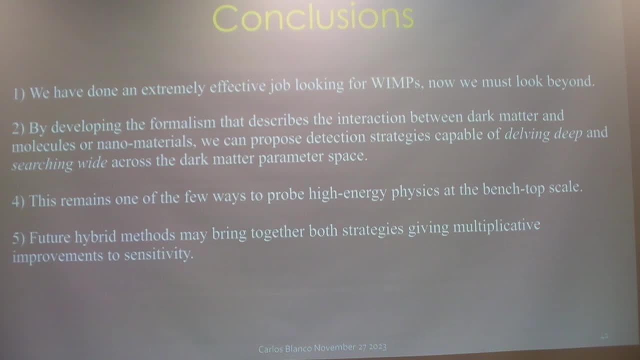 which means that you can trap photons inside of it. Their free streaming is going to change, But they have to be very, very dirty, crappy crystal to give you that kind of effect. right? You're really looking for extremely weak events, So weak. 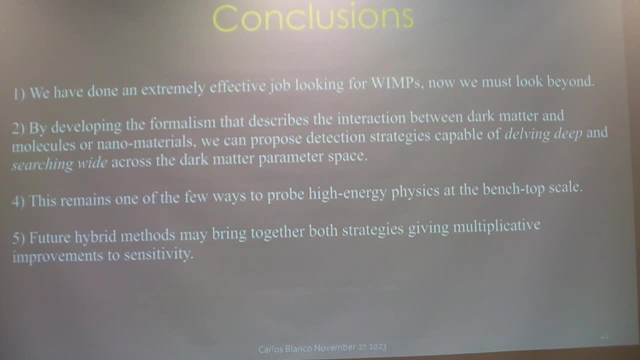 These. they've got to be very piece of extremely dirty crystal. Then I don't think I'm understanding your point. Are you saying that the difference between no cracks and a few cracks isn't the difference? I would expect very little effect, because if 99.99% of the material is video crystal, 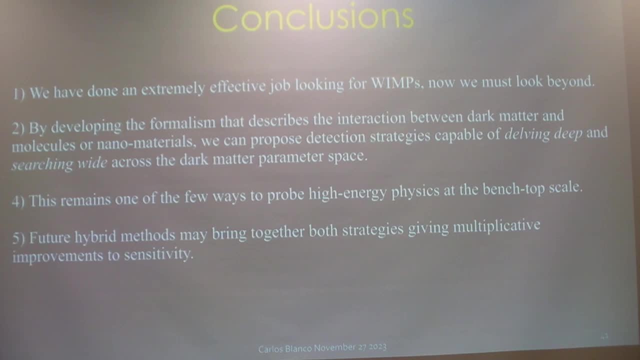 the rest is just a defect. whether it's in sheet form, line form or point form, They produce. no, You are looking at extremely weak events, Extremely weak events. So I think we're talking about different kinds of crystal dirtiness, right. 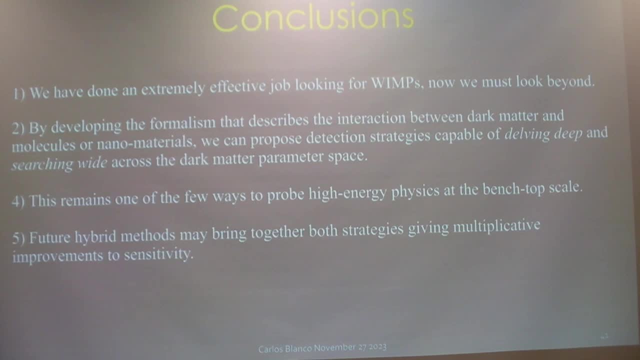 I'm talking about the difference between something like the kind of quartz you find in rocks that is essentially opaque, that looks white, versus a totally translucent optical quality crystal. The white is terrible, of course, But this is possible with molecules that They change the optical. 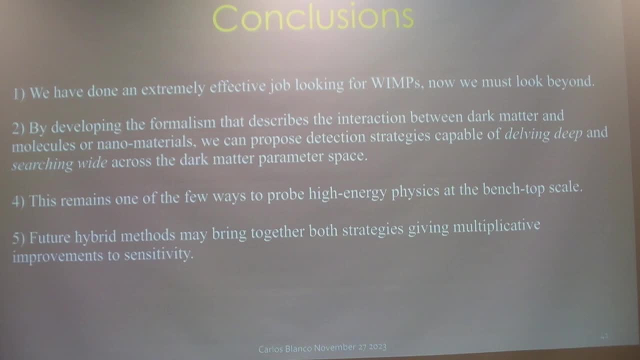 they change how light they come out of the crystal. I'm saying that it's pretty easy to get things clean enough. I'm not sure if you guys are really even disagreeing. I'm not sure we are. It's very easy to make a reasonably transparent crystal. 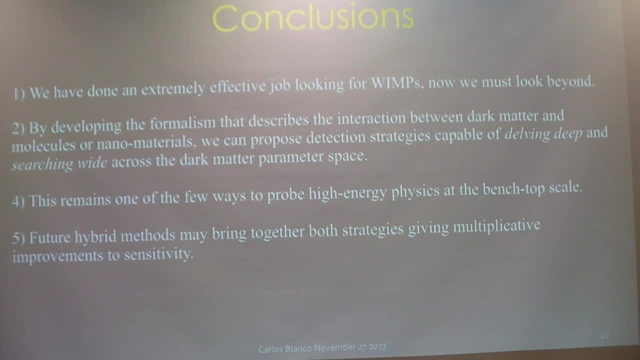 Yeah, I agree, That's what I mean. Yeah, I think you guys are saying the same thing. I mean, I don't think You don't need it to be perfect, but you need it to be Quite good. Yeah, I can't tell, but 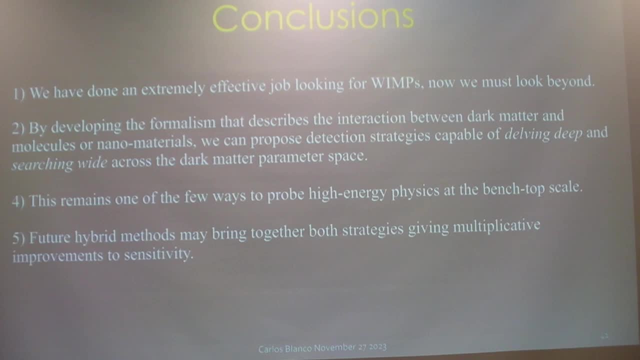 Yeah, no, I don't think we're disagreeing on this point. And for a similar thing, when it comes to a medical effect, the isotopes will do something right If you have different isotopes, even though the crystal is perfect. Yeah, Are you worried about like radioactive decay? No, just like, if I have different isotopes, the mass of the nucleus is different and the response will be different, and it's not a big problem. Yeah, isotopic effects are really quite small. 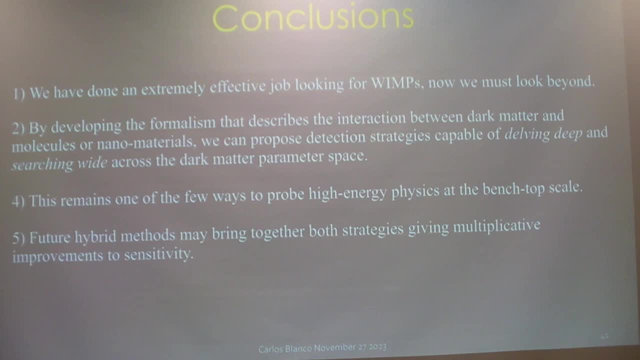 especially if you're looking at carbon. So if you're looking at just hydrocarbons, which are the kinds of things that we're looking at, the isotope contamination can be quite low, especially if you start with petrochemicals that come from deep underground wells to begin with. 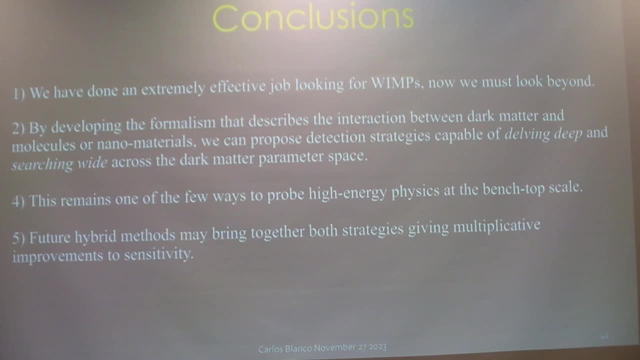 That's very low radio background and that's essentially all the same isotope. So you can really limit that. Now. if you were worried about the radio background, because that does deposit a good amount of energy there, I think you may have a little bit of a point. 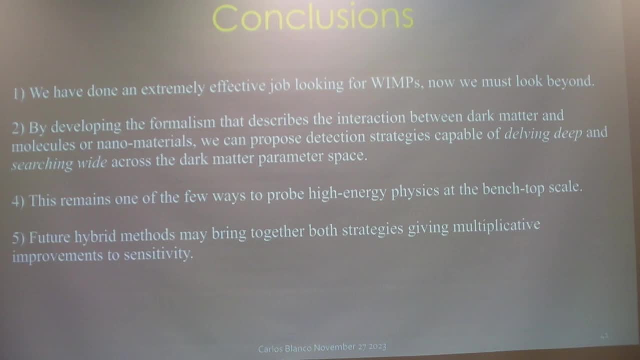 but there is a clever way to get rid of that, because you basically say: any time that your detector lights up with a decay, you just ignore that. You're not looking for your detector to light up, You're looking for single photon events. 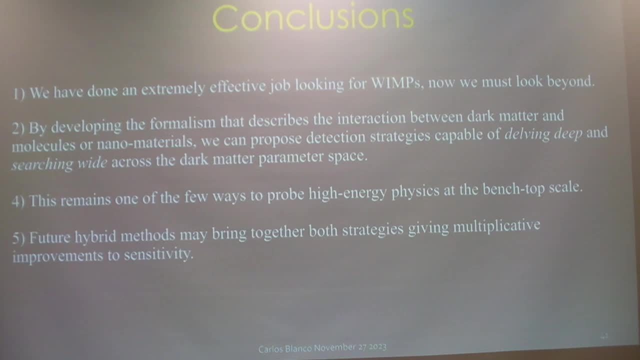 or coincident photon events, And so you can get rid of decays that way. This is a much more general dark matter question, but do you have reasons to believe that there are lower bounds in electron interaction cross-sections we were looking at? 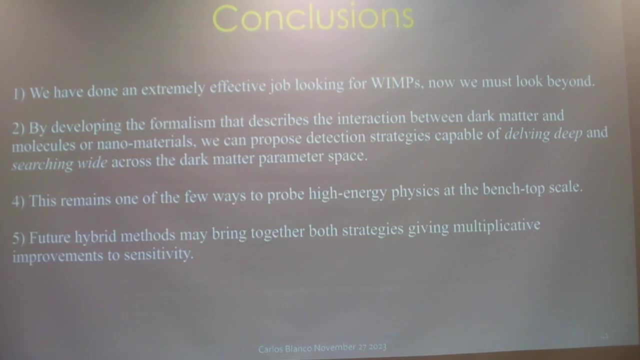 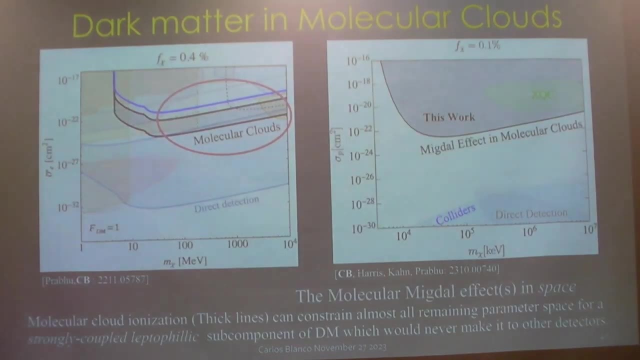 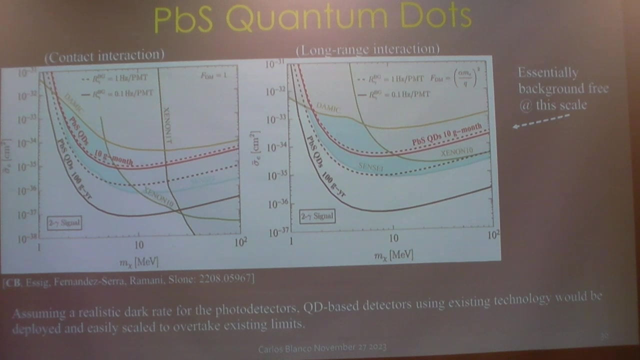 Lower bounds. You had some lines in there about freeze-in or freeze-out. Those are things I've heard in the seminar once but cannot remember anything about. Could the cross-section just be zero? Could it just be zero? Yeah, You can live in a nightmare scenario. 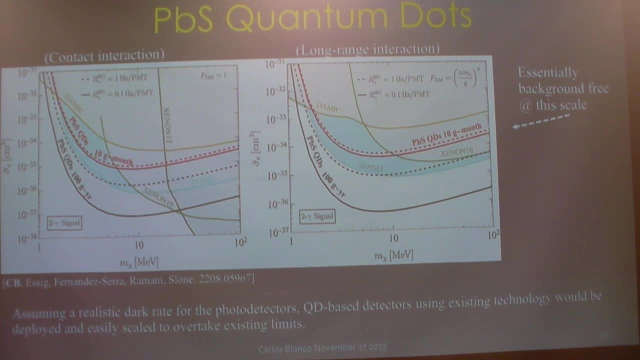 where you're only coupling to the standard model view of gravitational interactions and then you're totally asleep. But let me ask you: what predictive dark matter models can you really write down that are consistent with early universe cosmology, that are consistent with structure formation? 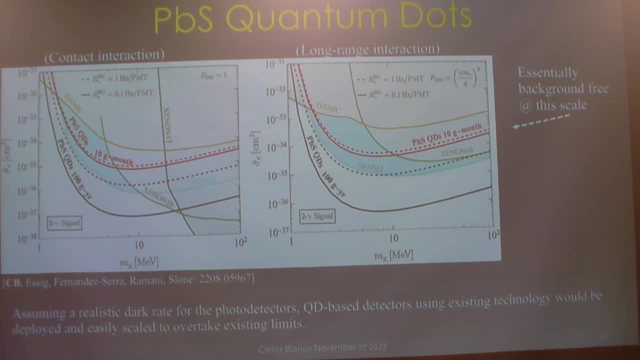 Most of them have at least equal couplings to the standard model, Got it? And all of the good dark matter candidates that we have generally predict have some prediction of what the cross-section ought to be. So from cosmology simulations, does that suggest we need a coupling, at least this week? It depends on what dark matter model you're talking about. Very generally, I would just say that if you just had gravitational interactions, there's no way to understand how you get the relic abundance in the first place. So in other words, the fact that there's a relic abundance. 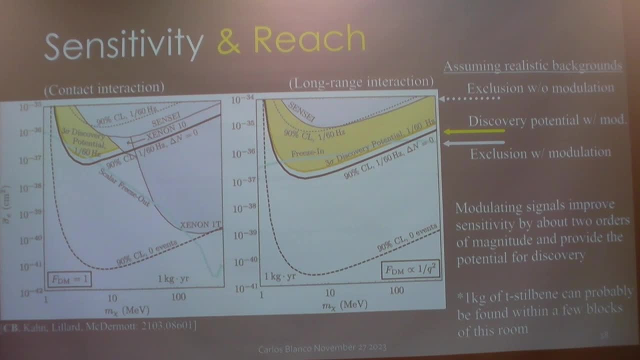 somehow suggests that there's. I don't want to hand-grey the argument, but that there's some additional interaction that's non-gravitational, that's responsible for its presence in the universe, its relic abundance. Now, there's not a way to make a direct line between that. 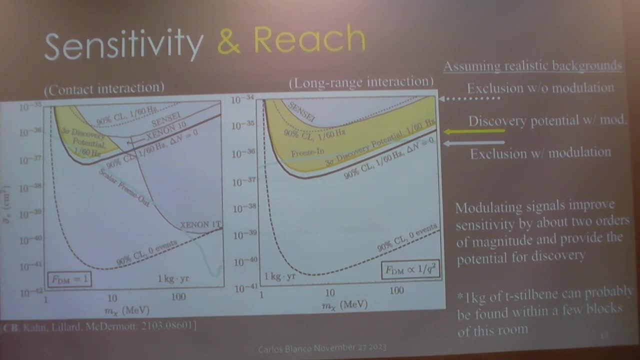 unless, as Carlos says, there's a lot of models that you can see very frequently. you do have some sort of signal that So if dark matter got made with the Big Bang, it has to couple somehow from whatever that creature was. Yeah, if you just had something.